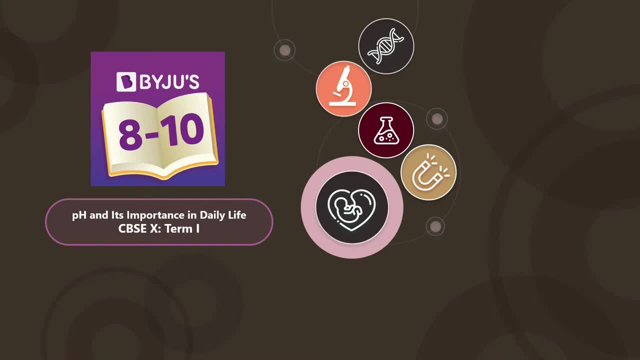 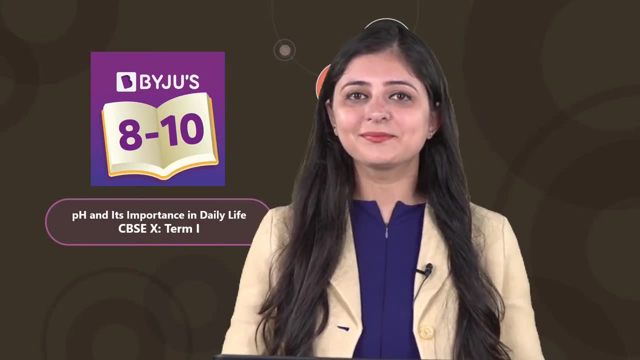 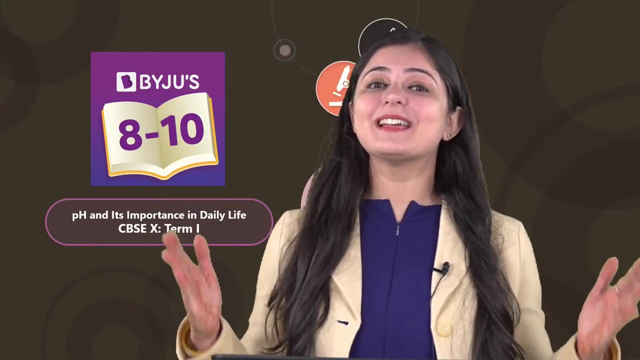 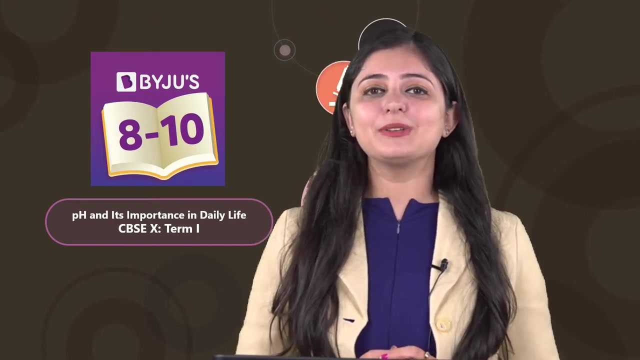 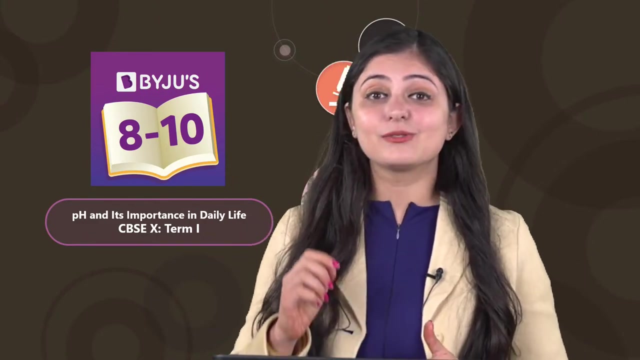 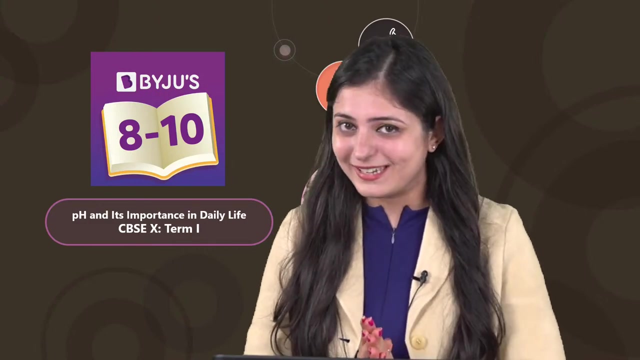 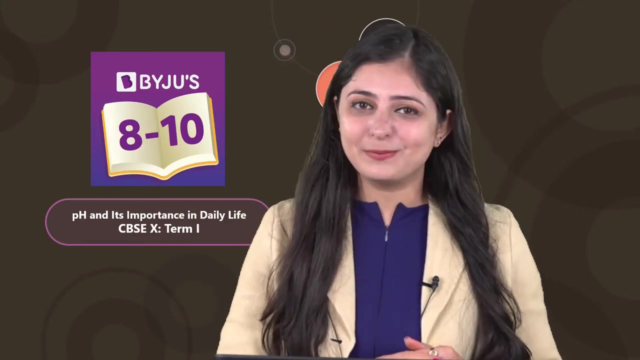 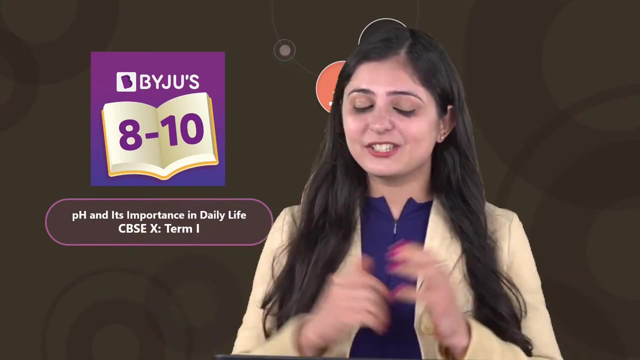 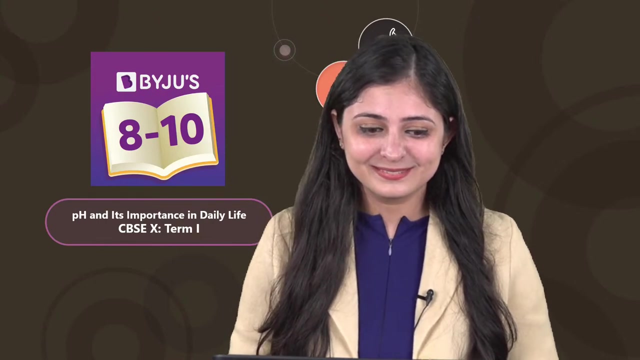 Hey everyone, a very good evening to one and all. My name is Kriti and I am back to help you prepare for your upcoming board exams. But before we start this session, you know what you have to do. Quickly let me know if I am perfectly audible and visible to everyone out there. But today, let's not post a thumbs up, let's not put a take or write yes in the comment section. Let's do something different. Let's write happy Diwali with a smiling face. So when I see your comment of happy Diwali with a smiling face, I'll get to know that this setup is working fine for you people. Well, tomorrow is Diwali. So let's have a very happy Diwali and let's have a very happy session today. Let's wish each other and start this session on a very, very positive note. Kashi says happy Diwali. Happy Diwali, Kashi. 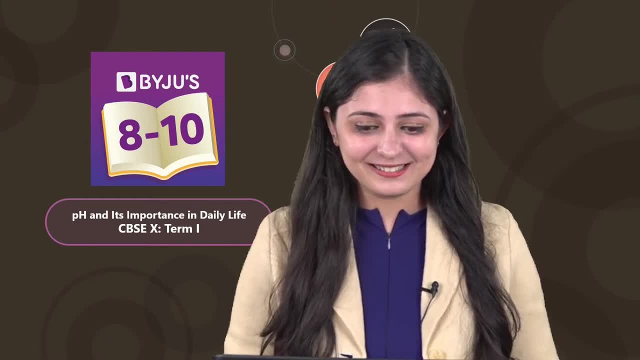 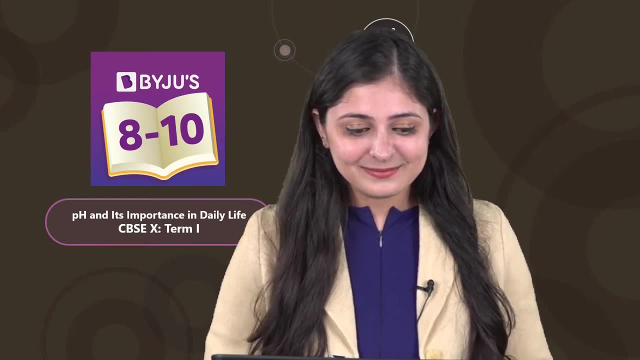 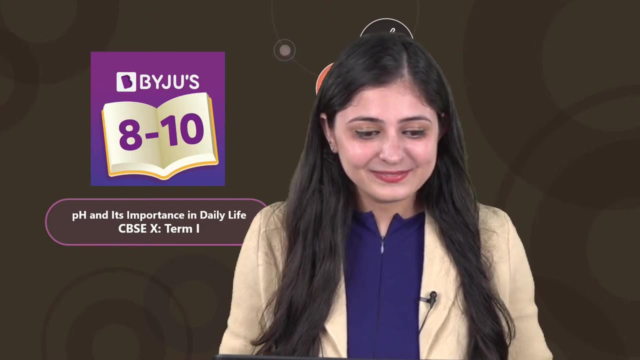 Happy Diwali, Adi. Happy Diwali, Rishita. Happy Diwali, Nikesh. Happy Diwali to you, Priya Shah. Hi, Swaroop. Happy Diwali. Hi, Priyanshu. Happy Diwali to you also. 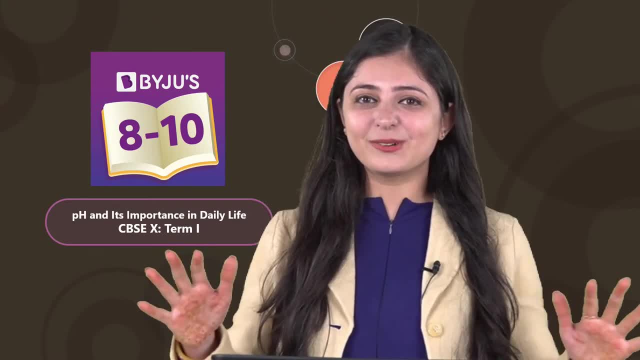 Great, great. Now this chat box is looking very interesting. 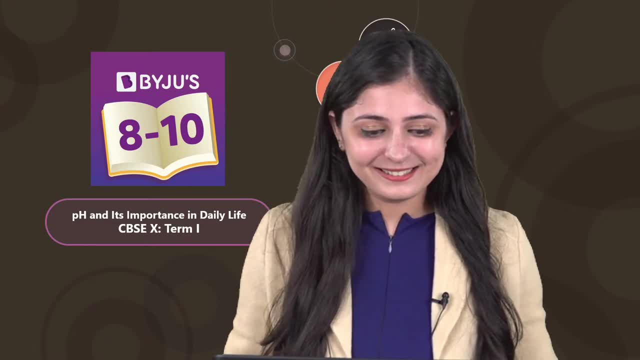 Hi, Jai. Happy Diwali. Hi, Darpan. Hi, Aradhana. Happy Diwali to you. 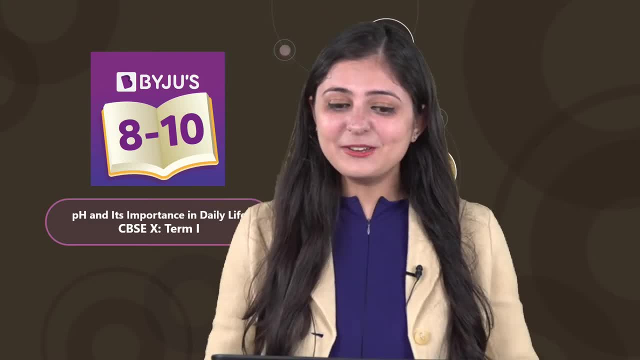 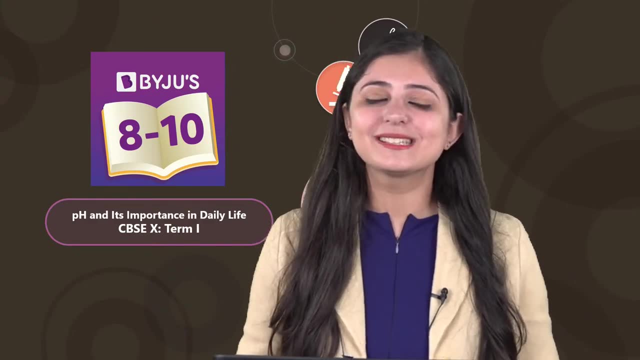 Hi, Pравствуйте. Happy Diwali. All right, you people have brighten up this chat box and on this positive note, I welcome all of you to Baiju's class 8, 9 and 10. 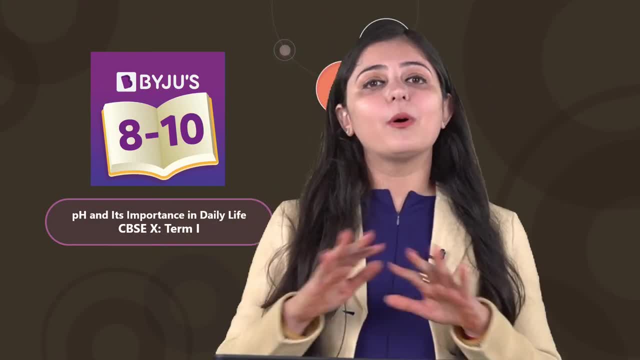 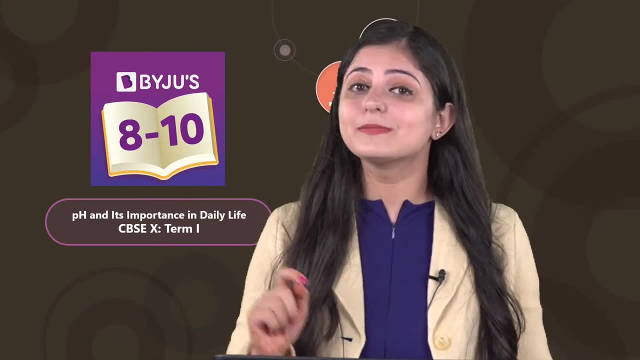 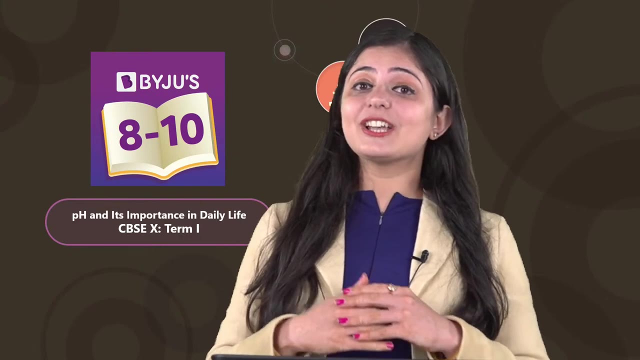 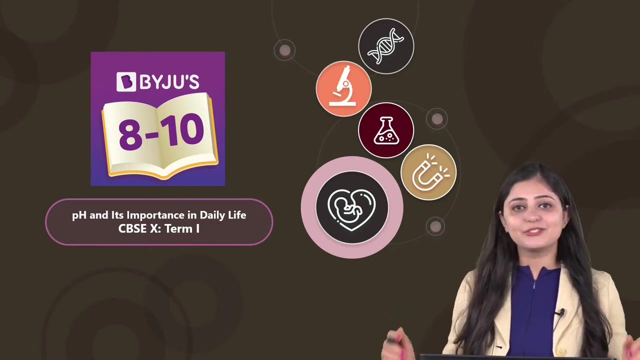 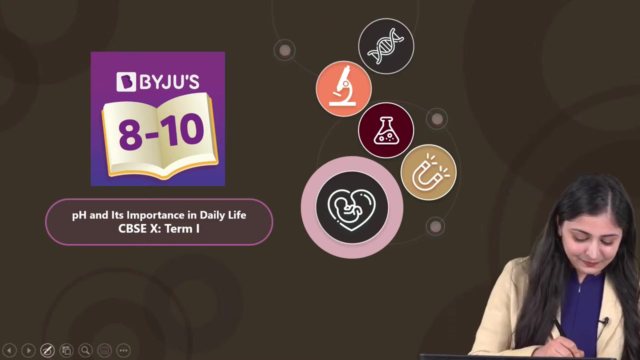 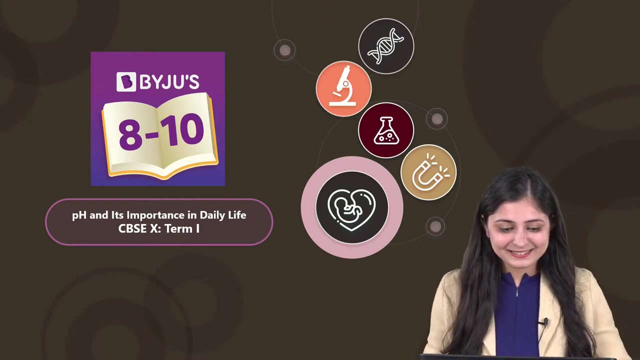 this is the MCQ crusher series that we people are having I hope all of you have subscribed to our channel another Nikiya Koi Barney do it right away and hit the bell icon so that you do not miss any notification from our end now the topic that we have today is pH and its importance in daily life how many of you find this topic interesting I personally think that this is a very very interesting topic how many of you find it interesting tell me good evening Priyanka Yes its PH and its importance Abhijeet sees he finds it interesting yes yes Abhijeet says yes yeah I think it's 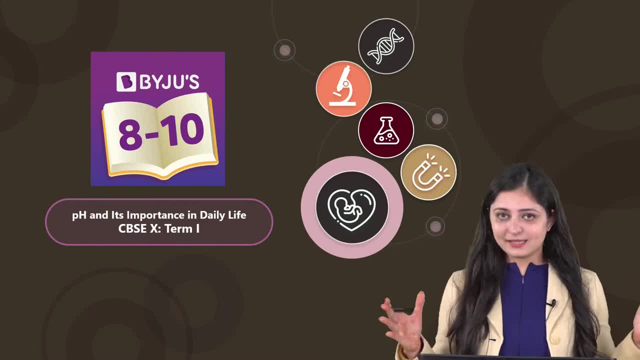 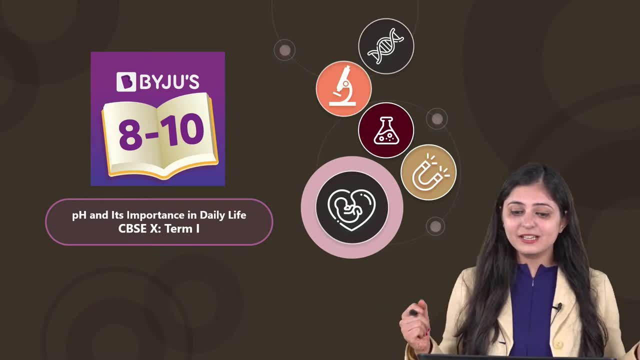 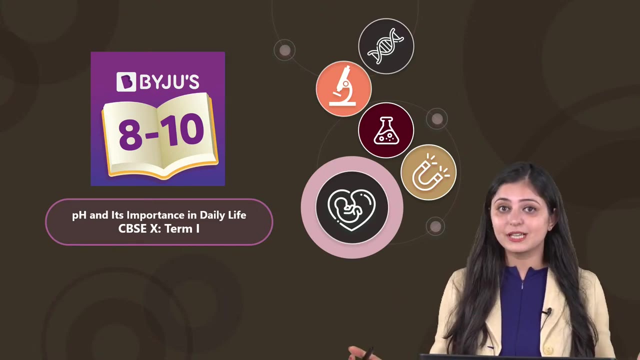 a very very interesting topic in fact I feel that chemistry is a subject science is a subject wherein whatever we study in the class we can easily observe that in real life isn't it whatever we are studying in we are following whatever is the problem problems we face in class, more or less they are the real life problems or real life situations 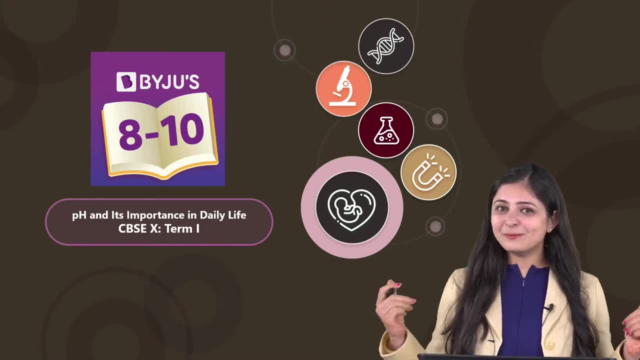 that we face on a daily basis. So I think that's really cool about this subject. Satyam says please provide classes for class 9th. Alright Satyam, we will definitely be starting 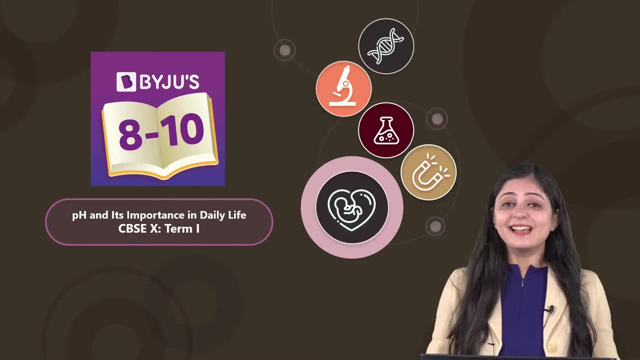 with this really really soon. In fact I feel that your home or your environment, it's like a laboratory of its own, isn't it? Hum jo bhi kar raha hai, hum jo bhi kar raha hai, somewhere or the other there are the chemical reactions. All you need is an inquisitive mind. Thoda sa inquisitive mind hona chahiye, thoda sa willingness hona chahiye and you will see all chemical reactions happening around you. Good evening Suryamani. Shatakshi 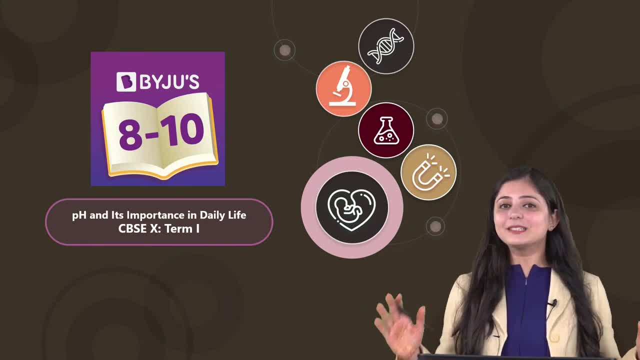 says yes ma'am. So Shatakshi bilkul agree kar raha hai, bohot hi interesting topic hai. 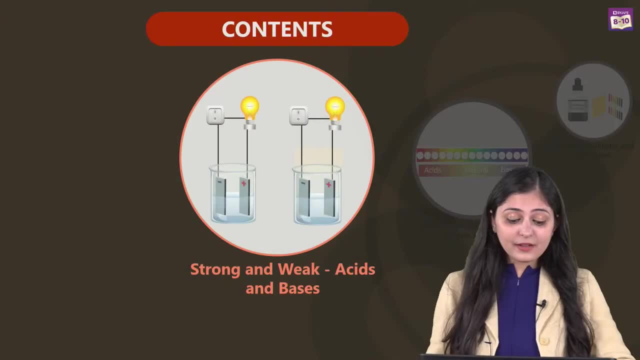 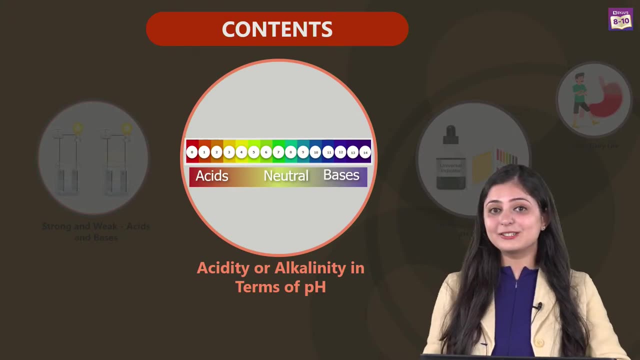 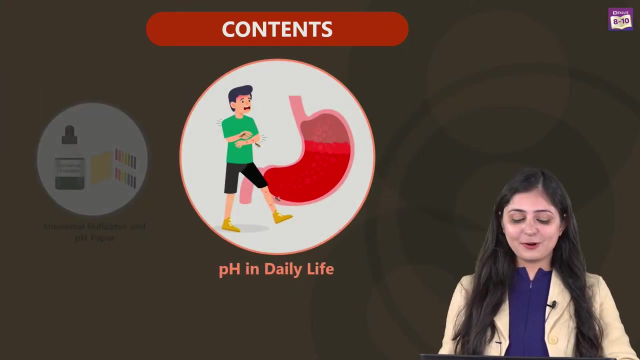 And let's see what contents do we have for today. We have strong and weak acids and bases. Then we've got acidity or alkalinity in terms of pH. Then we've got the universal indicator and pH paper. And finally we've got pH in daily life. So these are the sub topics that we have for today. I hope all of you have revised these sub topics. 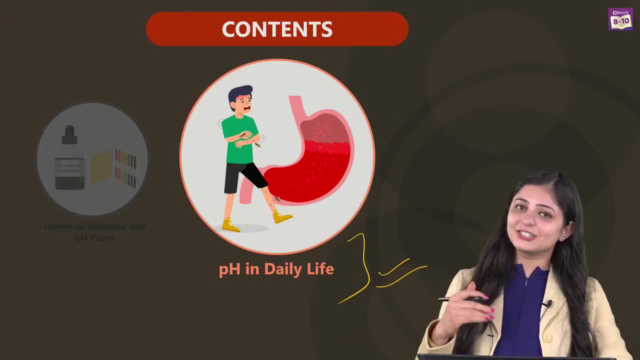 Kyunki jitne acche se aap revision kar ke aage, utna accha hi aamara yaaka practice session hoga. So if you've revised, write a yes in the comment section. So if you've revised, write a yes in the comment section. So if you've revised, write a yes in the comment section. Tell me. 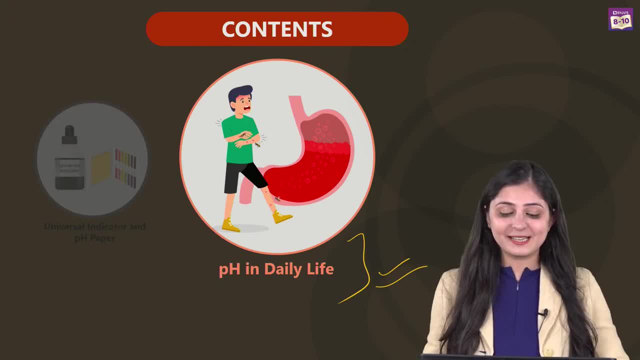 Devansh is saying please start quickly, I'm very excited. Happy Diwali Rituja. Manoj says yes ma'am. Alright. So you people have revised, very good. That means I'm going to get all correct answers. I can expect that, right? Yes ma'am, definitely. Sambhavi says yes ma'am. Satam says yes. So let's do one thing guys. Today let's go in a very organized manner. So let's start in a very organized manner. Instead of randomly posting answers, what we can do is we can write the question number followed by our answer. Say suppose you want to answer that question 3 has C as the correct option. Just randomly I'm saying. So what we can do is we can write 3 dash C. So this way, I will easily get to know, I can easily analyze whether you're answering for the current question or is it the previous one that you're answering. 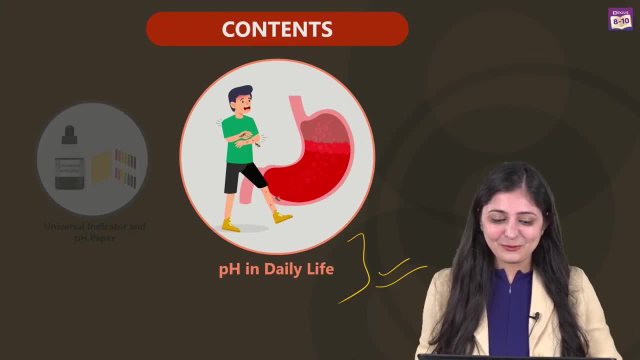 So can we do this way? Quickly, let me know. I think it's a better way. Okay. 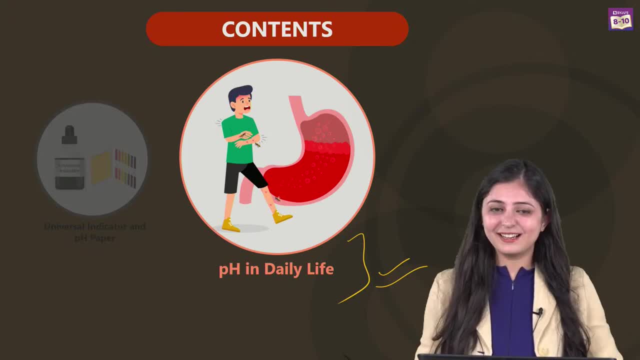 Hi Sachin, it's okay. We are just starting. No issues. Alright. Ayush says hi. Parul says yes ma'am. Alright. So you people are ready to do it this way. Great, great, great. Piyush 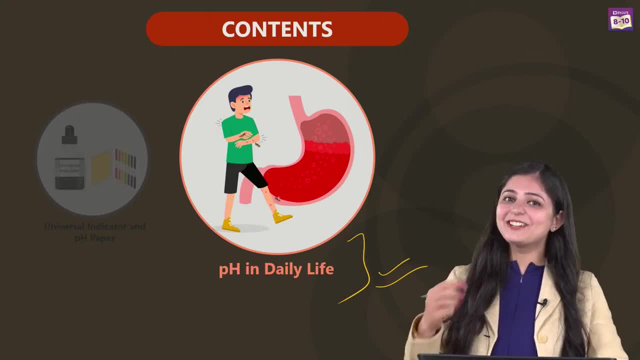 says yes. Alright. Then let's get started and try and solve the first question together. 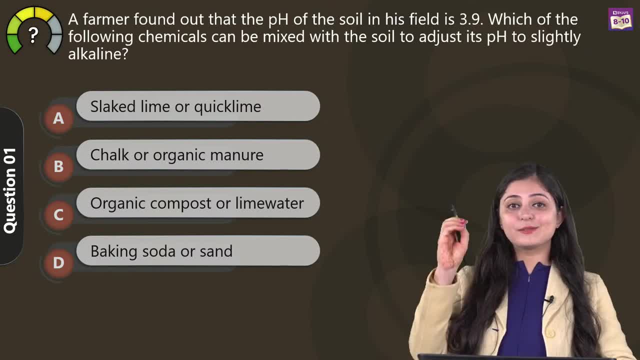 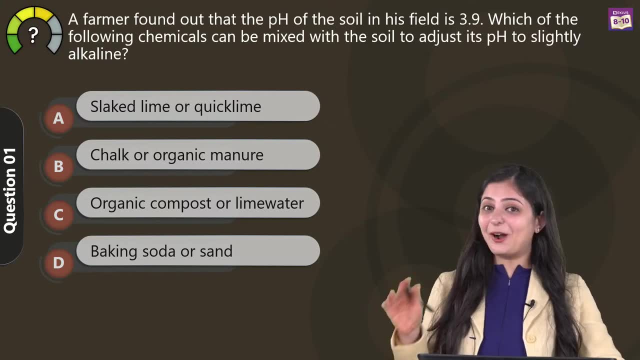 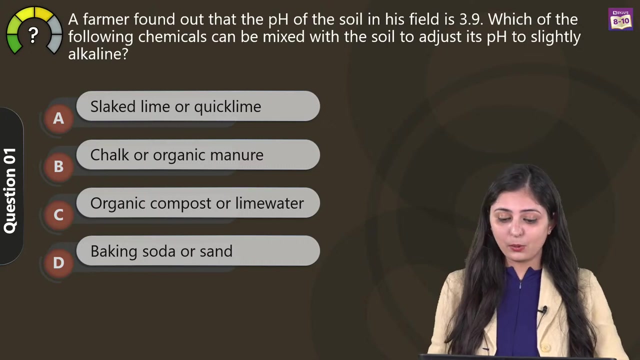 You know what you have to do. If you know the answer, start posting the answer as one, dash, and whatever is your answer. I hope I'm gonna get one unanimous answer over here. Let's see. Let's see how much you've revised and come. Bol toh diya tum logon aayin ki humne bahut achche se revise kara hai. Sabne yes lekha hua hai. But let's see, is it actually true. Now, question number one says, a farmer found out that the pH of the soil in his field is 3.9. Which of the following chemicals can be mixed with the soil to adjust its pH to slightly alkaline? Now, we know that plants grow in a sub-soil. So, it's a good idea to add a little more plants grow in a certain pH they need a pH range to grow in a healthy 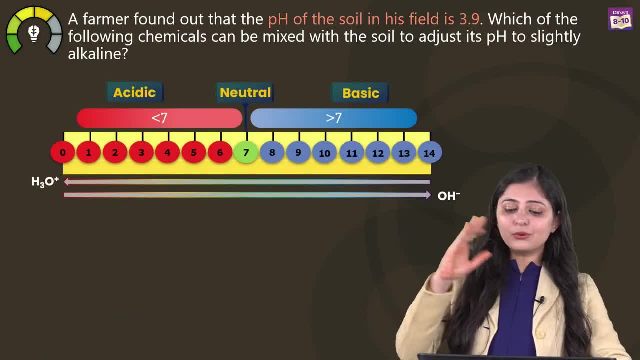 environment now in general 0 to 14 is the pH range that we have if it is 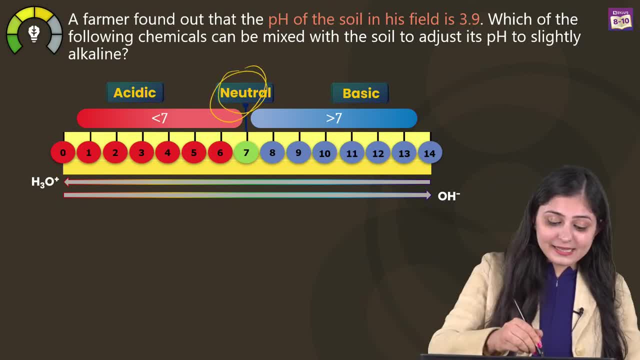 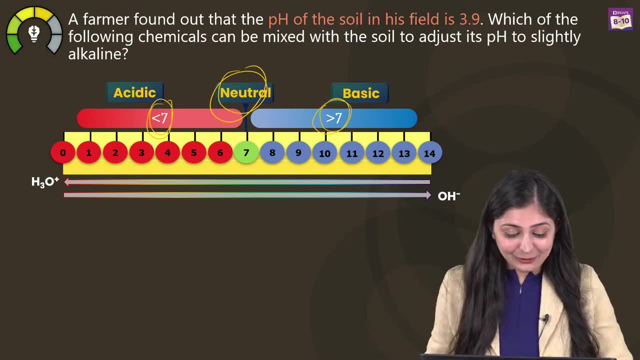 neutral it's going to be 7 if it's acidic it's going to be less than 7 if it's basic it's going to be more than 7 but easier you have a sub copata now the 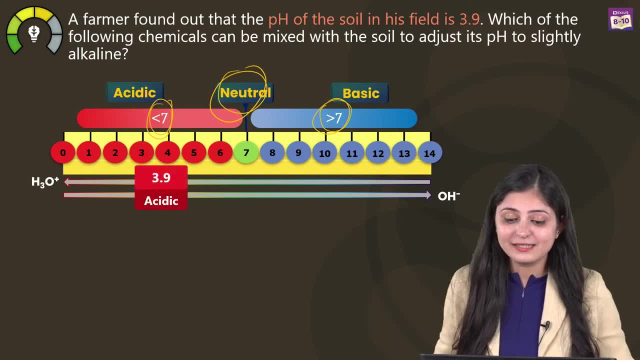 pH they've given is 3.9 and with this I see a lot of answers deepak says a or B deepak a or b what is this answer choose one and let 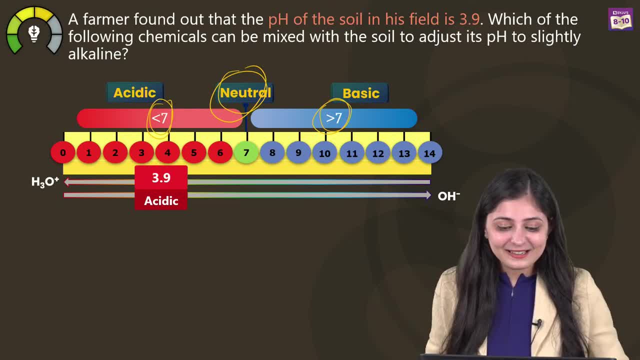 me know iron says a life of country says a Alyssa says B hurry Priya says a Jay Academy says C all right 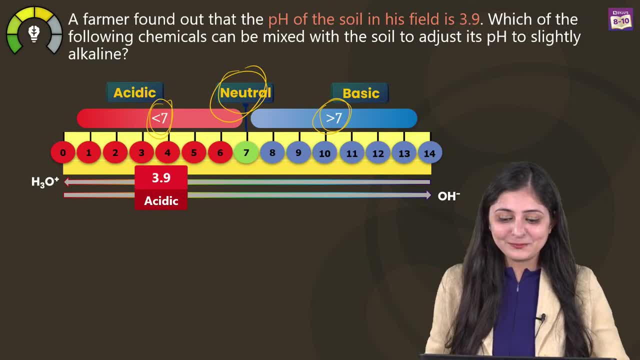 sub kut boldiyo a b c d sorry options ball them but I think mostly people are saying a Sutton says D pulleys is a sakina sees a je t'aime 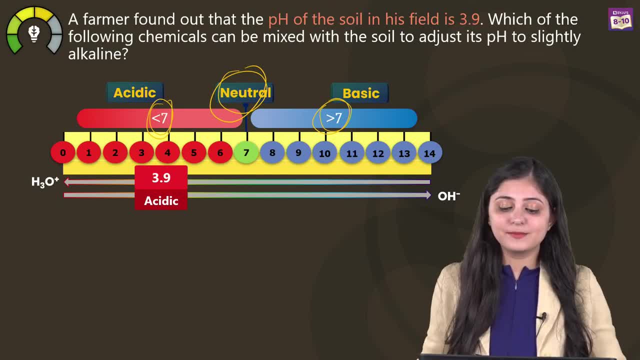 says a Abhi Gyan says even my name starts from a all right so I think majorly a is coming shatak she says a so I can see a lot of a is coming my way 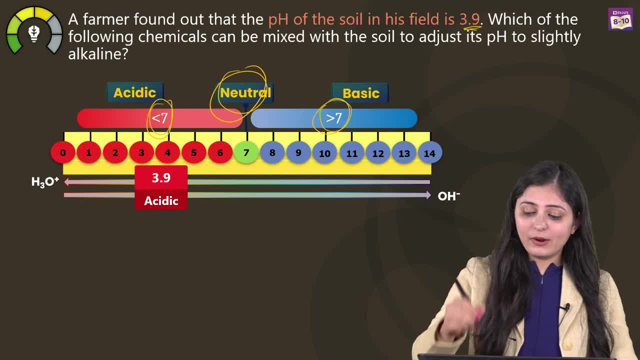 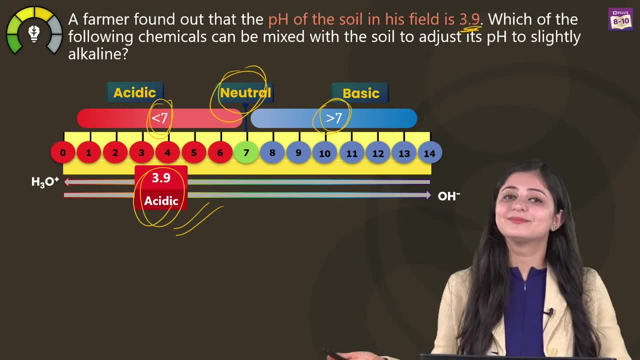 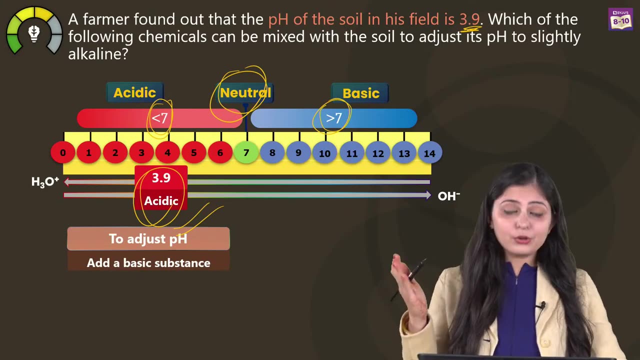 let's see now 3.9 that's the pH that they have given us in this question 3.9 less than 7 the soil is definitely acidic now acidic soil not so favorable to grow crop site what do we want we want to adjust the pH to adjust the pH 7th class apart they are a neutralization can I we need to add a 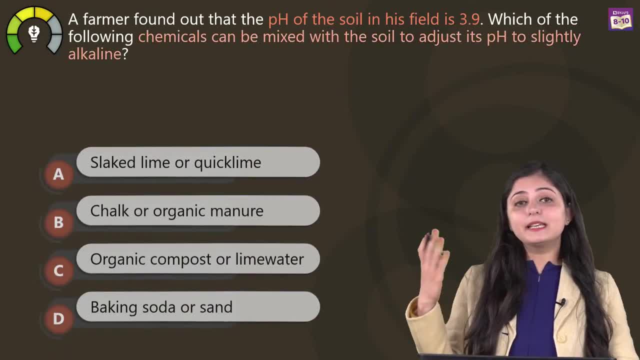 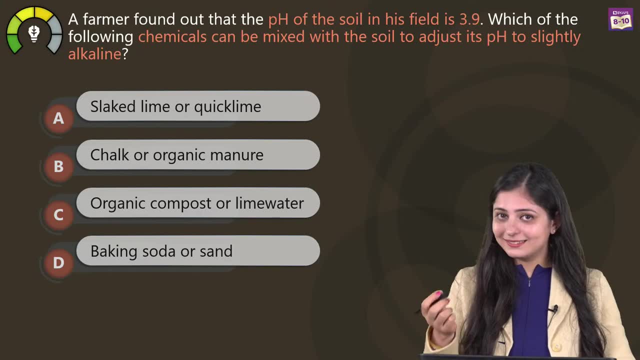 basic substance to it now this basic substance that we need to add we've got so many options of options could answer they come mark the compounds mark the 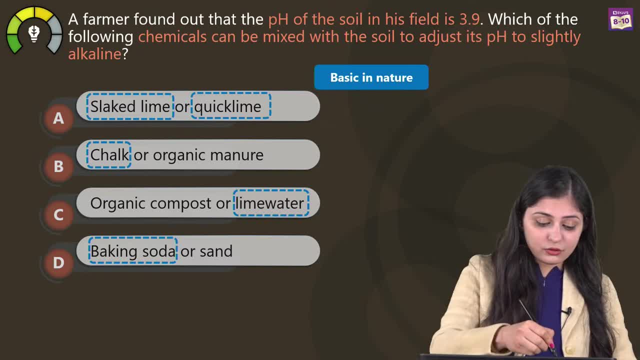 substances which are basic in nature so we've got slaked lime with us that is calcium hydroxide that's a base quick lime 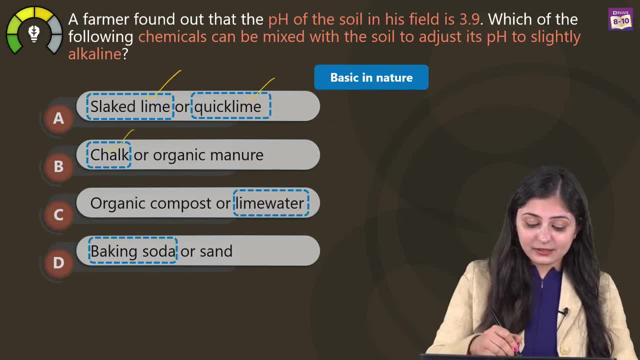 calcium oxide chalk calcium carbonate lime water calcium hydroxide baking soda sodium hydrogen carbonate in any case these compounds are very much basic but 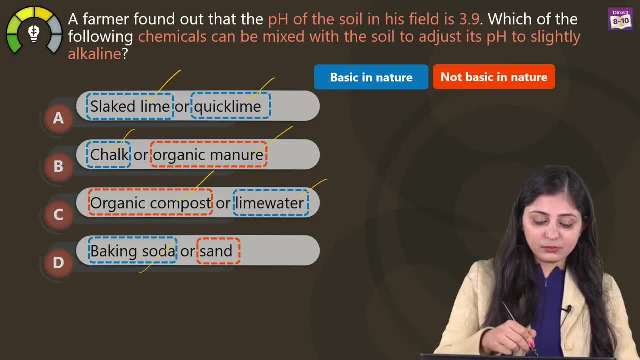 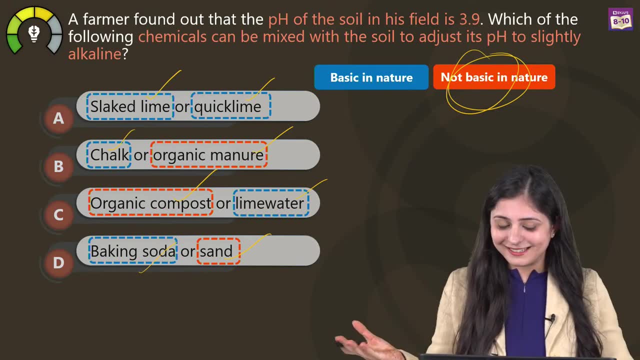 what do we have here we've got organic manure organic compost and sand they are not basic in nature for shaw organic manure organic compost yeah acidic right 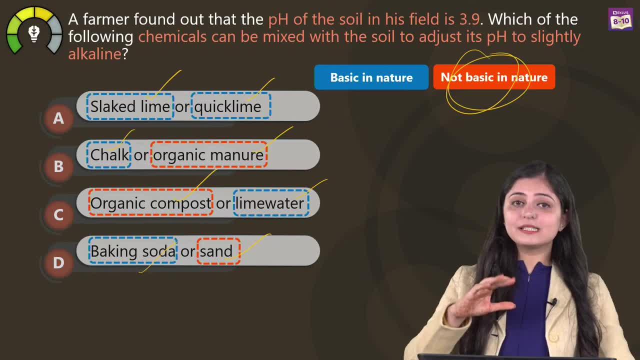 and sand is nothing but silicon dioxide now if the sand is pure and it's made from pure silica 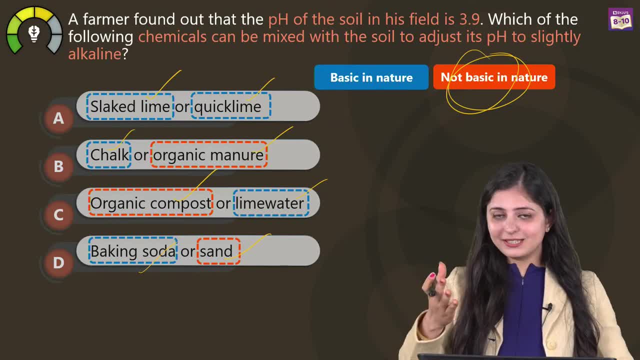 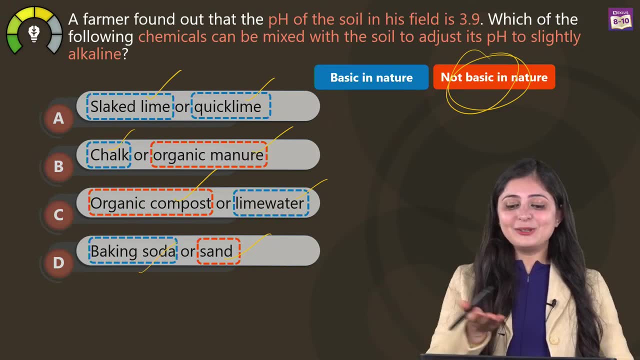 what's the neutral end it'll go body ideal situation a key neutral Jairo acid again neutrally that I'm basic though definitely neither at all so there you go you are left with just one option where in both the substances that they 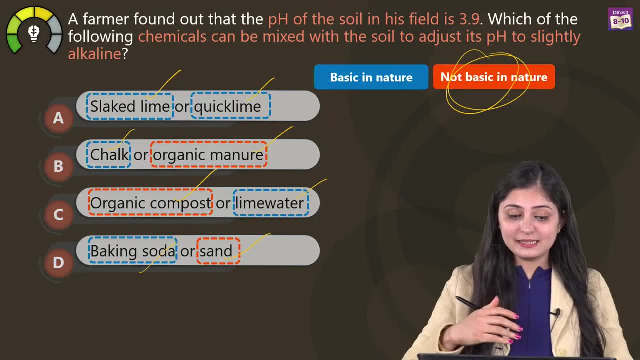 have given you is basic in nature now I see all the answers as a everyone has posted a Kamal says a Kashi says a abhila abhilashini says a part is a 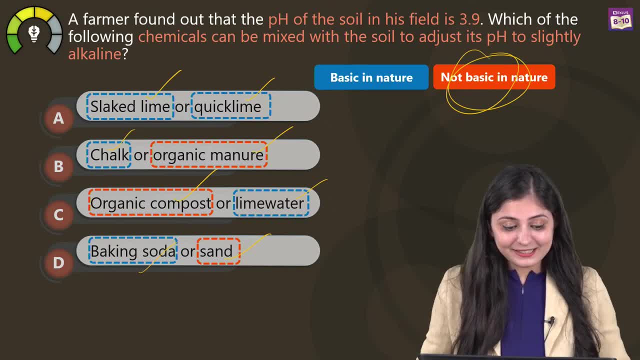 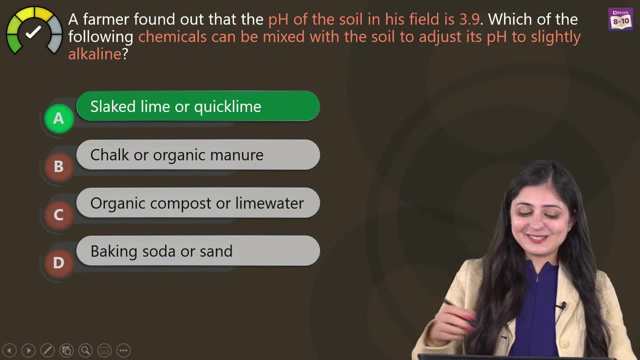 sartrex is a shada says a yaseem says a Sakina says egg that is the correct answer so a is your correct answer which says 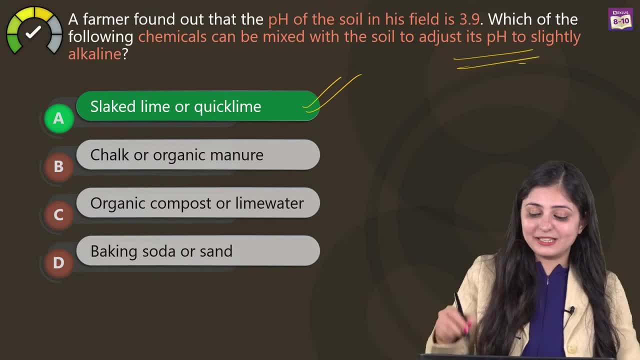 lake lime or quick lime will adjust the pH to the alkaline side very good you will have actually revised and come good I'm happy 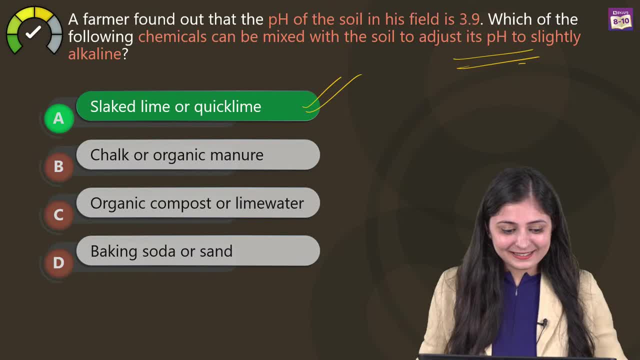 action she also said a utkarsh said a Nikish said a shatak she said slake lime or 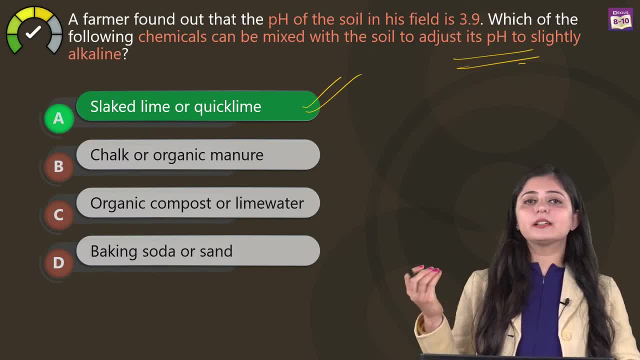 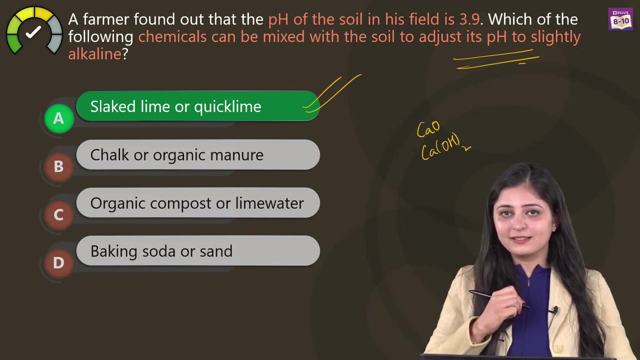 quick lime Asha I have noticed that some of you get confused keys lake lime calcium hydroxide here quick lime calcium hydroxide now what is quick lime it is CAO and what is lake lime calcium hydroxide joke quickly likha jara mo quick lime 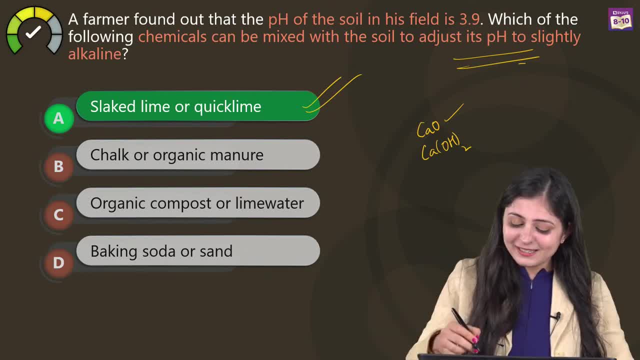 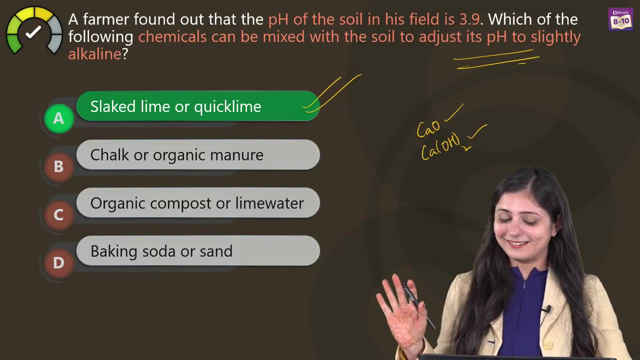 only using tea shaman oxygen are there where is a video catch in hydroxide make calcium be here oxygen here hydrogen be here blag rocket will AG little to beoki will etour knee with her just just a way to remember so quick line is something that you write 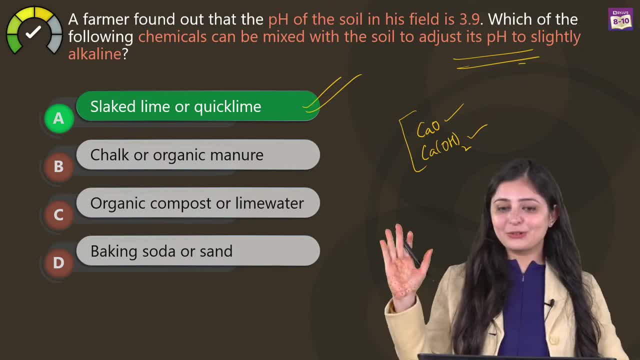 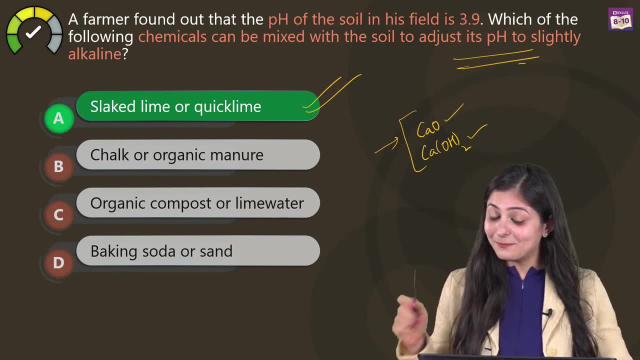 quickly so in Dono may confuse me you na in General cut the quick question I so you should know that quick lime is calcium oxide and in slime is calcium hydroxide okay a bill co 마지막 Al 是 Shinda says calcium hydroxide, snake lime, very good, you are absolutely right. 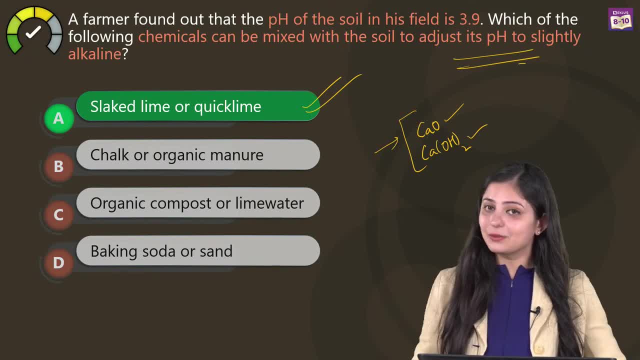 Kashi says calcium oxide is quick lime, yes. Alright, great, great, great. 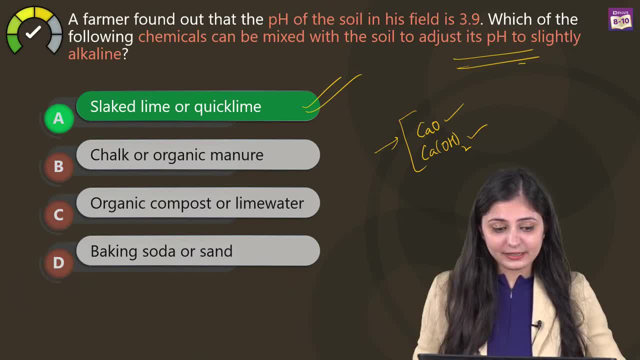 Anjana says your tips are wonderful, alright. These are the tips, keep following them, silly mistakes, all of them will get avoided. 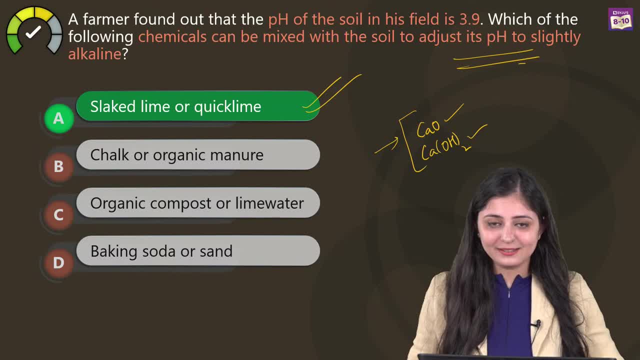 Palak, sorry ma'am, late for the class, no problem Palak, it's okay. 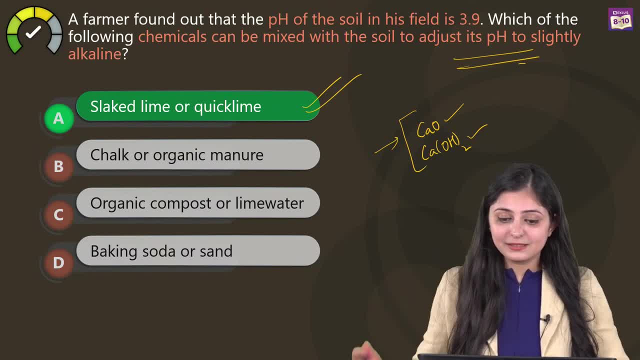 We have just done one question, now you quickly catch up and second ka answer, Palak I am expecting from you also. 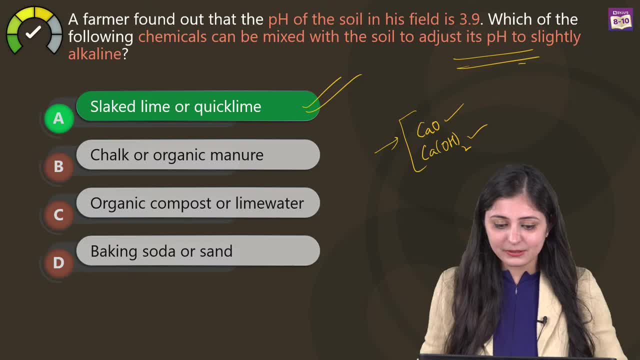 Alright, Ananya says easy to remember now, good. Ab bilkul nahi bhulna, yeh silly mistake bilkul nahi karne. 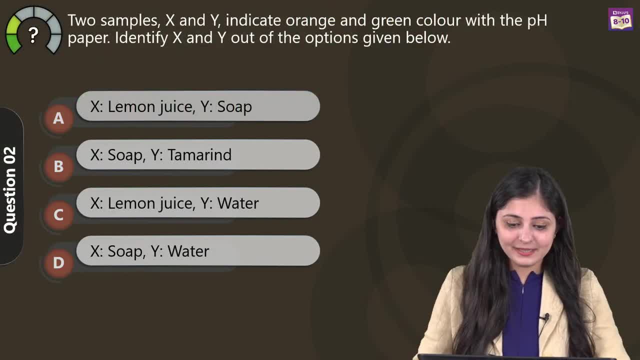 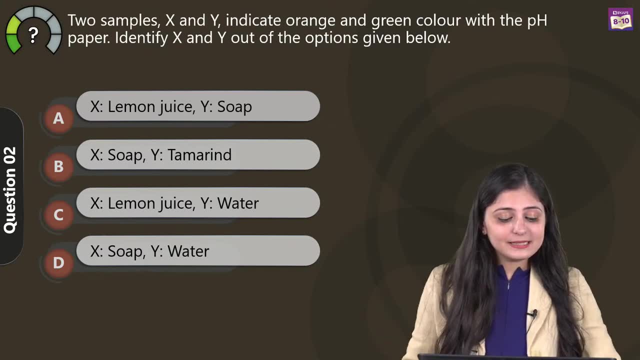 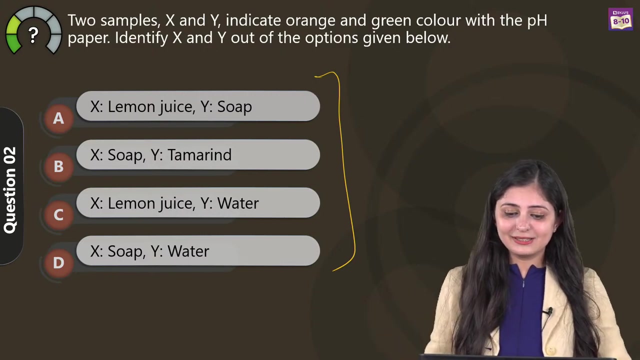 Now moving on to question number 2 that we have. Start solving 2 dash whatever your answer is, meanwhile I am reading the question for you people. Two samples X and Y indicate orange and green colour. Now pH related questions are very, very colourful. Isn't it? Identify X and Y out of the options given below, they have given you 4 options over here, choose the correct option and tell me. 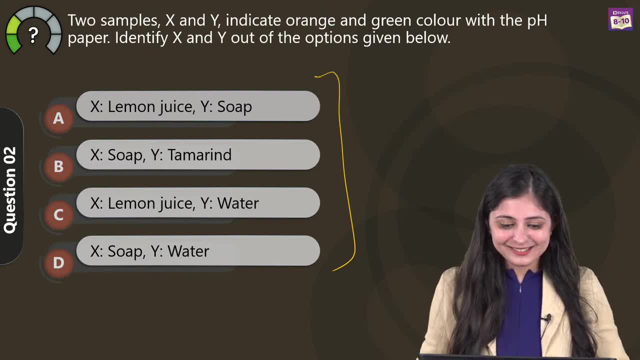 Yes, you are welcome Jai, alright, now I have started getting the answers. Satan says A, Abhijeet says A, Fenel says C, Aditya says C, okay A and C, these are your two probable answers that you think, 50-50 kar diya aap logon hai? 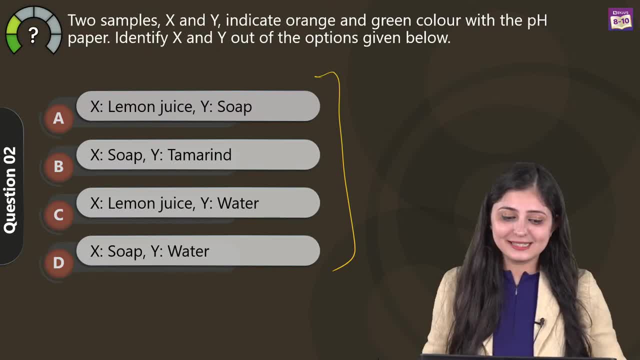 Okay, I can just see A and C on this chat box. 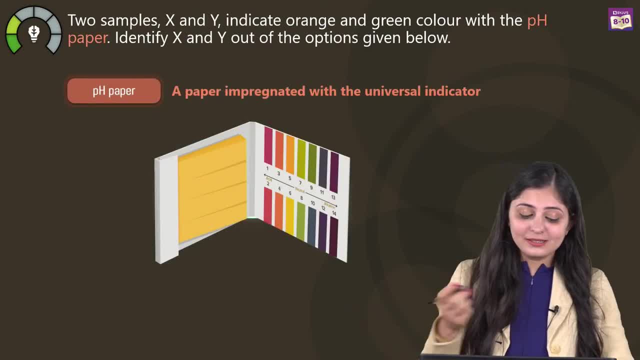 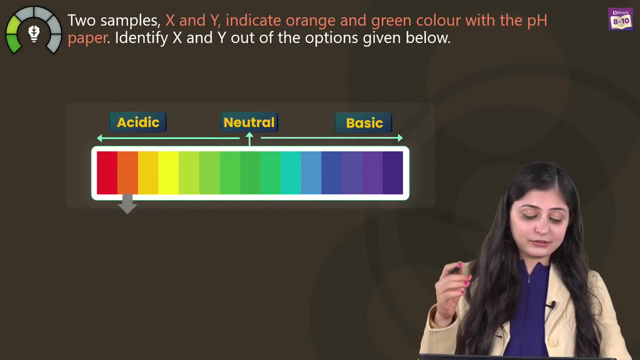 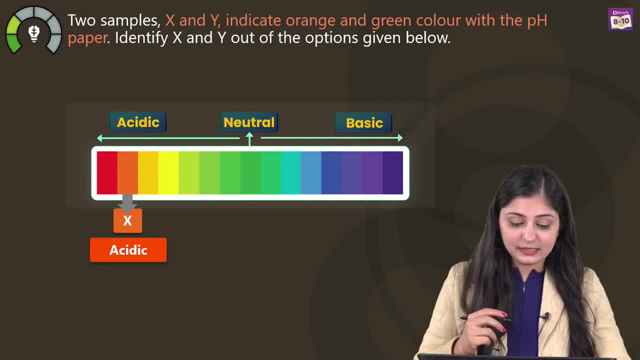 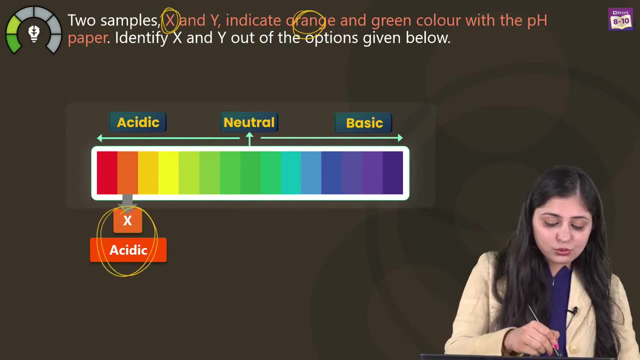 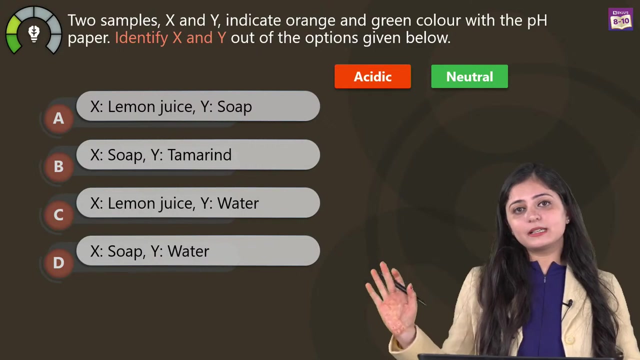 We've got acidity, we've got acidity, we've got acidity. towards the red side we've got basic towards the violet side now they are saying orange is the color that is being shown by X X is showing orange color which means it is acidic Y is showing green color so if Y is showing green color it is neutral now we know that extra matter substance over acidic over why do substance over neutral over now how to quickly eliminate the wrong 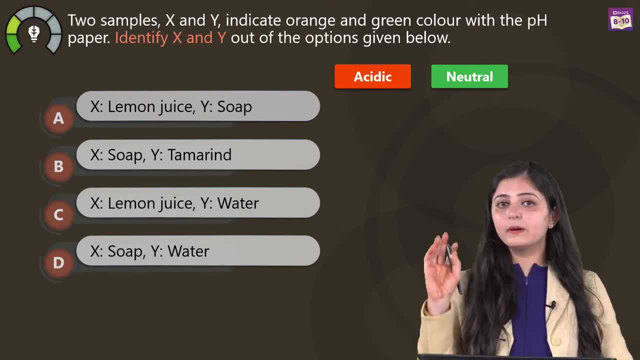 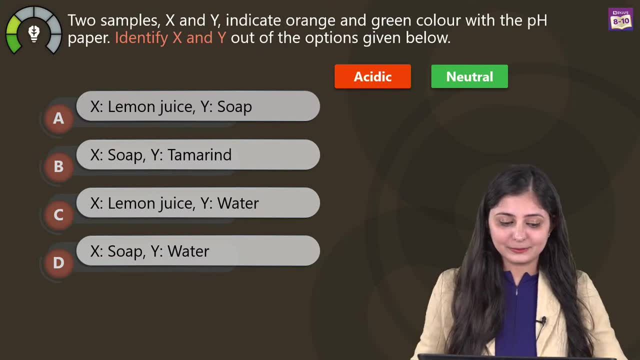 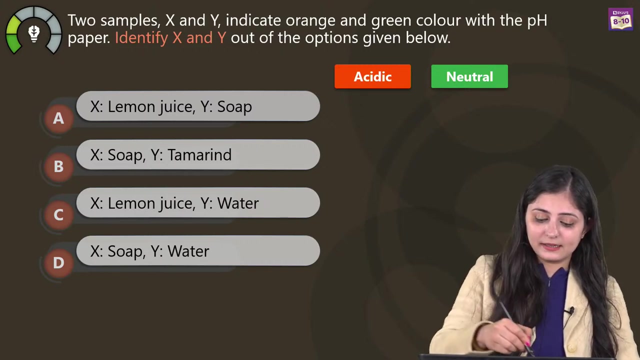 options from here let's see soap kya hota hai what is soap tell me what's the formula kya present hota hai soap mein okay I can see a lot of C's now Akriti says C Amisha says C Abhilashini says C Manoj says C A wale sab gaayab ho gaye ab sirf C dikh raha hai Manoj says basic yes Shanita says basic very good soap sodium hydroxide potassium hydroxide that is basic in nature so jaha jaha bhi aapko soap dikh raha hai you can see here here and here cancel these options kyunki hume to acidic 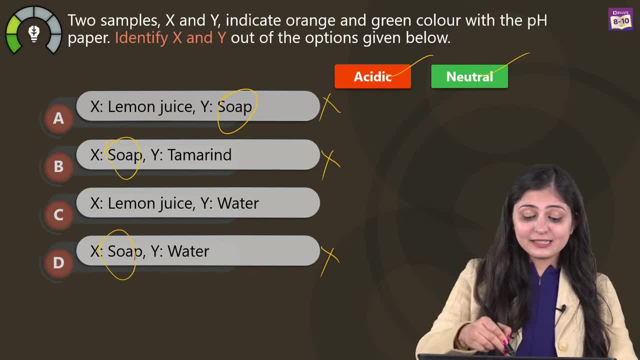 ho neutral se matlab hai basic ka bhi hume kuch karna hi nahi hai so you can 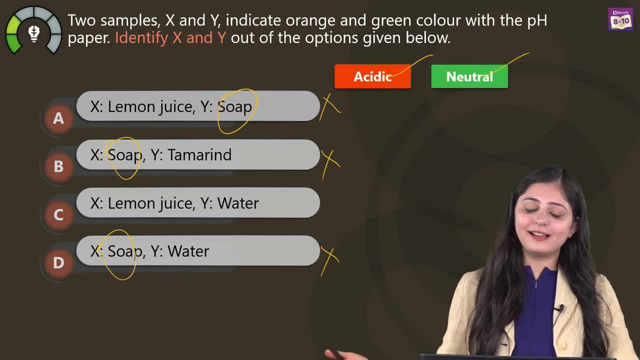 cancel these three options and with that you arrived at the right answer that is options 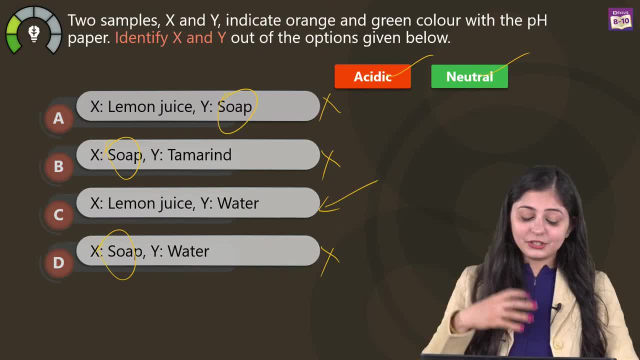 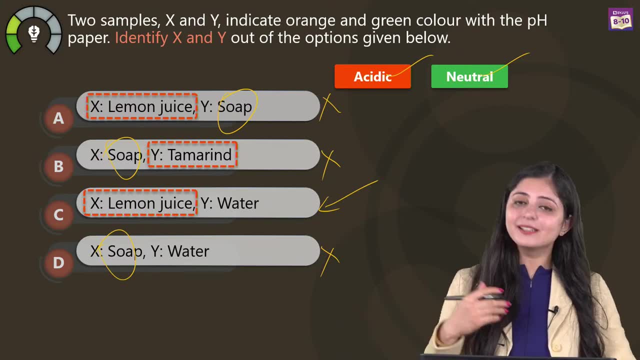 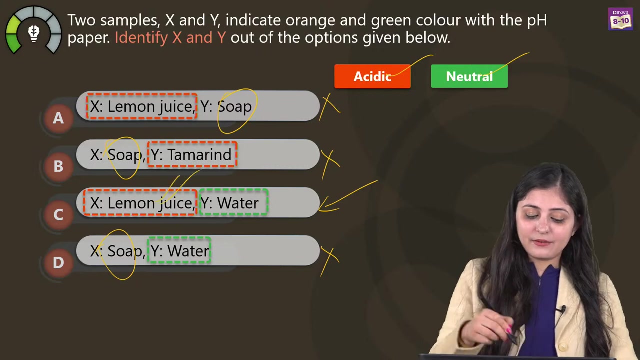 see this is just a shortcut trick to quickly reach at the answer otherwise if you see that lemon juice contains lemons citric acid is there tamarind imli tartaric acid is there so these are the substances which are acidic in nature what a neutral if it's pure definitely it's going to be neutral now the only option there in X is acidic and Y is base Y is neutral is option C so 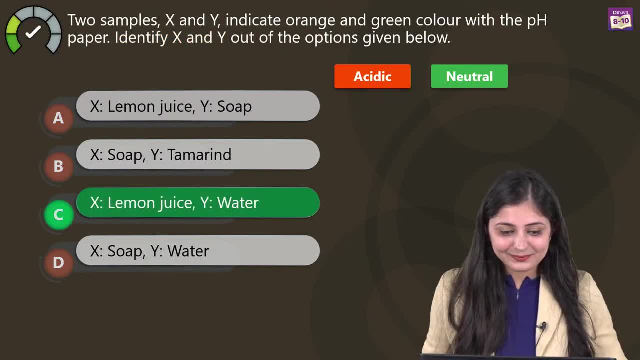 see is a right answer yes Monica you're absolutely right with this Ritisha say see mega say see yes I can says see Abhilashini say see Sabaraj say see Hari Priya say see all right so I think this 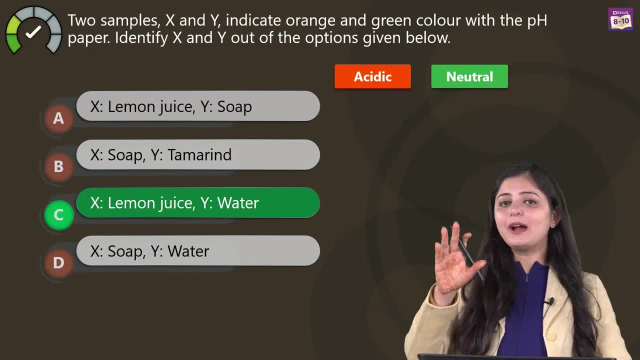 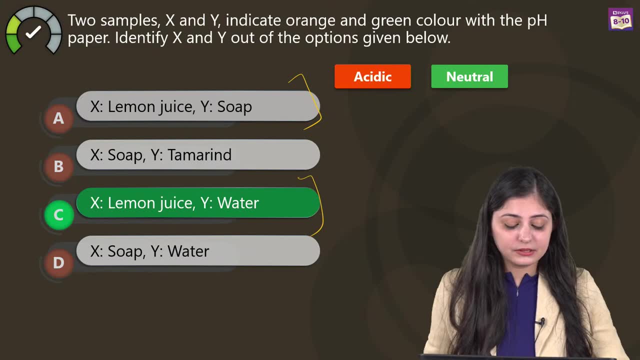 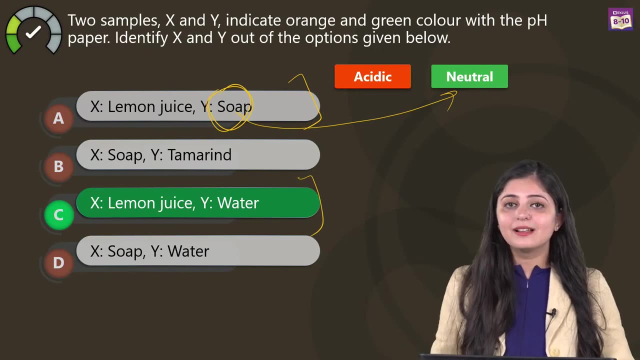 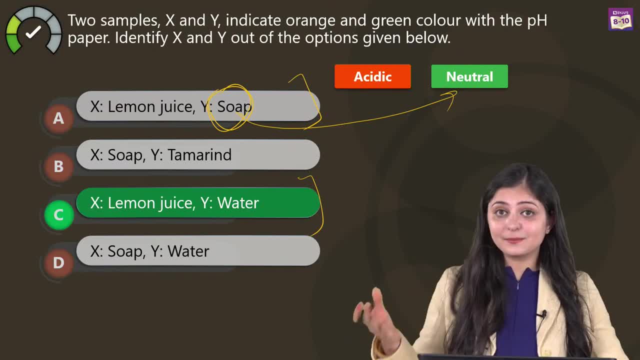 so sodium hydroxide potassium hydroxide it has basis substances in it isn't it so you have eliminated all the options wherein you saw soap all right done 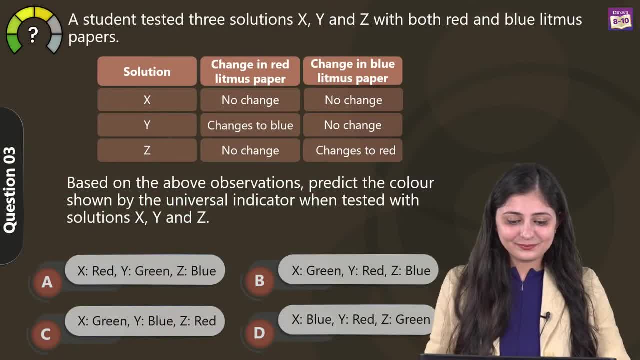 moving on to question number three now a student tested three solutions X Y & Z 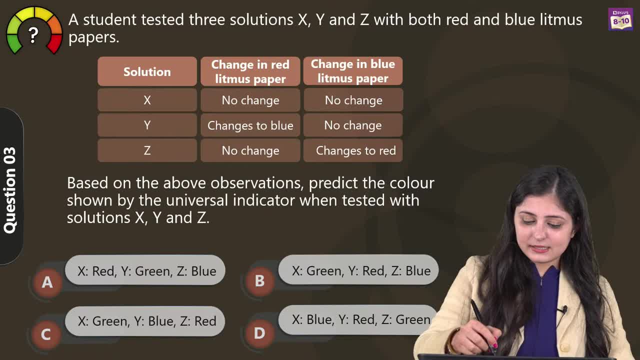 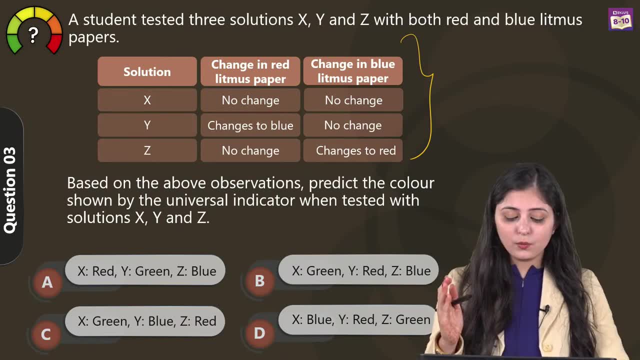 with both red and blue litmus papers this is the observation they have given us over here based on the above observations predict the color shown by the universal indicator when tested with solutions X Y & Z 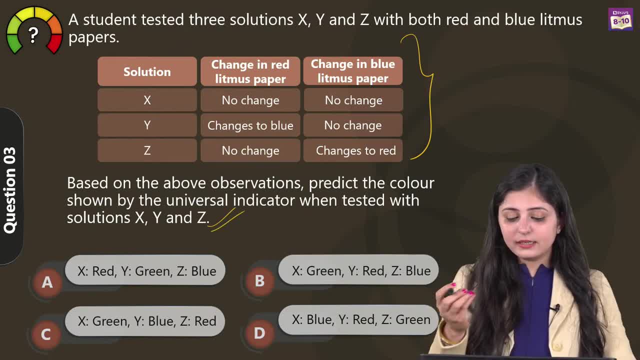 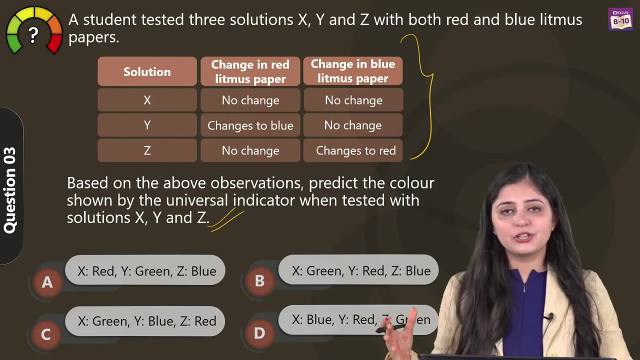 now here you will think that indicator is given color change is given again color change is asked so just a way to confuse you people please look closely they have given you different indicators this question in general deals with litmus and universal indicator but in in the exam you can get any two indicators basic approach that you people need to have is then you will figure out whether the given substance is an acid base or is it neutral then with the second indicator what will be 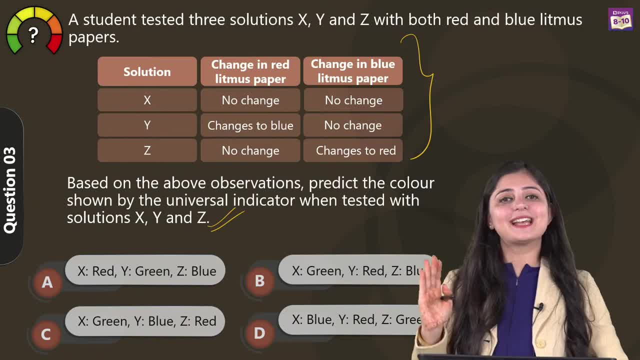 the color change for that acidic substance for that basic substance and for that neutral substance this is the approach this is how you need to proceed 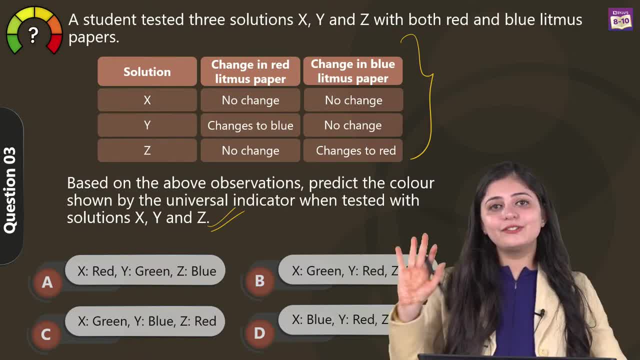 if you get such questions in the exam now I have given you the hint now try solving it man are says C ???????????? 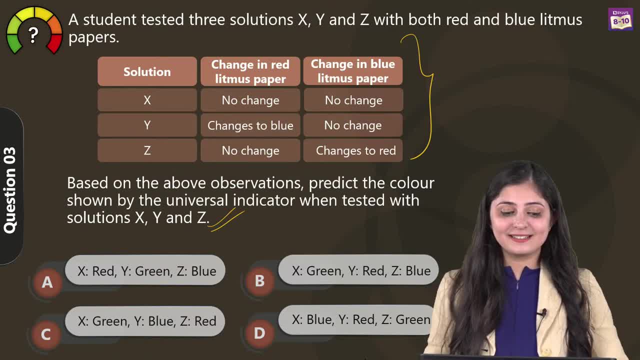 C. Parol says C, 100%. Very good, Parol. You seem pretty confident with this one. Palak says C. Abhilashini says B. Akriti says C. Geeta says C. Life or country says A. Sachin says 300% sure. I think you mean C. Jack Agni says B. Okay, so I think C and B. 90% of you are saying C, but some of you are also saying B. 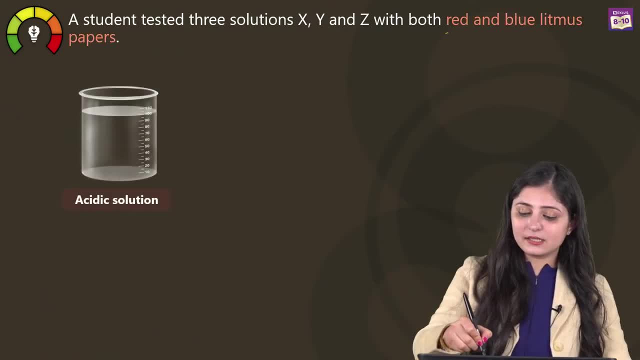 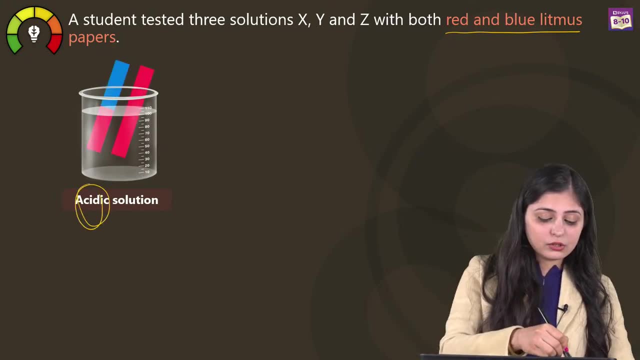 So let's see. Let's start with this. Let's start with red and blue litmus paper that we have. Now, if you dip red and blue litmus paper in an acidic solution, what happens? You will notice that red litmus paper remains red. There is no color change, but the blue litmus paper changes to red in acidic solution. 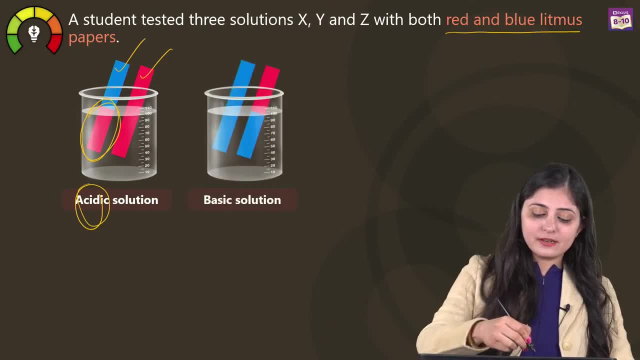 Now, do the same with the basic one. What will happen? The blue litmus paper remains blue, but the red litmus paper, it changes to blue color. 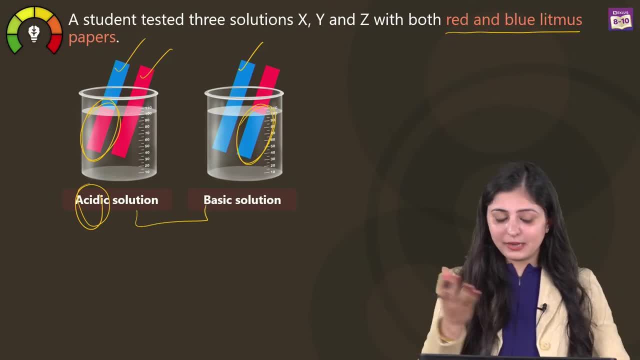 Now, again, one small trick. To help you people, how will you know that what color change is happening in acid and what is happening in base? Base starts with B. Blue starts with B. 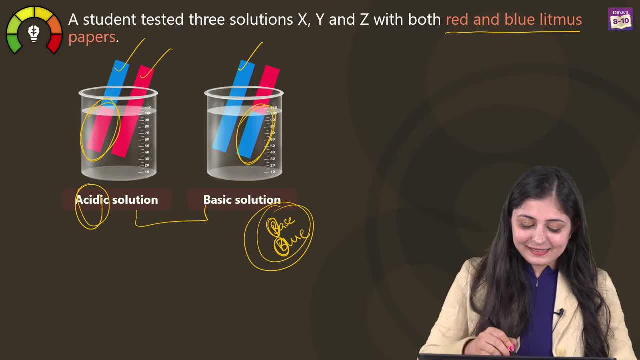 Now, you will remember. So, in base, the ultimate color change is going to be blue. If it's already blue, it will remain blue. 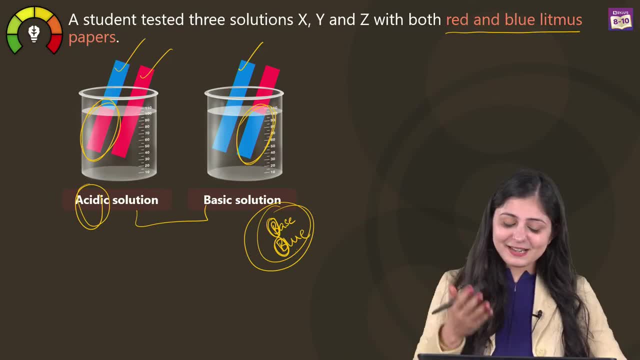 If it is not blue, if it is red, if you have red litmus paper, it will change to blue. Guys, this is just 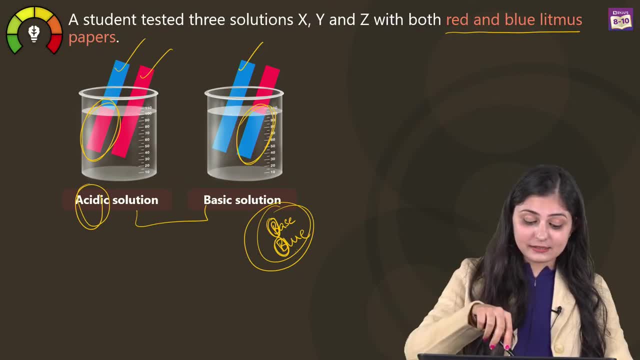 to identify between acidic and basic solution. That is it. 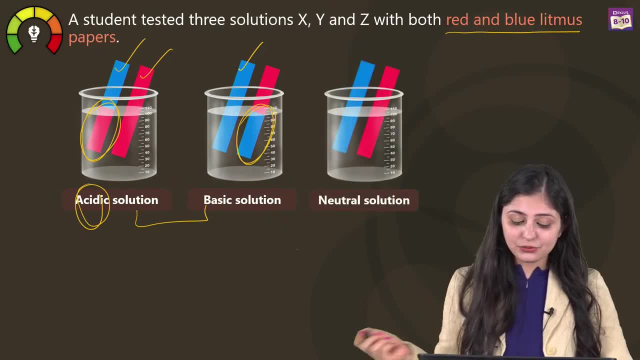 It is only for these two. Because next, what I am telling you is neutral solution. Now, neutral solution, no color change. Red remains red, blue remains blue. So, what I have told you is just to decide between acidic and basic solution. Hi, Sushil. 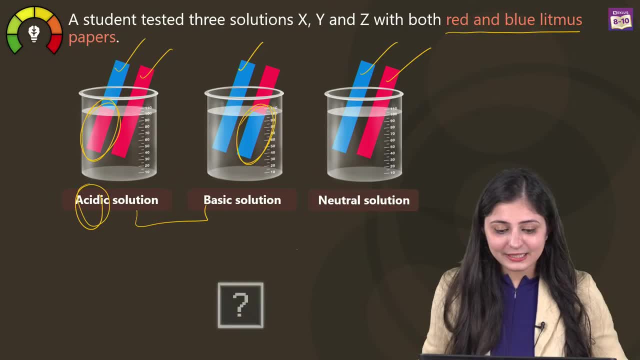 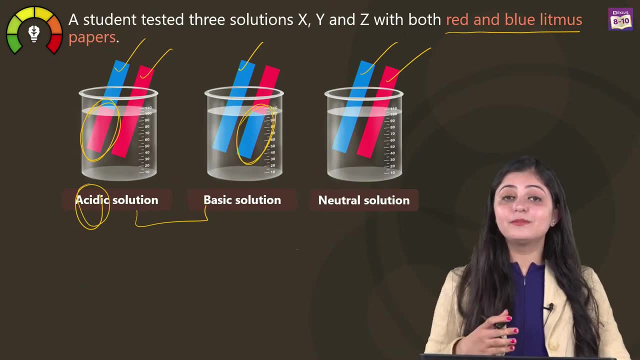 Manoj says, thank you. These tricks are very helpful. So, if you want to know, if we are sharing little hacks here and there with you people, we are expecting full marks in return. 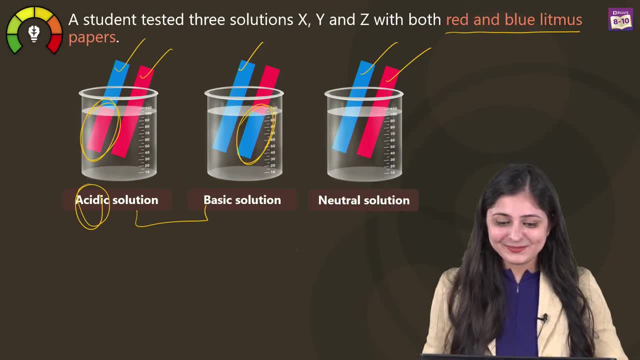 Bata chal raha hai, full marks aane chahiye return mein. All right. 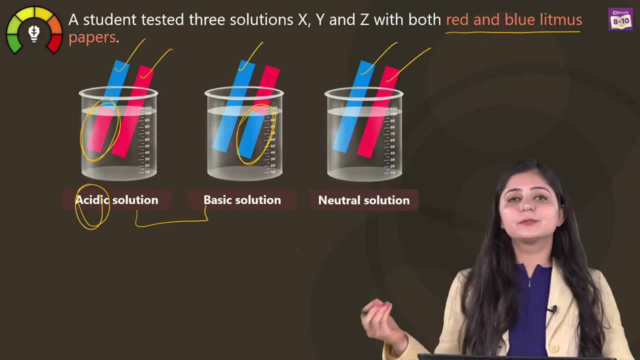 Now, this much we know ki up acidic solution mein final kya color change hai, base mein kya hai and neutral mein kya hai. Now, what do we have here? They have given us this in the question. Question mein pehle hi ye given hai. 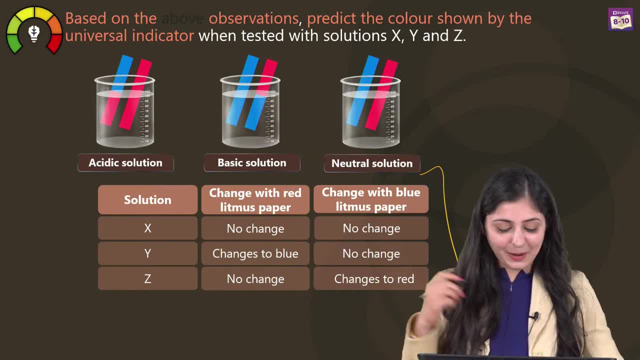 Ashi says C. OK. Ashi will just come to it. Very quickly. 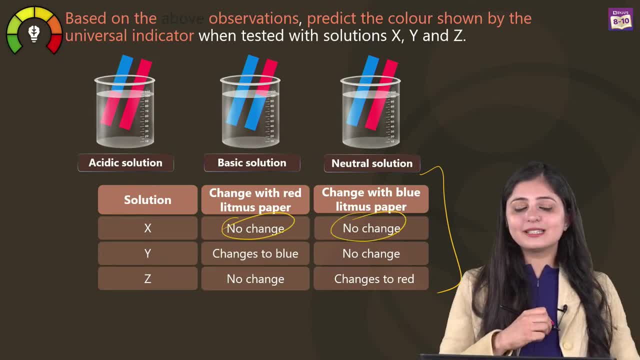 X is not showing any change in color. What is the nature of X? It's going to be neutral. 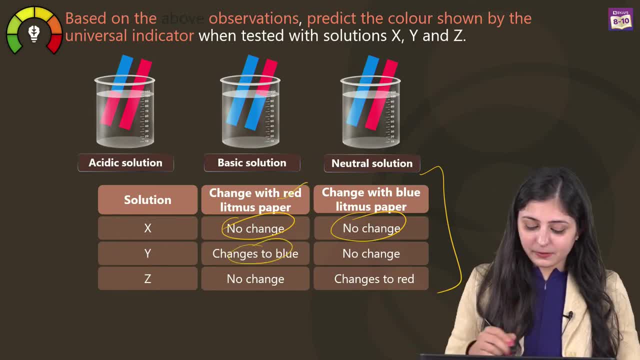 Y changes to blue with red litmus paper and no change with blue litmus paper. 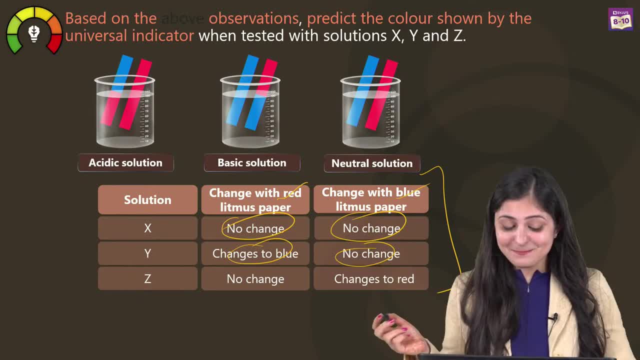 B, blue. B, basic. What is going to be Y? It's going to be basic in nature. 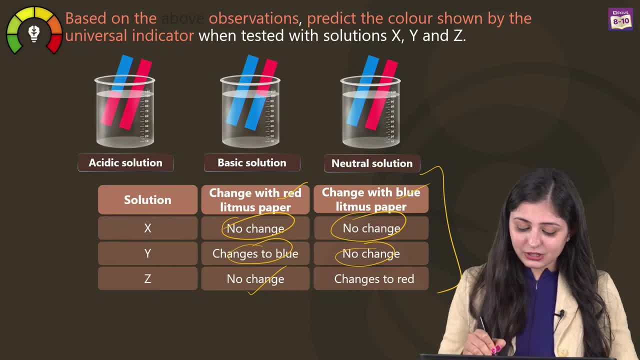 And Z is not showing any change with red litmus paper, but it changes to red with blue litmus paper. So, it's going to be acidic. 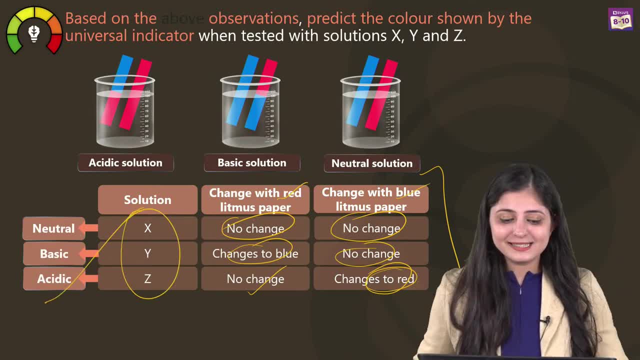 So, there you go. You've identified the nature of all these substances. I have noticed one thing. 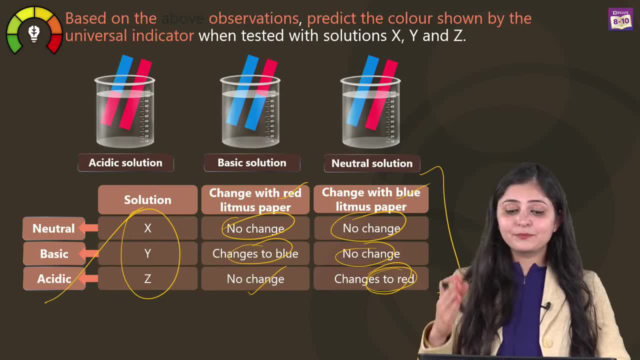 You people start with random options, but then slowly, as I explained, you are repeating and writing the correct answer. That is great. 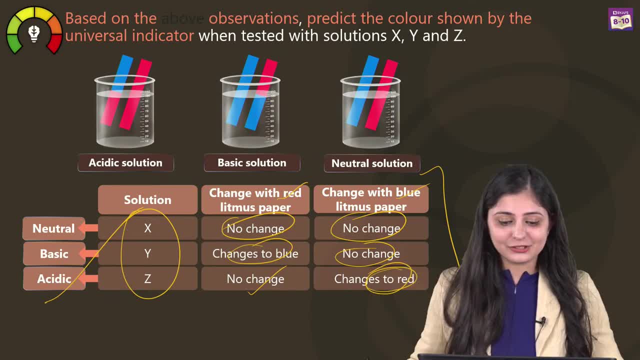 That means you're understanding how to proceed if you get such a question. Yes, absolutely right. 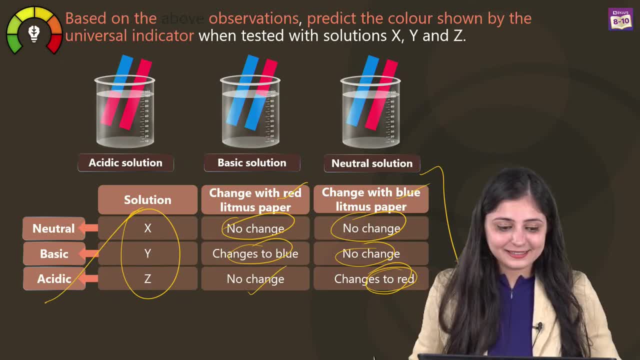 Haripriya, you're absolutely right. Samojit, you are correct. Samovi, you are also right. All right. So, now we know what X, Y and Z are. We have known this. Universal indicator. 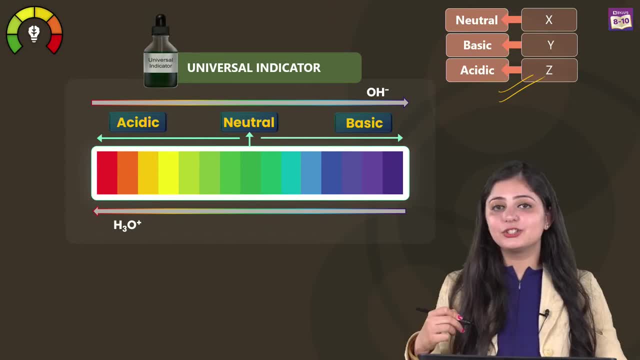 Now, we have taken another indicator. With this, what changes will X show, what will Y do and what will Z do? Let's see. 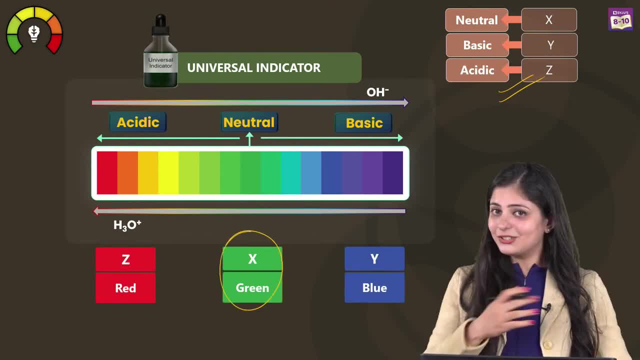 Now, X was neutral. We just found that out, isn't it? If it is neutral, it's going to show green color. Simple. Now. 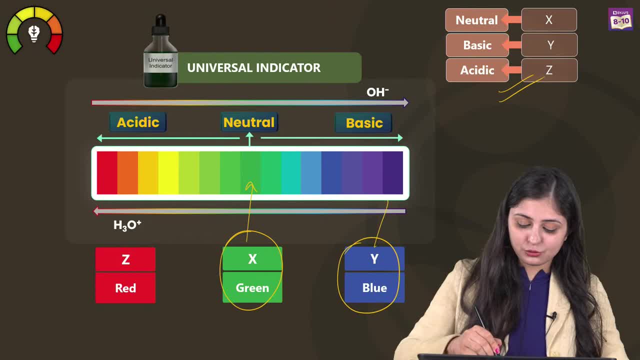 Y is basic. It's going to show shades of blue. Z was acidic. It's going to show shades of red. 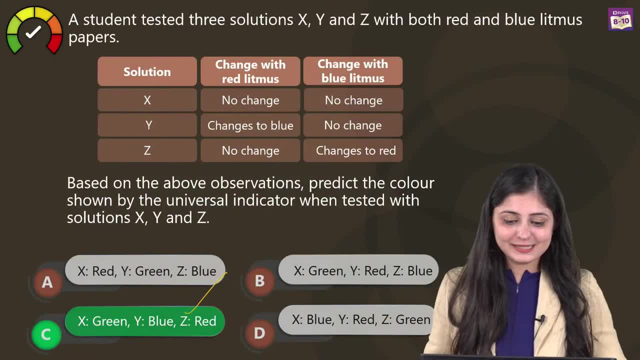 And there you go. This is the correct option. Option C. Sakshi, you're right. 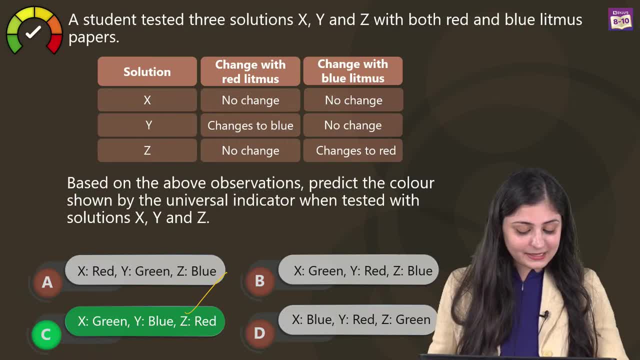 Abhilashini says X is neutral. Yes. Y is basic. Very good. And Z is acidic. Absolutely right. Umama says, I knew it. Very good. 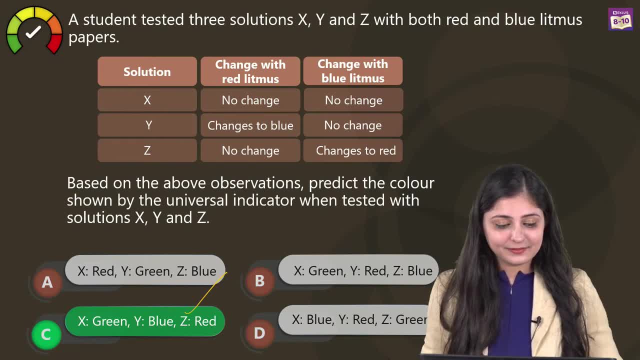 Sharda says, my right answer is C. 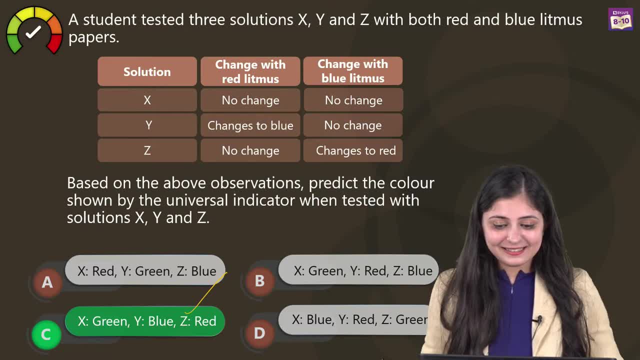 Ashi is saying C. Shankar C. All right. 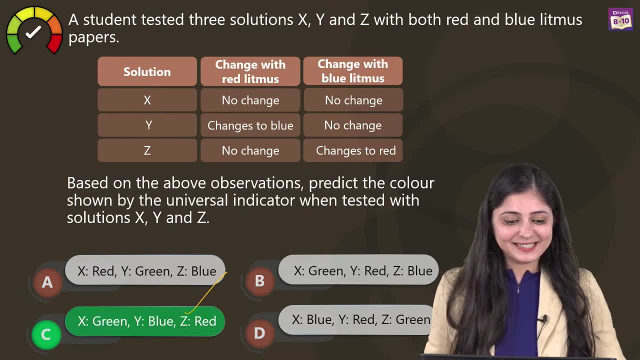 Great yaar, sab padke aaye hain. Abhijeet also said C. Paj said C. Great, great, great. 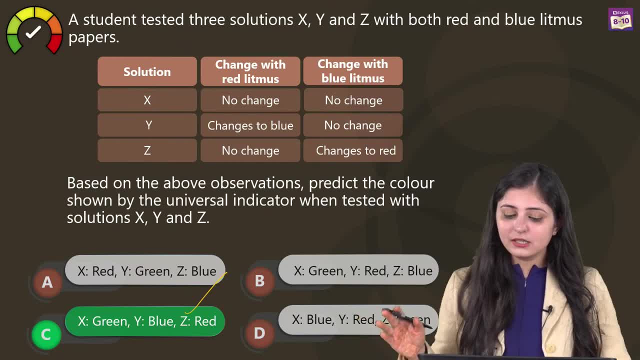 So, you people understood how to go about such questions. So, don't leave such questions yaar. 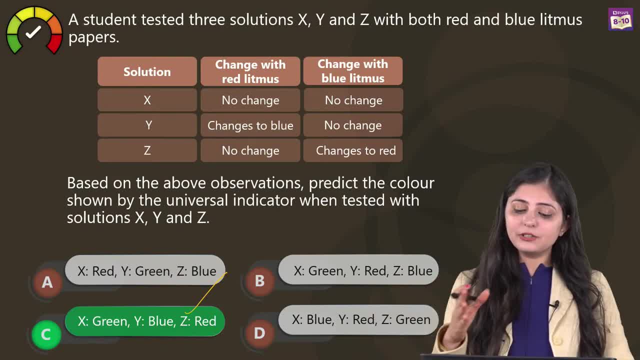 Basic color change is mein yaad karke jaana hai. Color change pata hoga na, then you can easily attempt these questions. 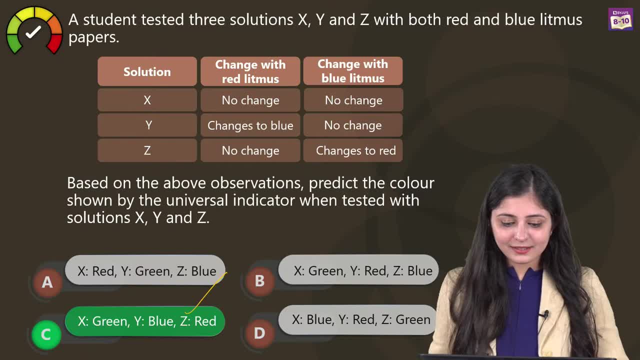 Now, aage pade? 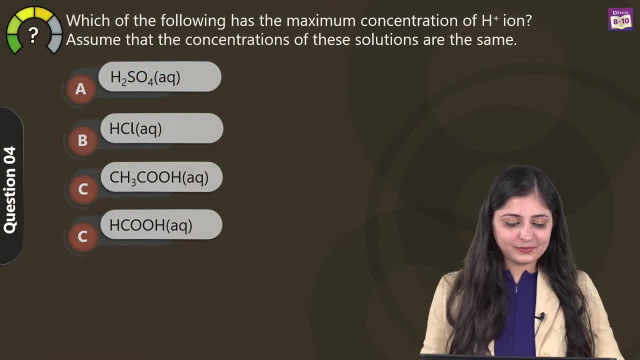 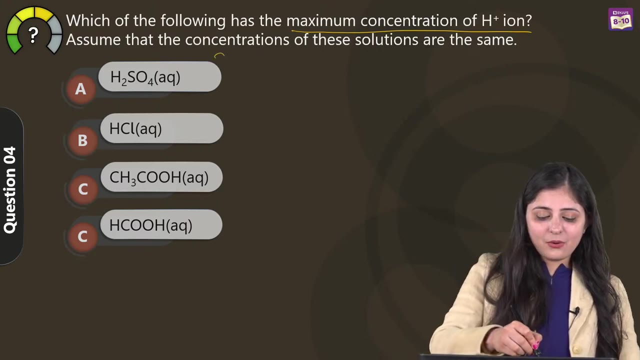 All right, moving on to question number four now. Which of the following has the maximum concentration of H plus ion? Assume that the concentrations of these solutions are the same. Chalo, attempt karo and tell me the answer. You've got four options over here. Let's see who is going to answer this first. 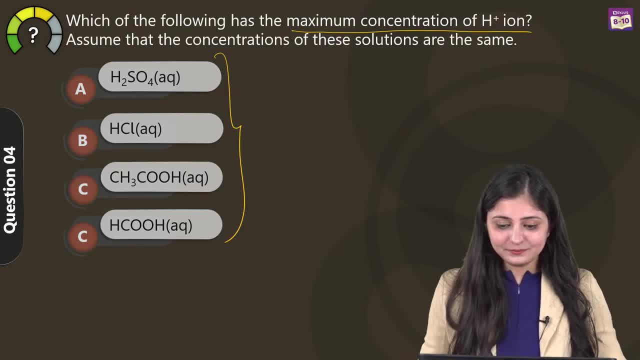 Okay, Fennel has answered B. Okay. Sameeksha says B. Hrithisha says C. Shailaja says A. 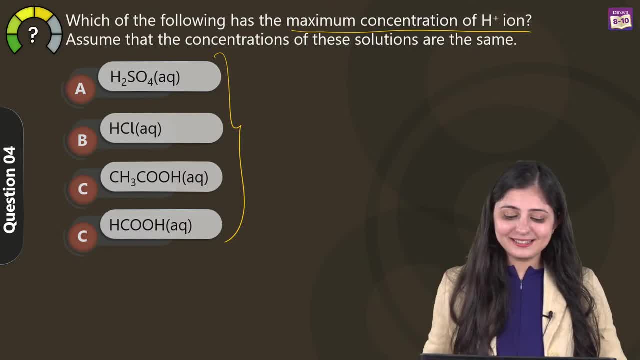 Ayush says A. Sakina thoda sa confused hai ki A hoga ki B hoga. 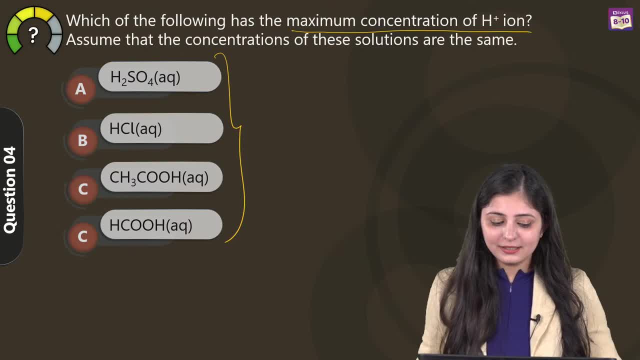 And I think Sakina ka jo doubt hai na, wo mostly aap sab ka doubt hoga ki answer A ya B mese kuch hai. 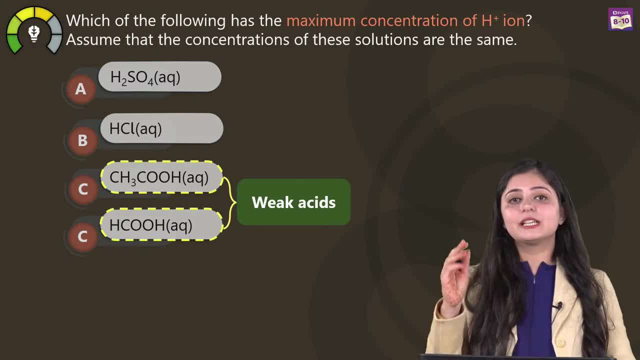 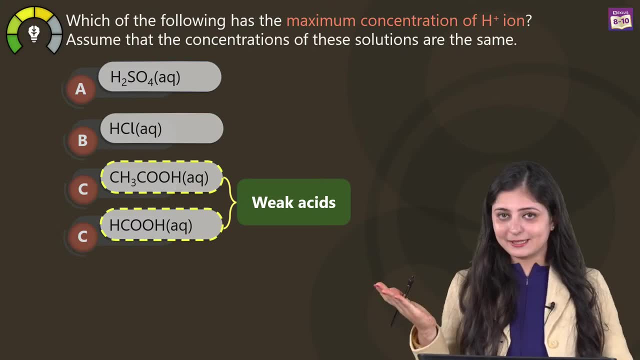 Well, maximum concentration of H plus ion. Jaise hi hum maximum concentration ki baat kar rahe hain. If you see any basic substance in the options, eliminate that. Baj gaye acids. If you see weak acids, those are also wrong options. 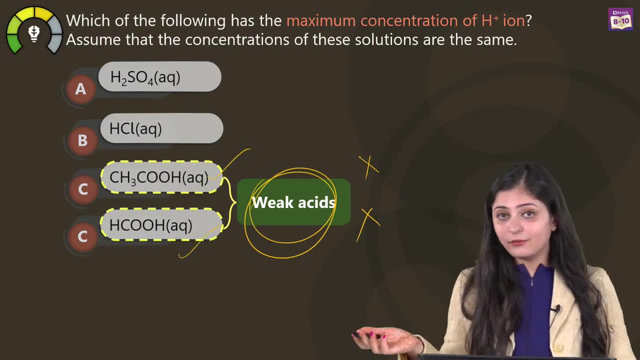 So, acetic acid hai, ya methanoic acid hai, formic acid hai, weak acids. Weak acids mein obviously concentration of H plus ion is going to be less. It's not going to be maximum for sure. 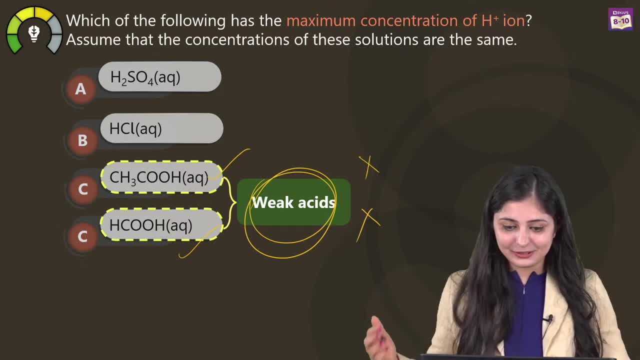 Basic substances and weak acids can easily be eliminated. 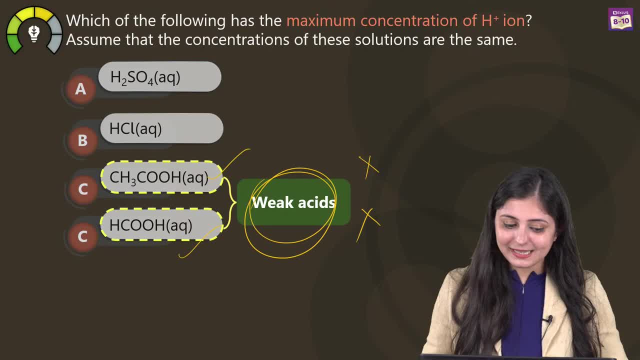 Sanya is also confused, A or B. Priyanchu says A, Akshat says B, Ashmita says B. 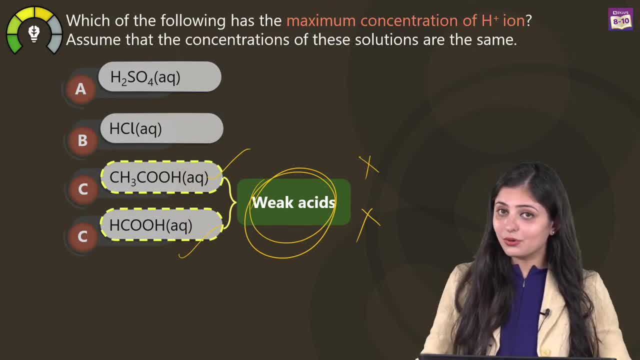 Guys, please note, are they asking which is a stronger acid or are they asking maximum concentration of H plus ion? Alright, let's see how we have to proceed with such questions. Now, weak acids, they dissociate incompletely in aqua solution. 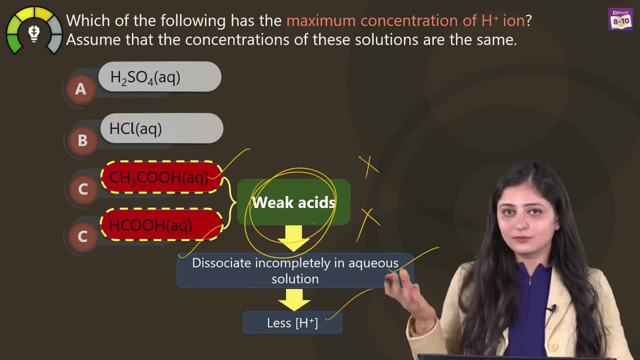 So, obviously, very less H plus ions concentration is being generated in this case. 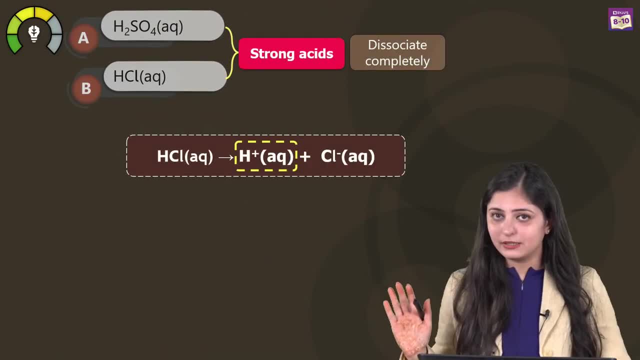 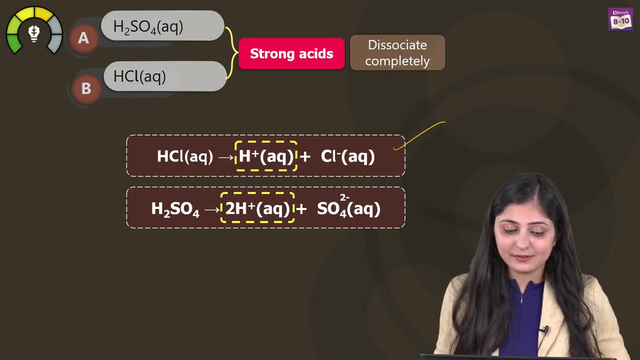 Now, we are left with strong acids. They dissociate completely. Wo poore ionise ho rahe hain. So, let's start with HCl. HCl ko, if you add it to water, it's going to break into ions. And this is how the equation looks like. Let's do it with H2SO4 also. Let's add that to water as well. And this is how the equation is going to be. 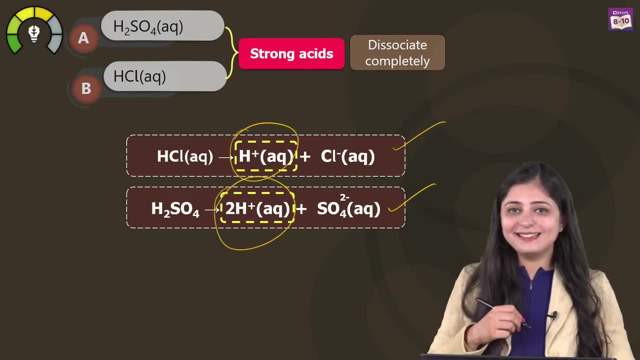 Now, over here, clearly we can see that H2SO4 is having higher H plus ion concentration. Sameer says it was too easy. 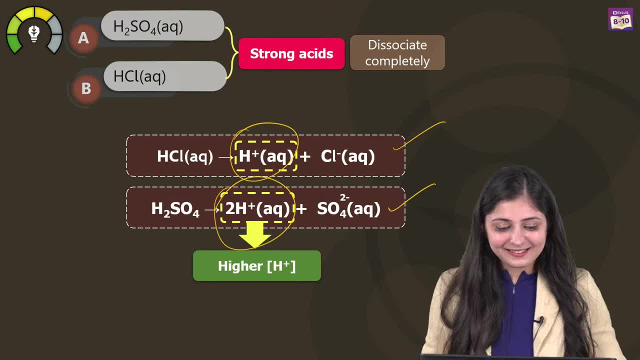 Harry said A, right, great. 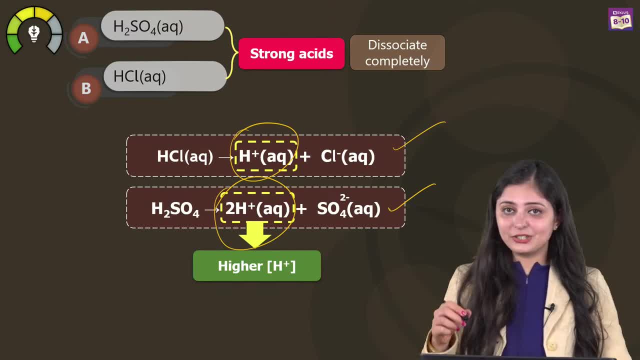 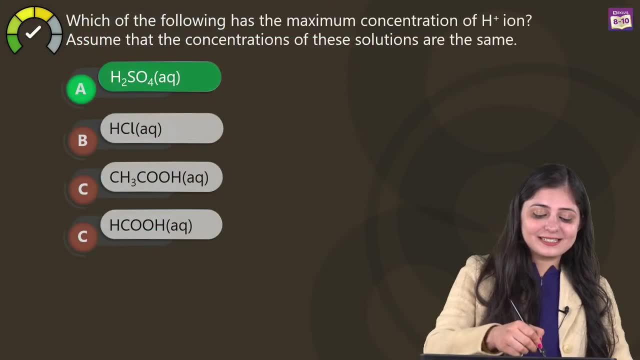 So, you can see it's getting dissociated into H plus in this case and 2H plus in this case. So, which is having higher H plus ion concentration? It is H2SO4. H2SO4. 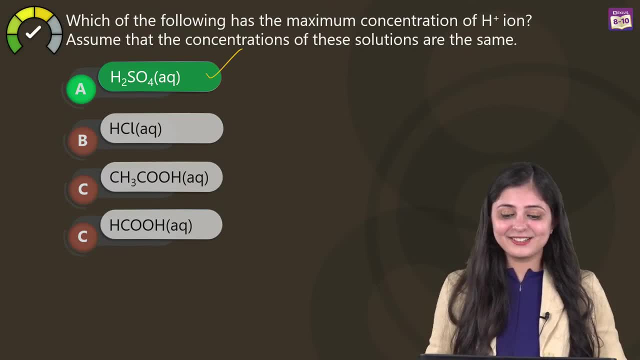 Ayush said A, Bharat said A, Geeta said A, Aryan said A, great, great, great. 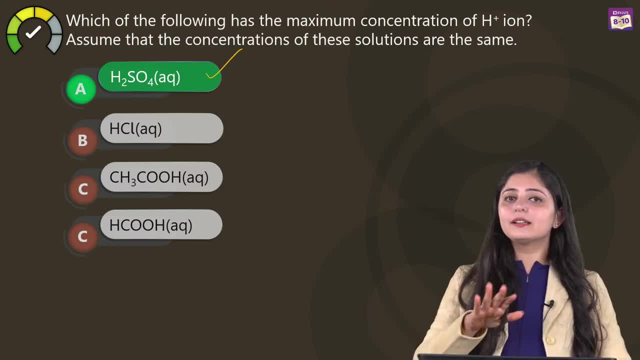 Why are we bringing these questions? Because we know that these questions are a little tricky. 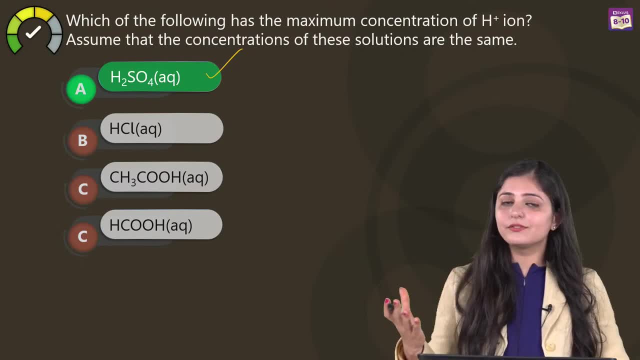 These are the questions wherein you might, you know, get confused in the exam. Yaha pe jitna confused hona hai holo, waha pe bohot confident hoke jaana hai. So, all confusions are out there. Over there, only confidence. 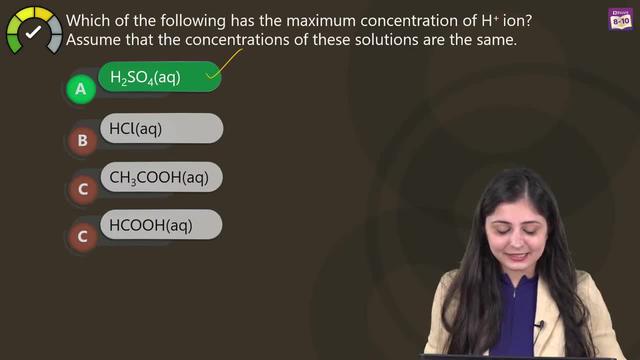 Kamal says, now the question is clear. Great, Kamal. So, there is no harm in going wrong, yaar. 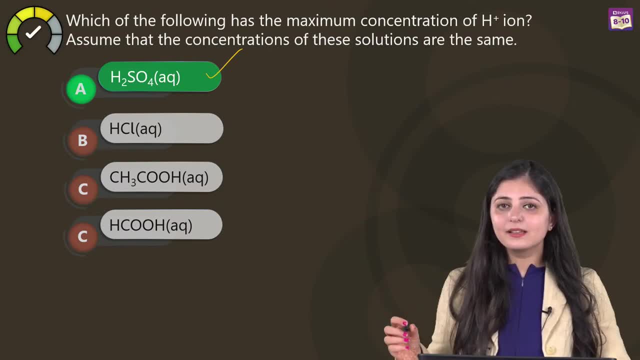 Yaha pe jo marzi karlo, jitni galti karlo, waha pe our main aim is to score well there, to ace the exam, to ace the board exam, isn't it? 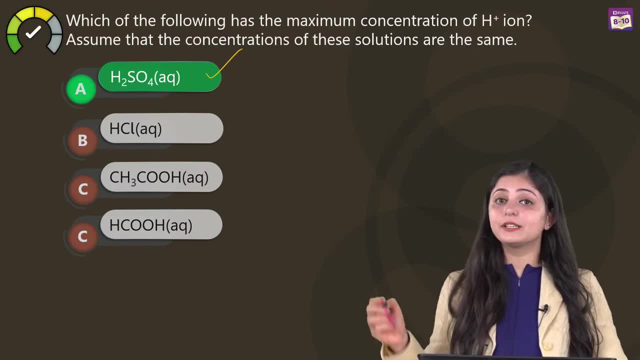 Ayush is saying, ma'am, what is H3O plus? Hydronium ion, Ayush, we did it in the last class. 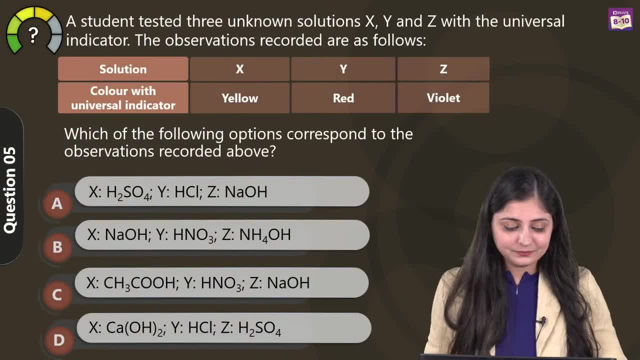 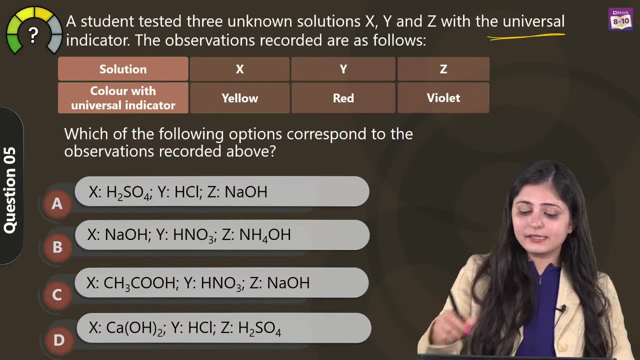 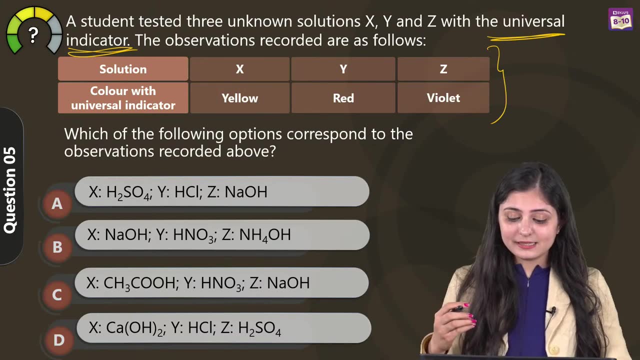 All right, now, moving on to question number five. A student tested three unknown solutions, X, Y and Z with a universal indicator. Bohot simple question hai. Itse difficult question abhi am discuss kar chuke. These are the observation, X is showing yellow, Y is showing red, Z is showing violet. 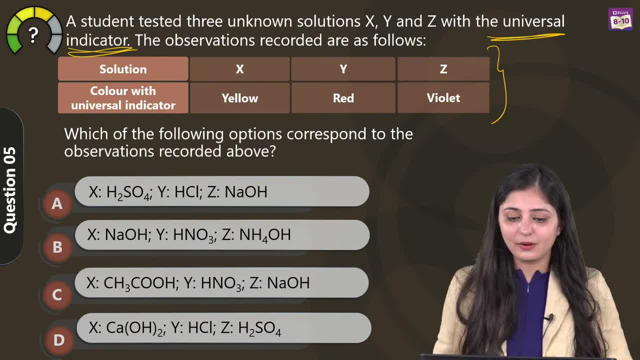 Which of the following options correspond to the observations recorded above? 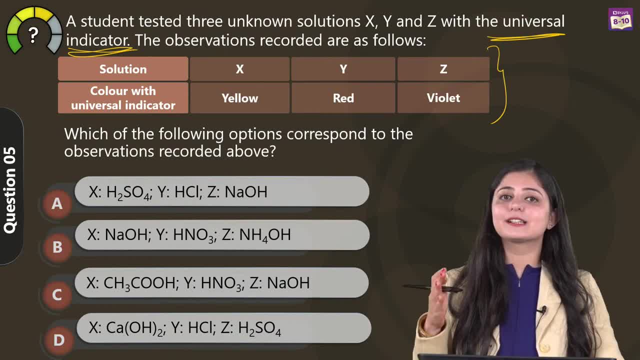 We've already done such a question, colour based question am kar chuke and yeh uska simplified version, I would say. 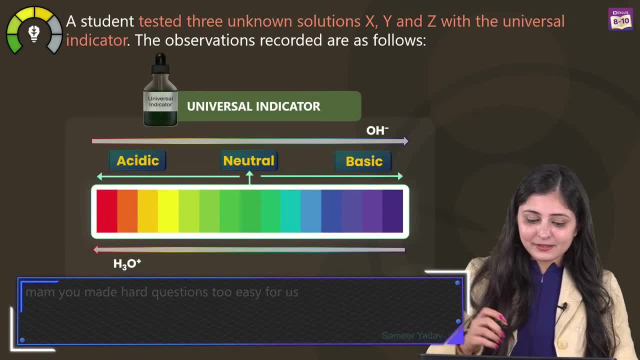 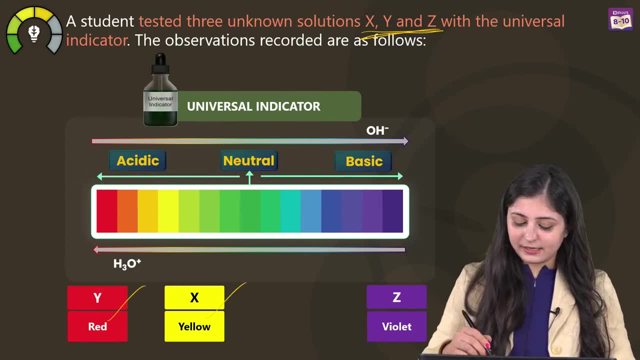 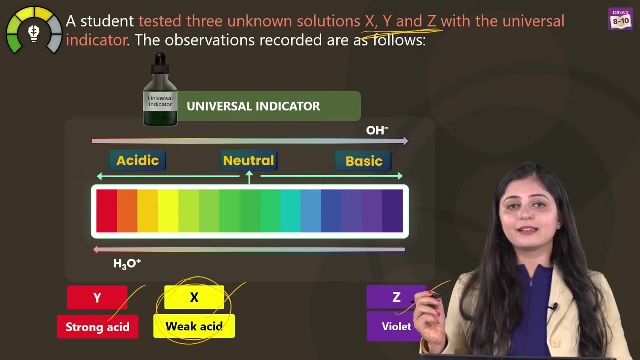 So, what basically they are saying is, they are saying that we've got these three solutions with us. X is showing yellow colour, Y is showing red colour and Z is showing violet colour. Universal indicator ko yaad karo, kya hai? Agar hum X ki baat kar rahe hain, now, Y, X and Z, tino substances hai, X se start karte hain. Kyo colour show kar raha hai, it's going to be a weak acid. 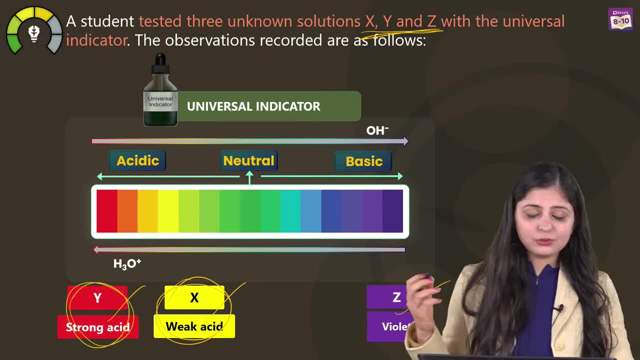 Acid ek side pe hoga but weak acid. Y showing red colour, strong acid, see, over here. 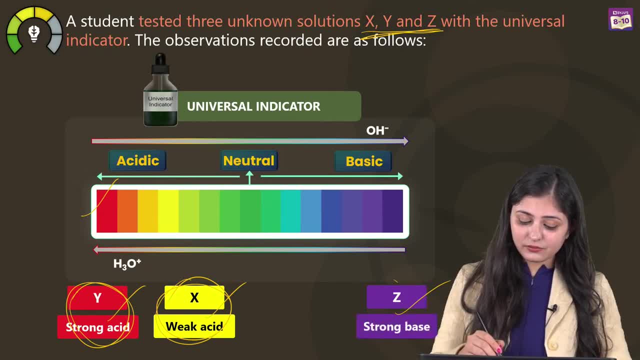 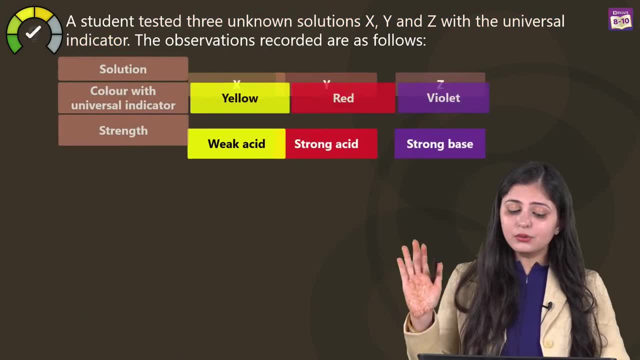 Then, you have Z showing violet colour, so it's a strong base. Now, you know what X, Y and Z are. You know that X is your weak acid, Y is your strong acid and Z is your strong base. 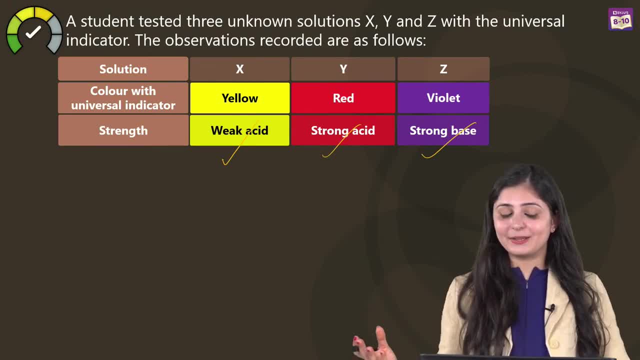 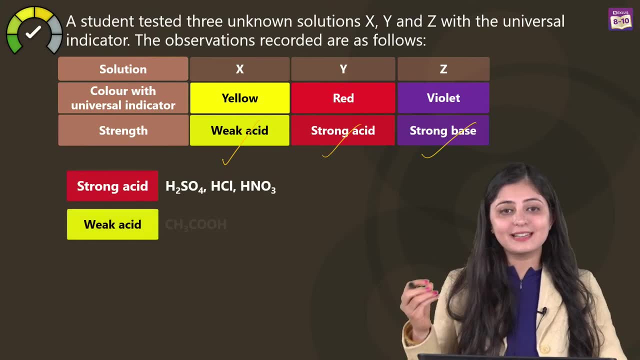 Ab kya karna hai isme? Ab toh sirf substances identify karna hai. Now, a lot of options were being given to you, right? What we've done is, we've categorized these options into strong acid, strong base, weak acid and weak base. 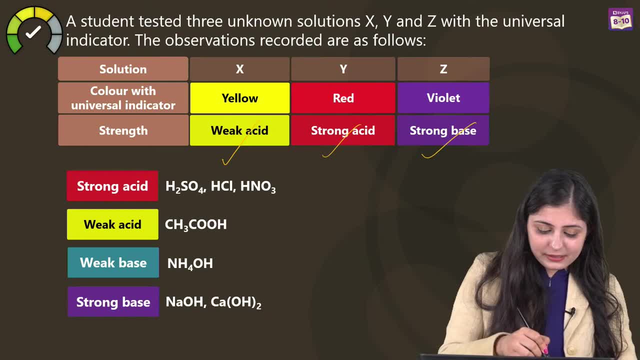 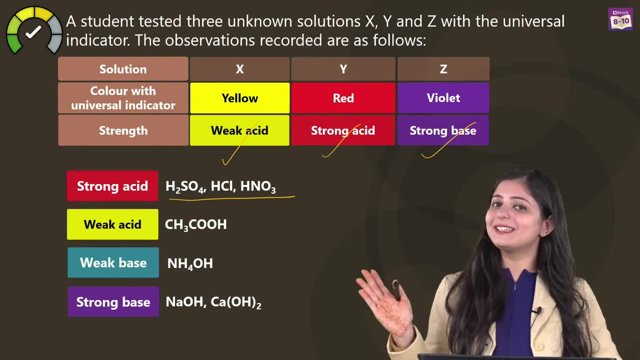 So, whatever options were being given to you out of these, these are strong acids. Sulfuric acid, hydrochloric acid, nitric acid, all are very very strong. 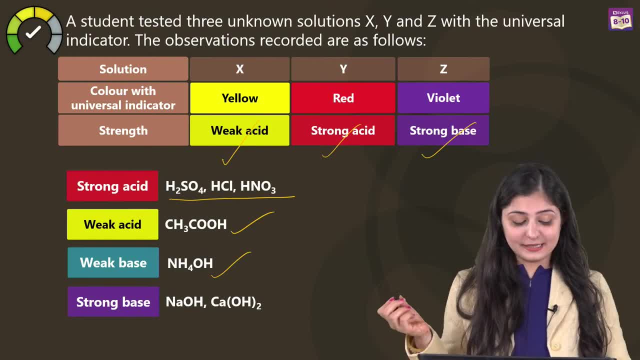 Acetic acid is weak, ammonium hydroxide is a weak base and you've got sodium hydroxide and calcium hydroxide. 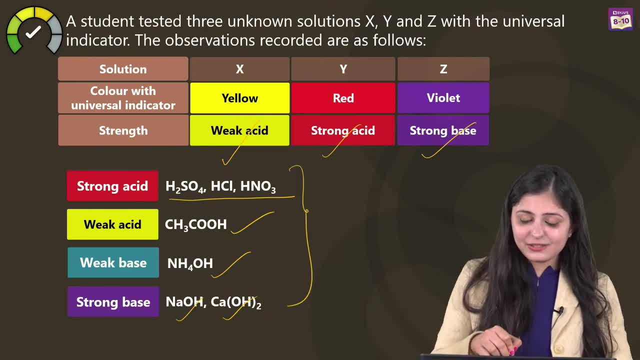 Calcium hydroxide as the strong basis, isn't it? We've just categorized the options only. 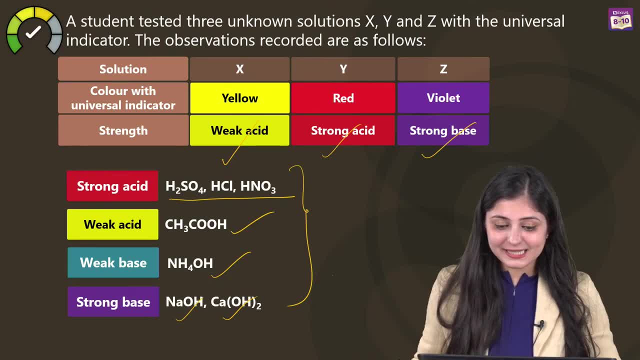 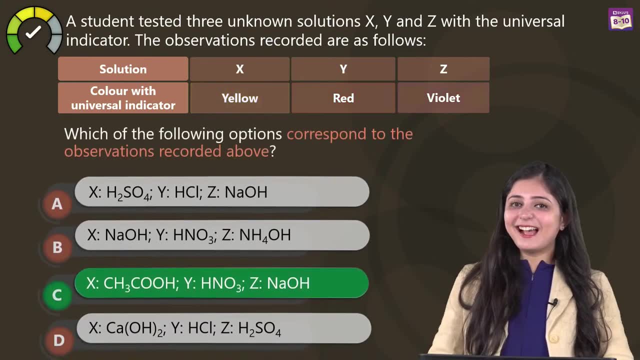 Alright, Harry says C, Shailaja says C, Rami says C, Nikesh says C and that is the right answer. You people are very much correct, C is your right answer. 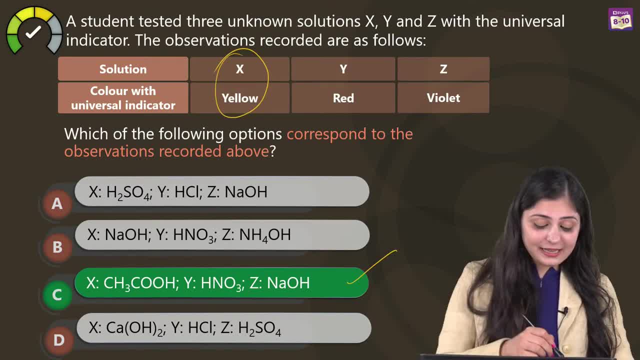 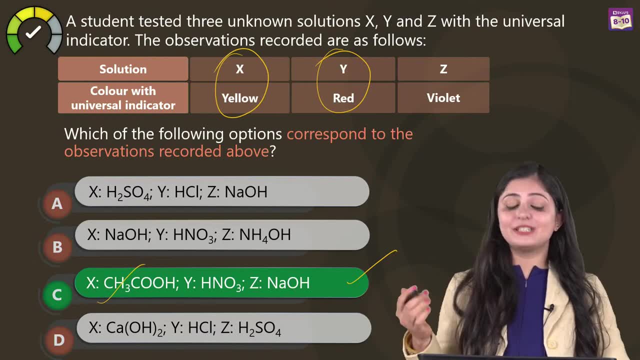 X, aapka yellow show kar hai, that means it's going to be a weak acid, like acetic acid. Y is showing red color, red, which means it's going to be a very strong acid, like nitric acid. 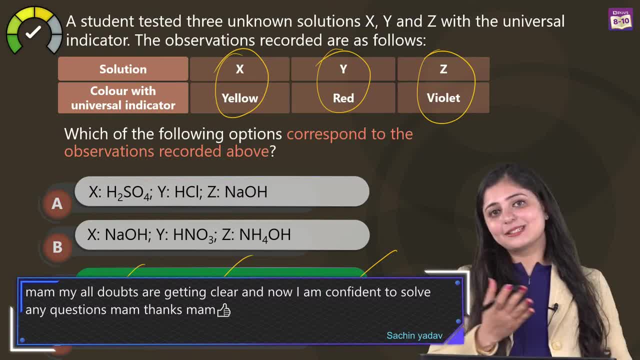 And Z is showing violet color, which means it's towards the basic side and that to a strong base, so sodium hydroxide. 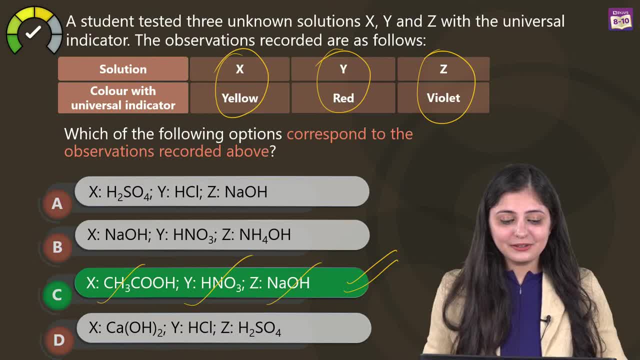 So, you people have guessed the answer absolutely right. Pat said C, Haripriya also said C, Abhilashini said C, Priya said C, Vani said C, great. Some of you also said C, great, great, great. Shweta has also written C is the right option. Shakshi said C, Umama, you're welcome. Alright, Devu, just read the question again, go back and just read the question. You would definitely arrive at the right answer, I'm pretty sure. Alright, now, moving on to the next question. 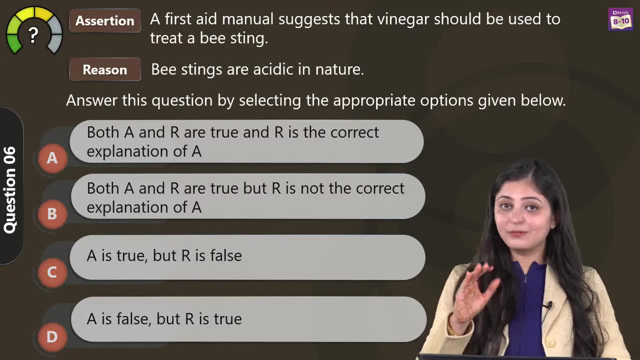 Now, Assamesee said, Assertion reason type of questions, I know you people want to practice a lot. 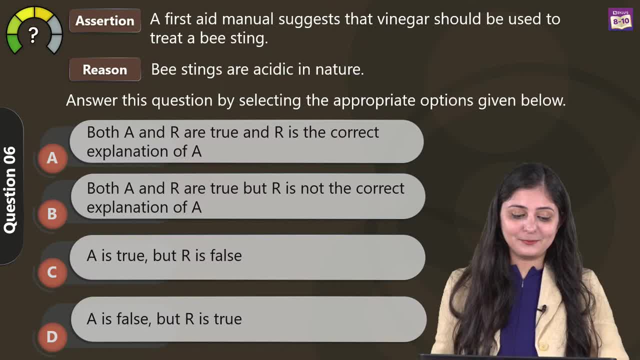 So, there you go, we've got an assertion reason kind of a question for you people. But, you're going to attempt it. 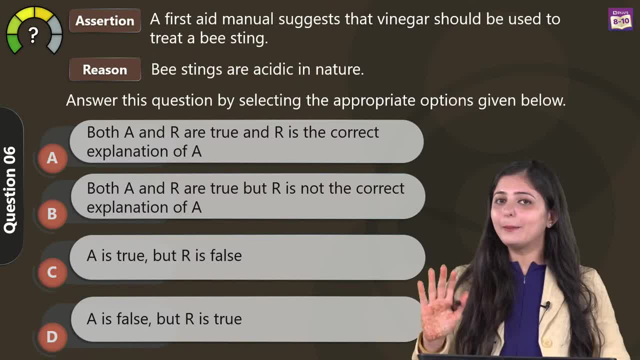 We have attempted a lot of assertion reason kind of questions now. So, now, you shouldn't be scared, what's this? Now, you should be like, give me the assertion reason type of questions and we're going to solve it. 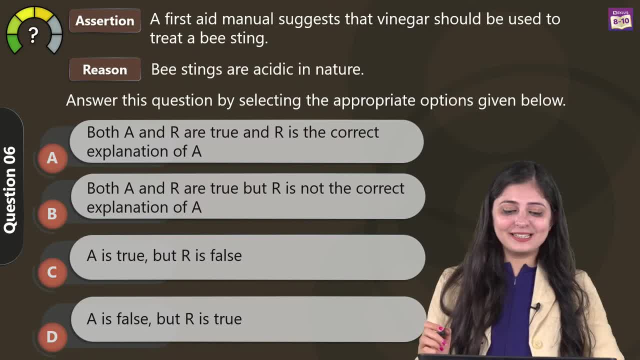 I hope you people are having that kind of confidence. Come on, let's start. 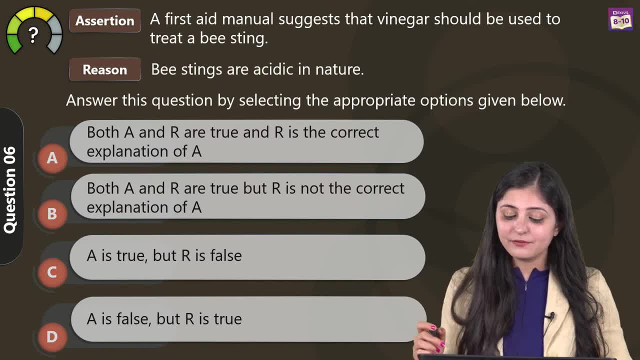 Assertion statement over here is, First aid manual suggests that vinegar should be used to treat a bee sting. 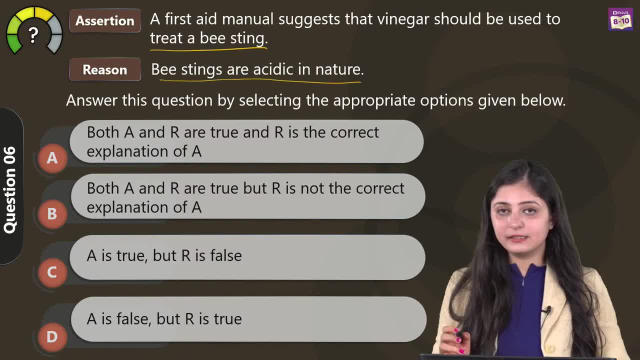 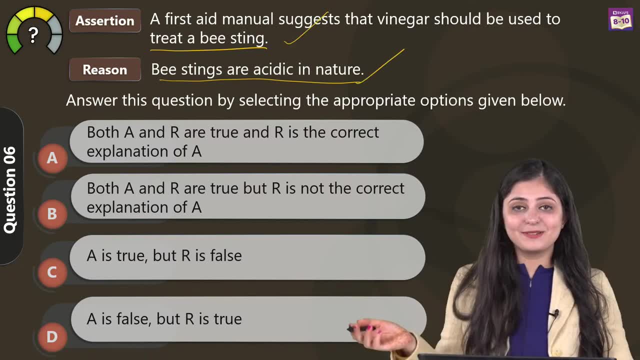 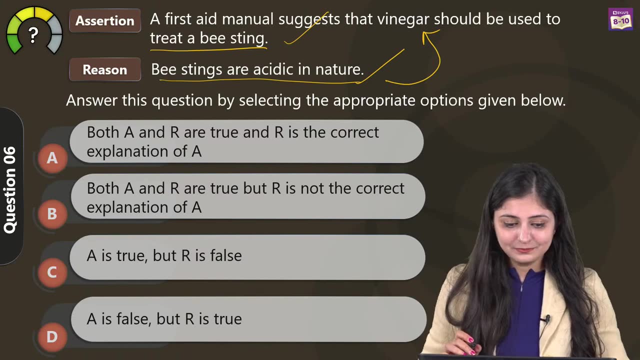 And the reason they've given for this is bee stings are acidic in nature. What you have to do, you have to see whether this statement is true or false. Then, whether this statement is true or false. And if this reason is true, is it the correct explanation for assertion or not? 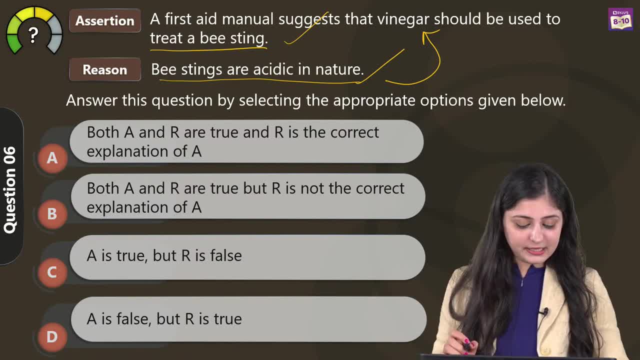 Sakina says, sixth answer is D, A is false but R is true. Phenyl also says D. Omama says D. 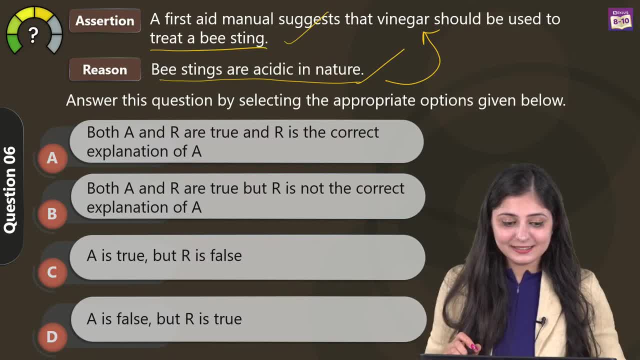 Nisha says D. Aditya says D. Paat says D. Shweta says D. Arun says D. Everybody is saying D. Sadhan says D. Alright. Sachin says B. 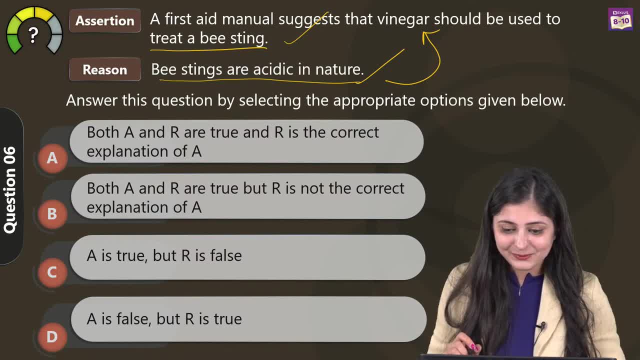 Both A and R are true but R is not the correct explanation. Okay. 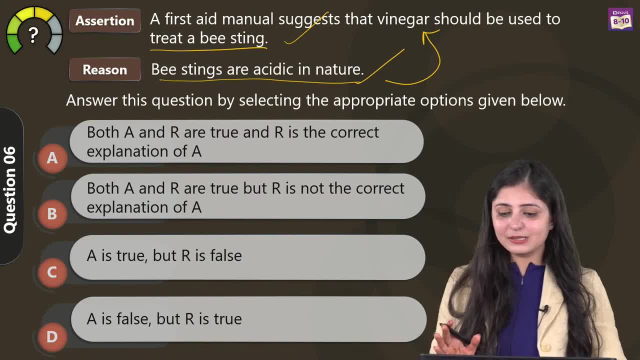 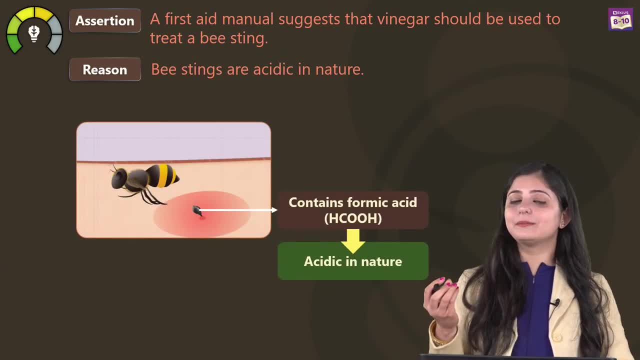 So, mostly you people are saying D but I can see B also in the chat box. Let's see. Now, unfortunately bee sting has happened. And what happens in bee sting? Formic acid is present which is acidic in nature. Acid is formic acid or methanoic acid. Now, bee stings are acidic in nature. 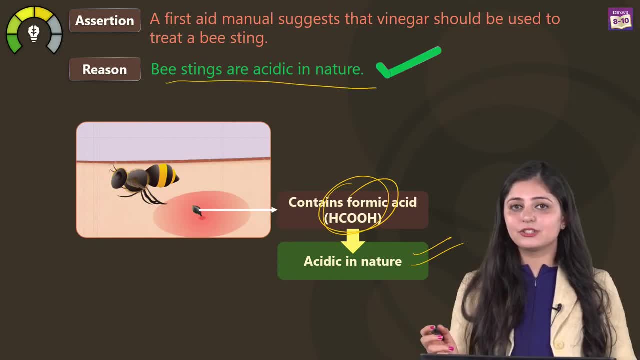 This is very much true. So, this statement bee stings are acidic in nature. Our reason is absolutely true. 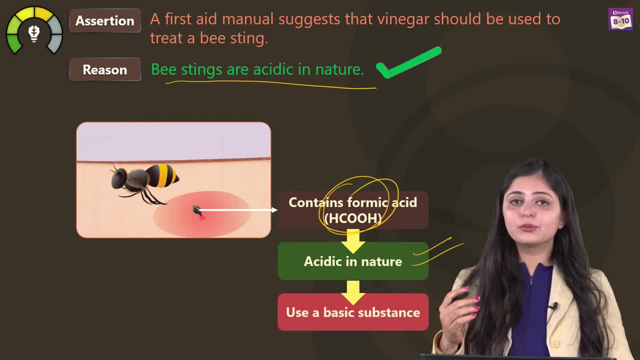 Now, if you want to neutralize this. If you want to cure the person. If you want to provide a remedy. You would definitely use a basic substance. So that it nullifies the effect of the acid. It neutralizes the effect of the acid. 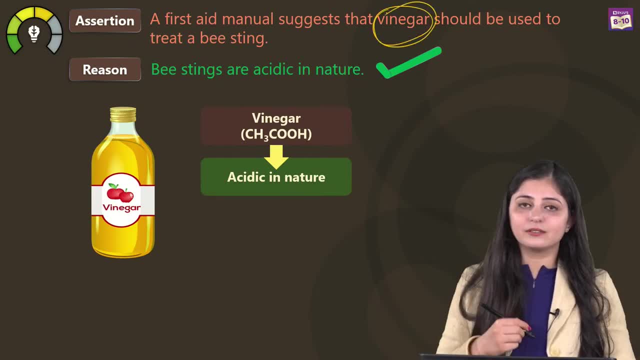 Now, the substance they have given us is vinegar. And we all know that vinegar contains acidic acid. If it contains acid. 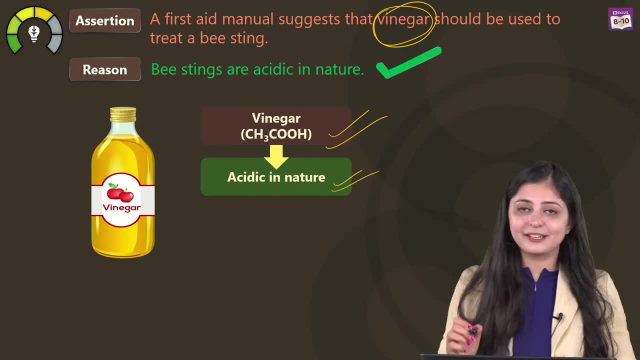 What is its nature? Its nature is acidic. Isn't it? 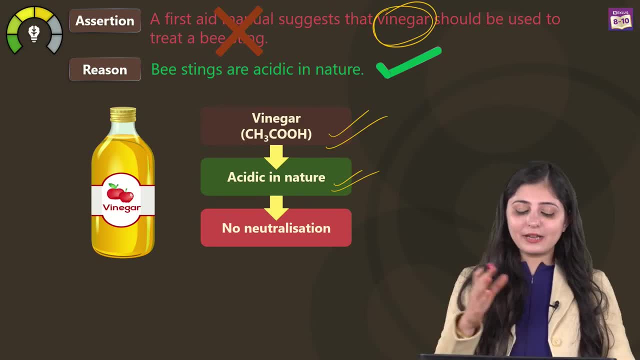 If there is excess acid and you are going to add more acid. No neutralization is going to take place. We need a base for this. Isn't it? Base is not given. Acid is given. 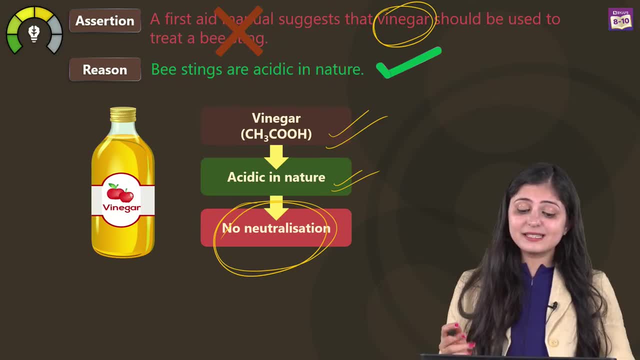 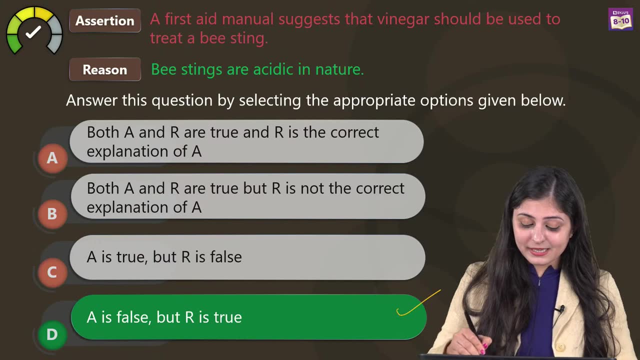 Which means that this assertion that they have given us vinegar. Is somewhere not fitting in. And that brings us to the answer that A. That is your assertion is false. But your reason is true. This statement that they have given you is false. 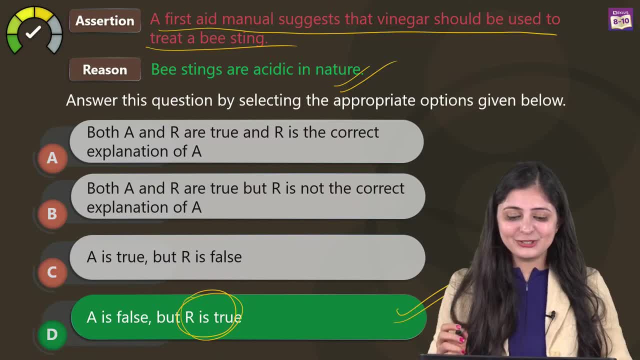 But this reason is very much true. Shweta said D. 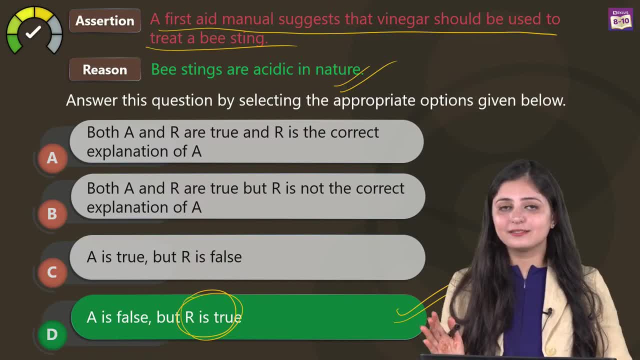 Harry says use baking soda instead. Absolutely right. Use baking soda. 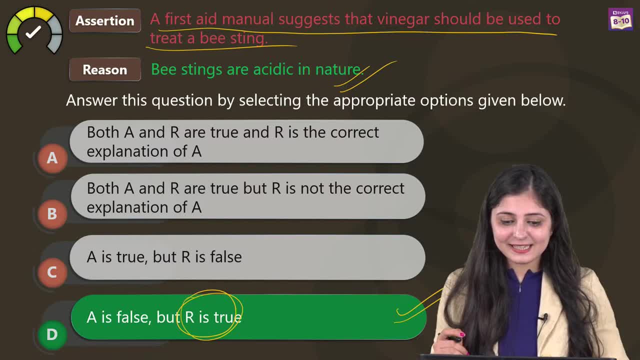 Why acidic acid? Priyanshi says base must be used. Absolutely right. I told you the last time. 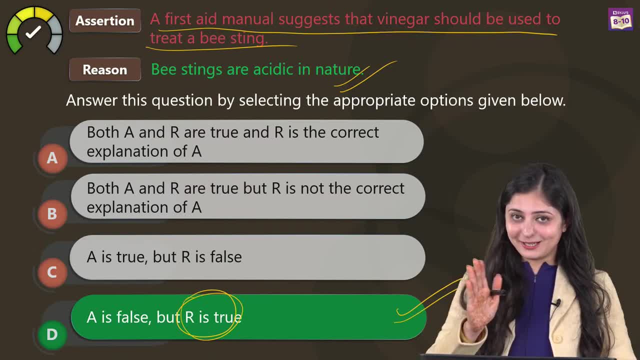 If you use acid in acid. So that's not going to be the remedy. That's going to be the comedy. Right? 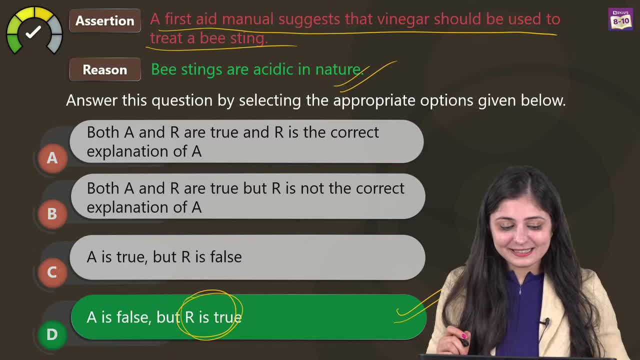 And we don't want that to happen. Alright. Shweta said D. Great. Great. Great. 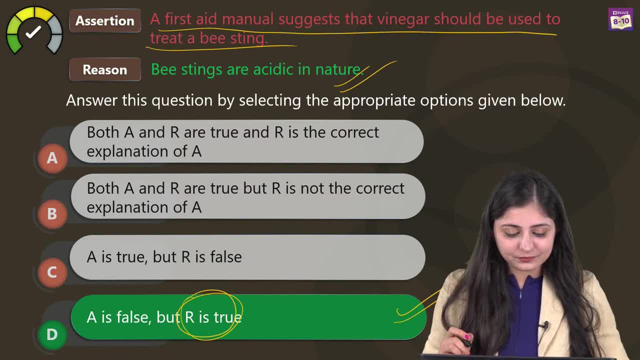 Deepak is saying C. A is true. No Deepak. A is not true. 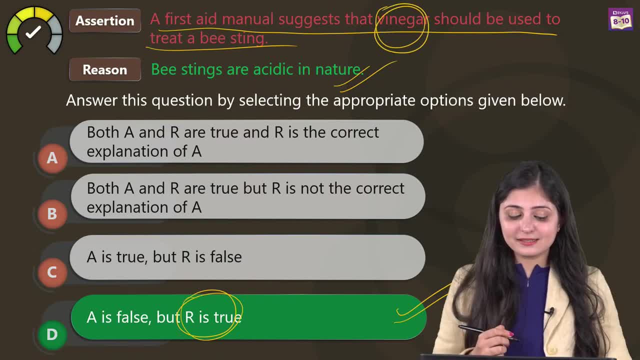 Because vinegar is an acidic substance. How can it cure an acidic situation. Wherein the acid is already in excess. Deepu says weak base use. Alright. Kamal you are absolutely right. Manoj you are absolutely right. 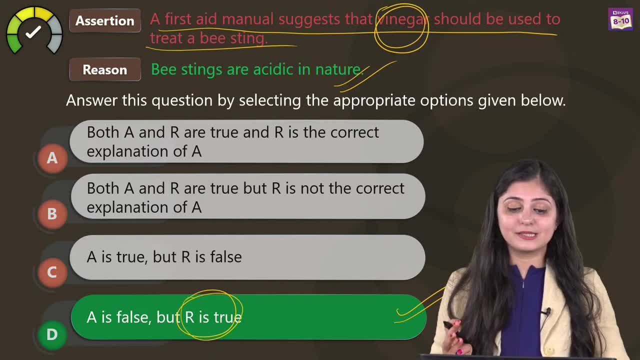 Sameeksha says sodium bicarbonate must be used. Yes. Sameeksha you are absolutely correct. 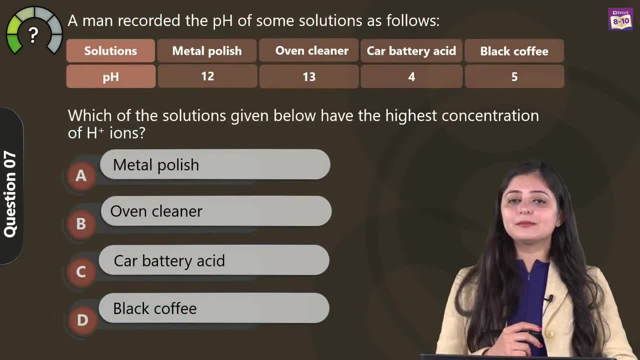 Now moving on to the next question. Question number 7. 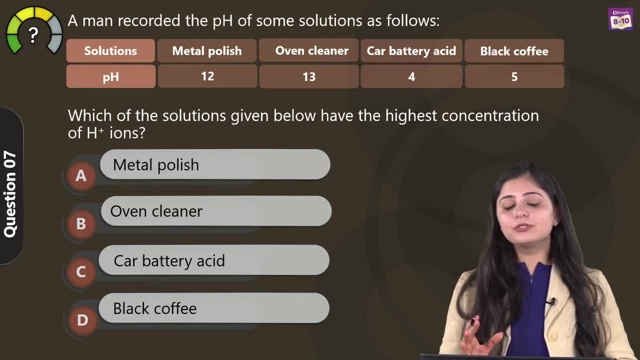 A man recorded the pH of some solutions as follows. 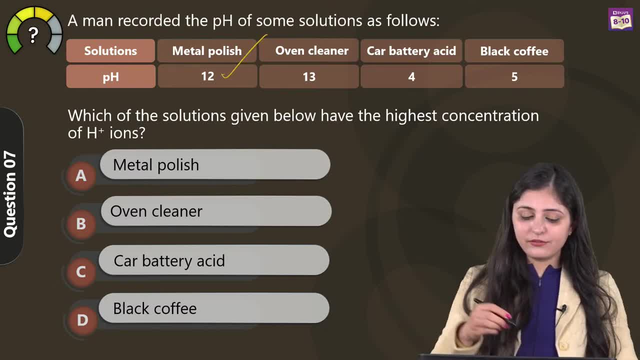 So you've got metal polish with a pH 12. You've got oven cleaner with a pH 13. 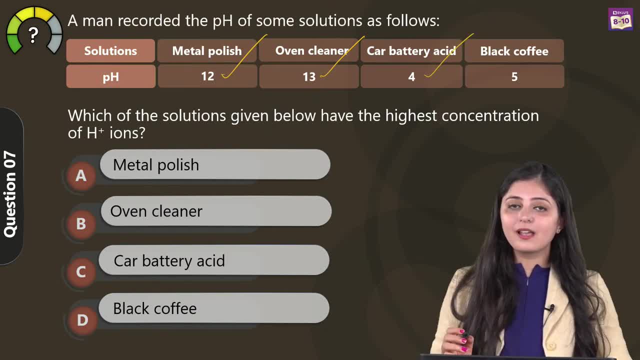 Carb battery acid with pH 4. And for all fitness freaks we've got black coffee with pH 5. 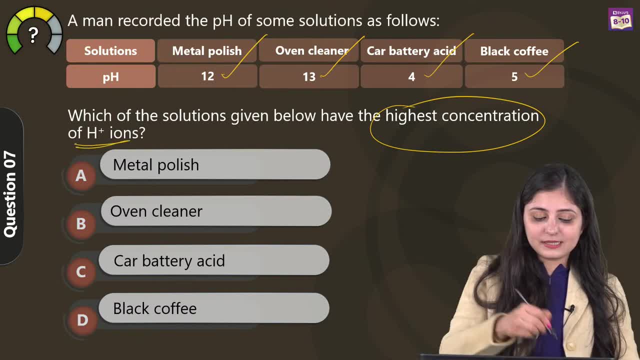 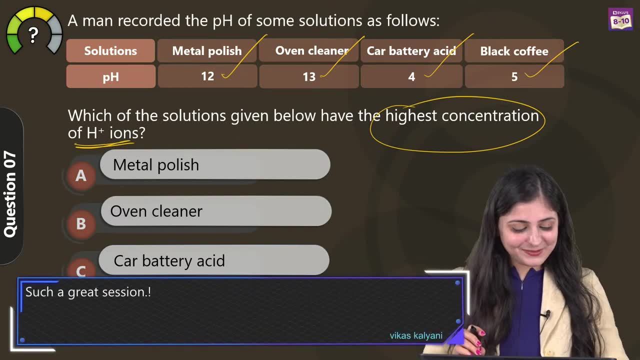 Which will have highest concentration of H plus iron. We've just solved a question like this. Come on tell me. What is the correct answer. Question number 7. 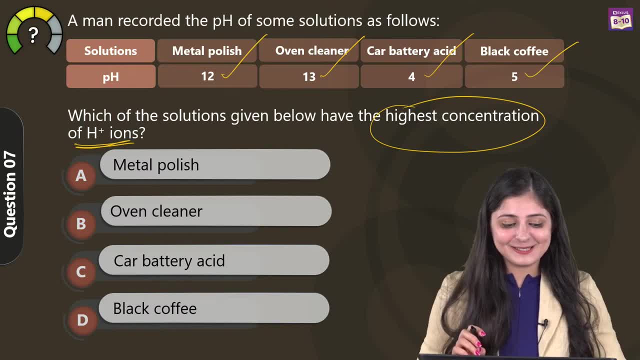 Ayush says C. Umama says C. Seema says C. 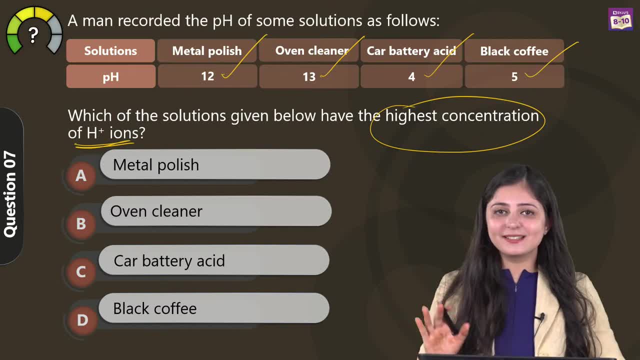 When same unanimous answers come. I feel very happy that you people have revised the topic very well. And I am pretty confident. That you people are going to give very good exams. 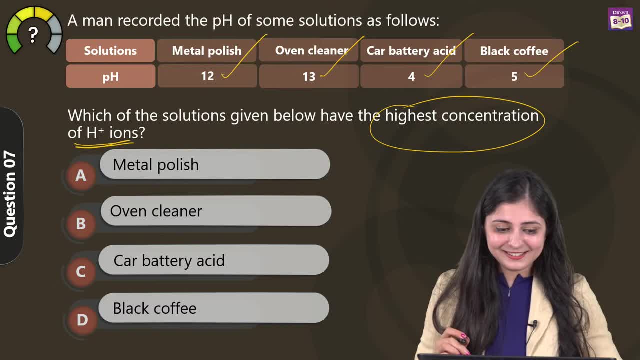 I can see everybody has written C. Good. That's how the class should go about. Study well. 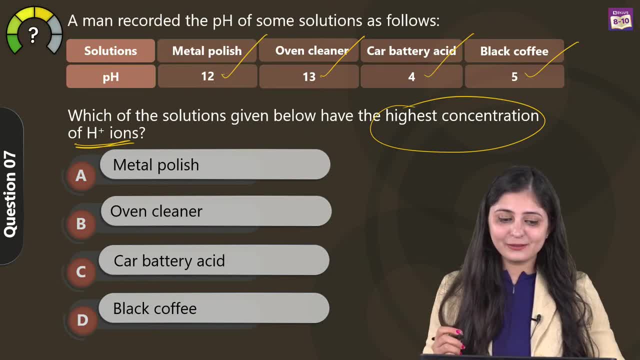 And then here we can have a very good revision. Of whatever you've studied. 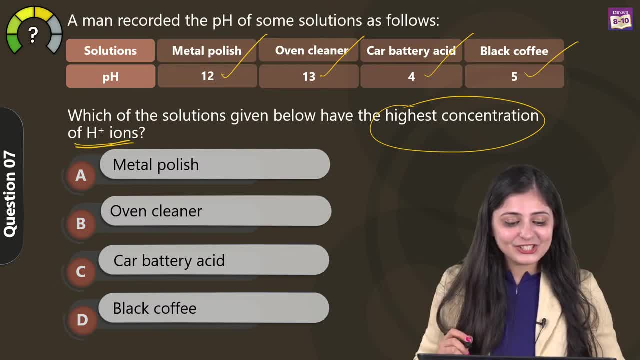 Hari Priya says C. Fennel says C. Satam, Nikesh, Abhilashini, Ritisha, Shahinita. Everybody has said C. You've all become pro in chemistry. 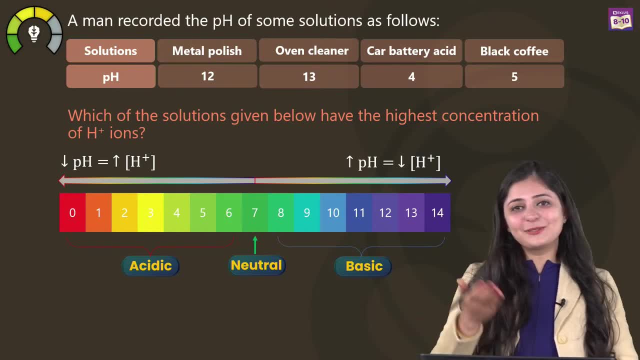 Alright. Now. Quickly I'll just tell you what the answer is. 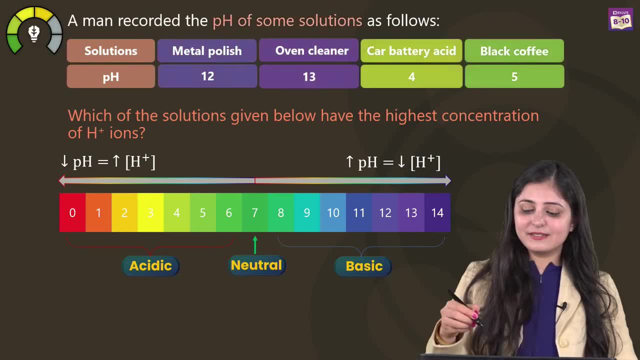 You people know it already. Now they have given us 12 and 13. 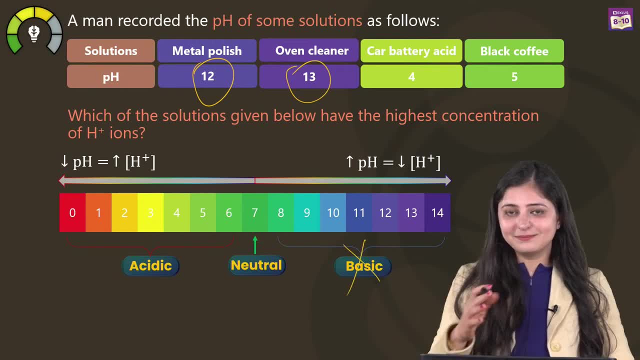 This is the basis. So obviously there is basic substance. H plus iron concentration will be less. Out of 4 and 5. 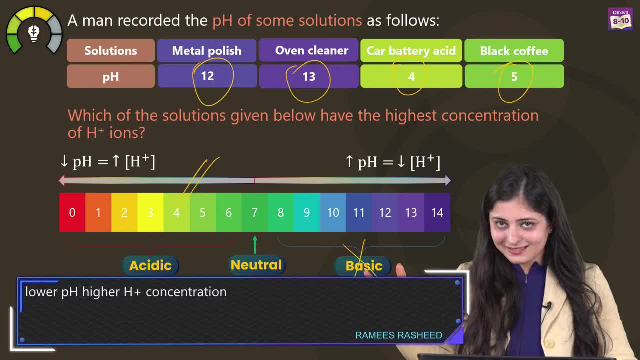 pH 4 is towards the left side. More left side. More acidic. 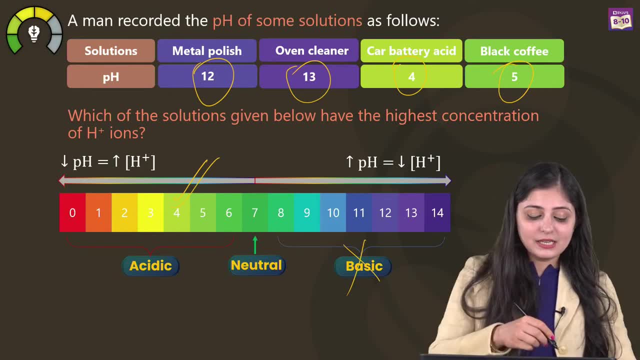 H plus iron concentration would be more in this case as compared to this. Because as the hydrogen ion concentration increases. What happens to pH? pH goes on decreasing. 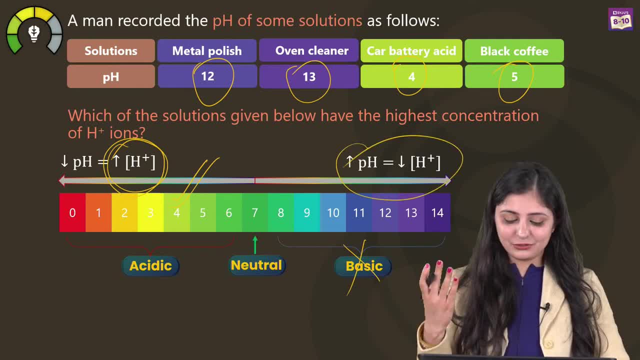 Plus vice versa is also true. As the hydrogen ion concentration decreases. pH also increases. 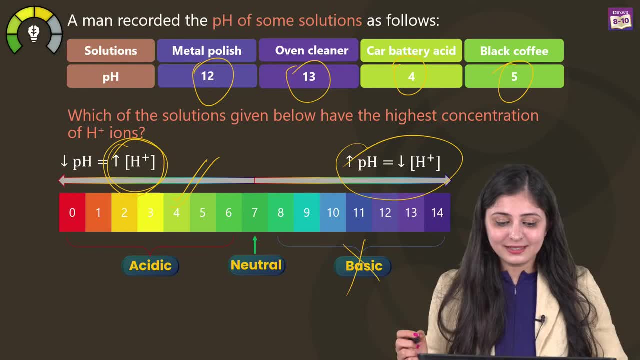 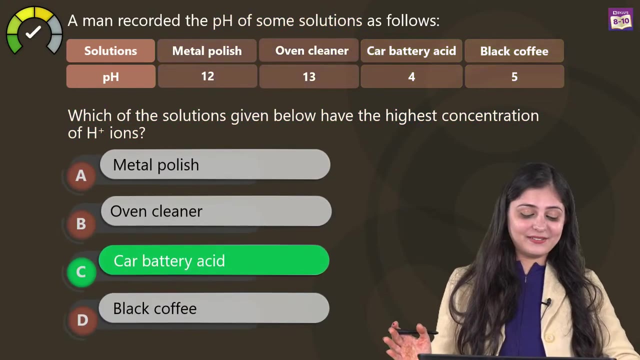 Manoj you are absolutely right. Good. I like it when you people give the explanation also in the chat box. I mean I can understand. You are not cheating. I can understand you people. Great. So with this we've arrived at the correct answer. That car battery acid with the lowest pH amongst these is going to have the highest concentration of H plus ions. Alright. Now. 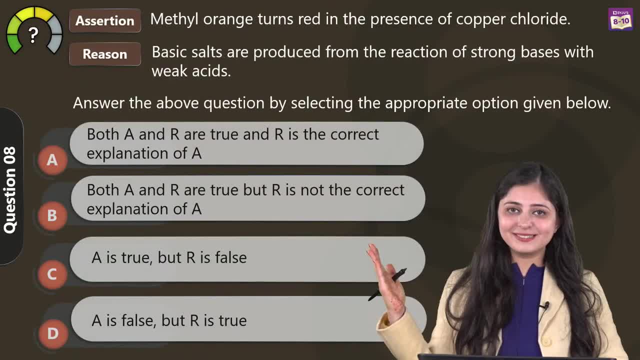 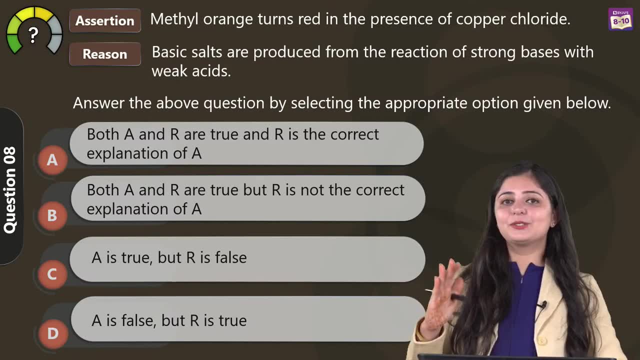 Moving on to question number 8. Again here we are with assertion reason kind of a question. So question number 8. Put a dash and let me know the answer. Meanwhile I am just reading the question for you people. Alright. 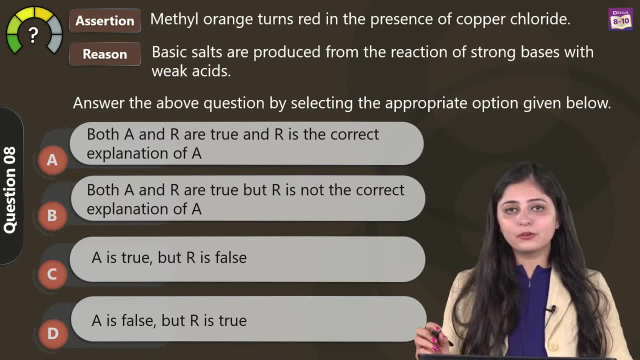 Assertion says that methyl orange turns red in the presence of copper chloride. Copper chloride ke saad methyl orange turns red. Is what the assertion is saying. 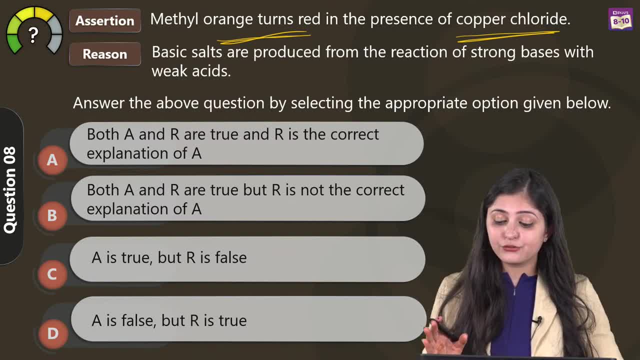 Reason mein statement likhai basic salts are produced from the reaction of strong bases with weak acids. Question number 8. 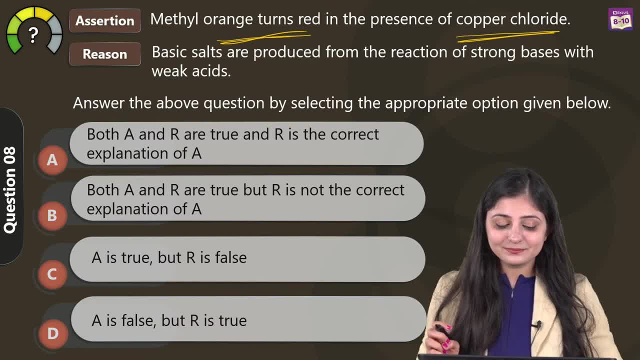 Let's see who answers this first. Yes we are done with question number 7. And you people are right. D was the correct option. Now. 8th. 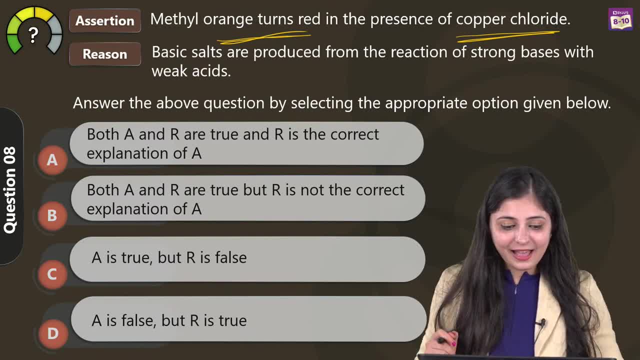 Come on let's see who is going to answer this first. And we've got Rohini who has answered it first. Rohini says I don't know if it's right or wrong. We'll get to know that. But she is saying B is the right answer. Ritesha says B. Satna says B. Mayank has given the explanation also. Okay. 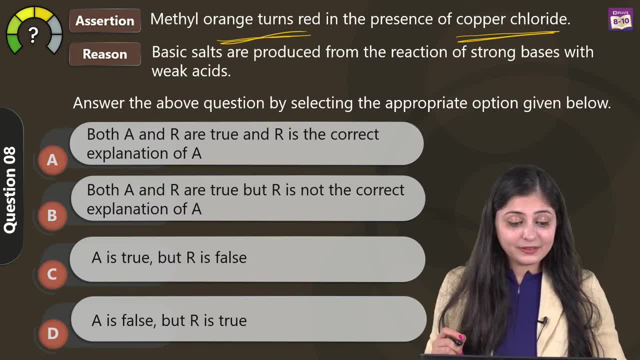 Akshat says B. Praveer Tekno says B. Divu says B. Ritesha says B. Chirag and Tarun says A. Priya says D. Alright. 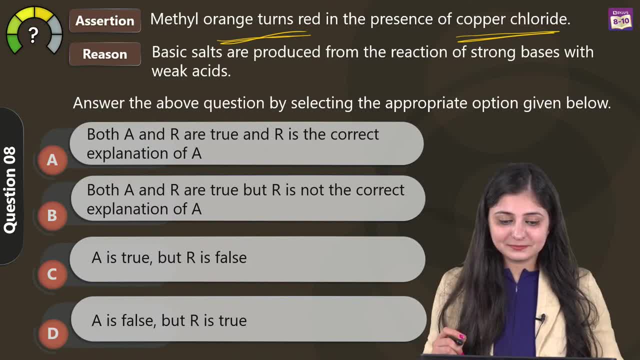 C is left. Rest A, B, D everything is written. 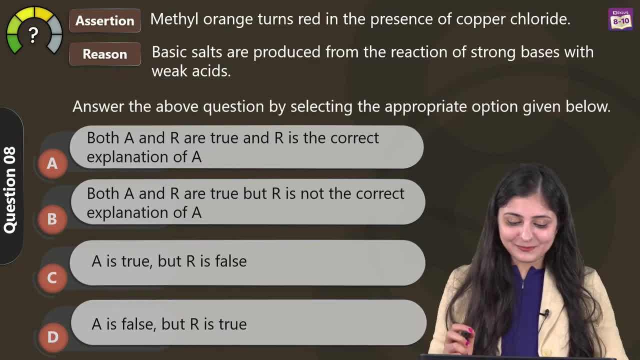 But I can see one answer is very common. So let's discuss. Now. In general we all know. 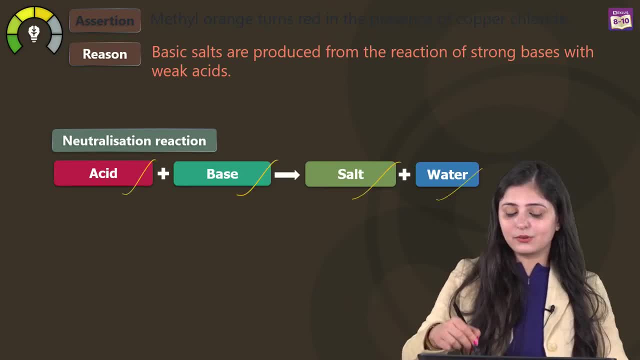 Acid plus base gives you salt plus water. Class 7 say we've been studying this. And I told you that salts are not always neutral. It depends on the acid and the base that is present. 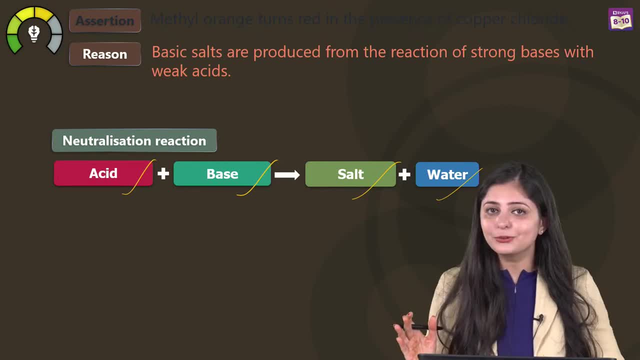 So you have to come out of that bubble that salt is always neutral. That's not true. 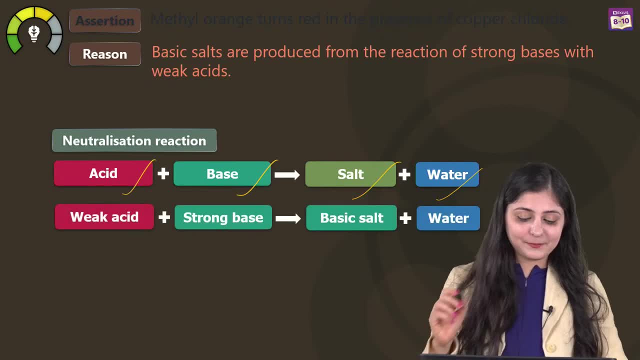 Now we know that salt can be acidic and basic also. If we have weak acid. And if we have strong base. Whatever is strong. Salt is on its side. So strong base would give us a basic salt. 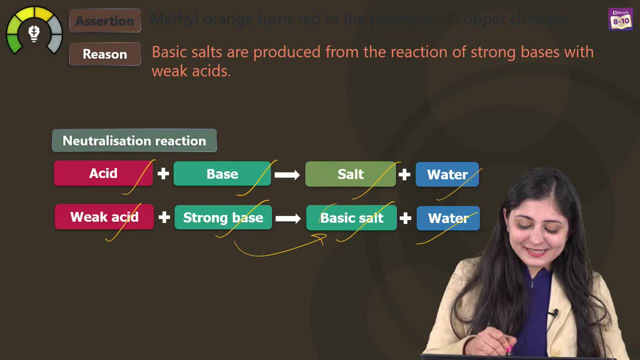 Plus water comes from free funds. So basic salt is being formed in this case. And that is very much what is being given in the reason. Isn't it? 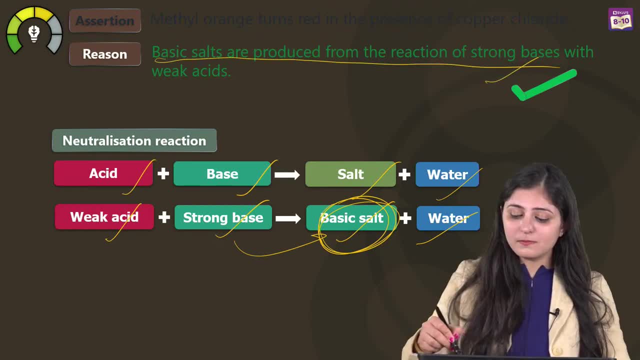 Basic salts are produced from the reaction of strong bases with weak acids. 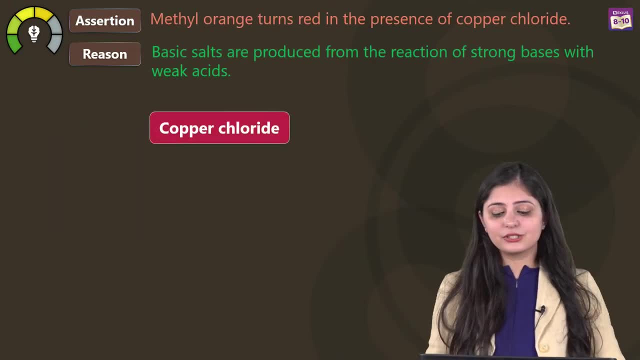 Absolutely correct. Now. Coming to the assertion statement. They have given us copper chloride. Now how is copper chloride made? 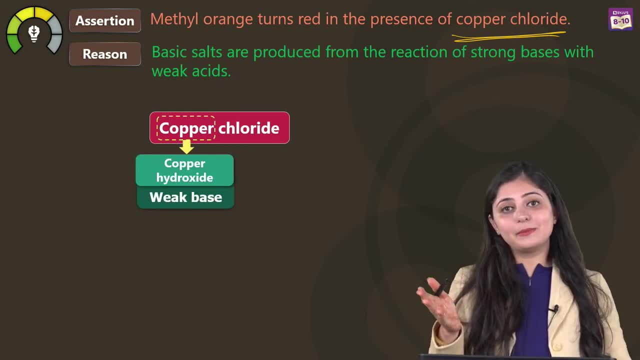 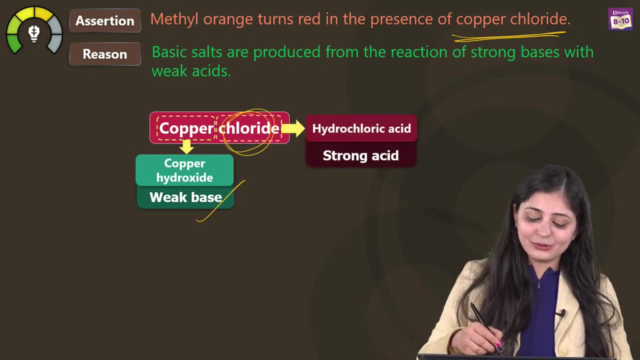 If we focus on copper. We'll know the base. Copper hydroxide which is a weak base. If we focus on chloride. We'll get the acid. Which is hydrochloric acid. And that is a strong acid. So now you know that this salt is being formed. 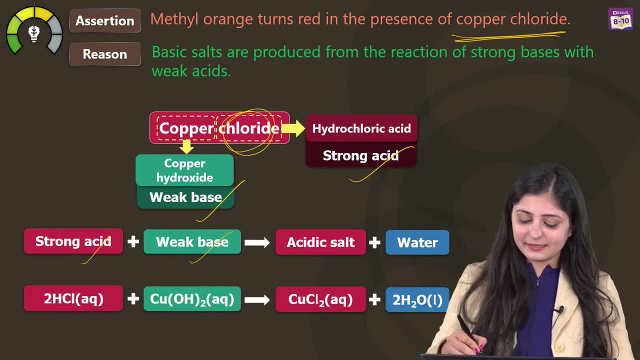 If we use a strong acid and a weak base. And this is the equation for the same. 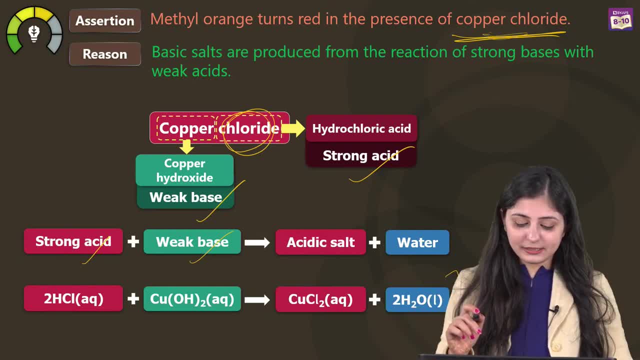 Now copper chloride. You have come to know. That it is an acidic salt. Right. What you need to do is. You need to figure out that. What color does methyl orange give in acidic solutions. That's all you need to do. 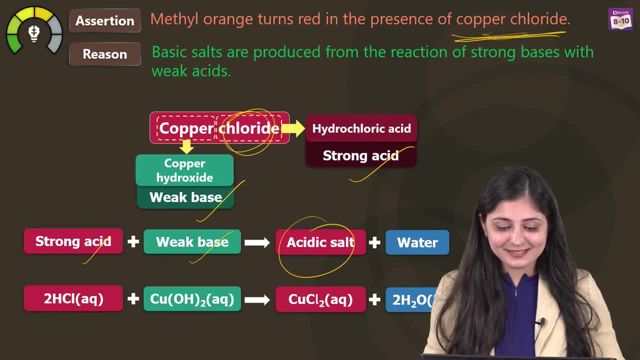 Music full on says B. Shalja says B. Mayank says B. Because reason should be. 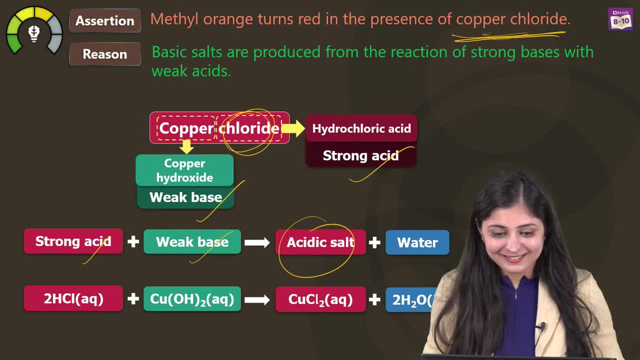 Methyl gives red color with acid. 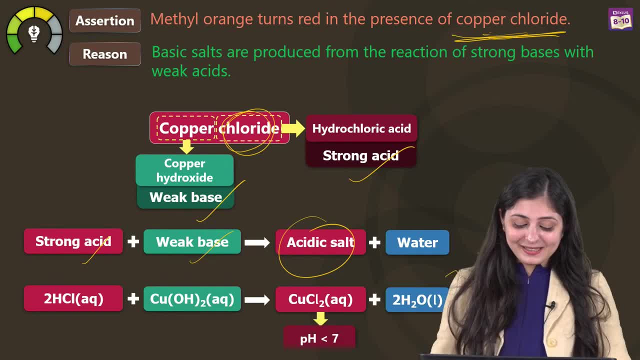 Alright. Okay. Now. If it is an acidic salt. The pH is definitely going to be less than 7. Now we know that copper chloride is an acidic salt. 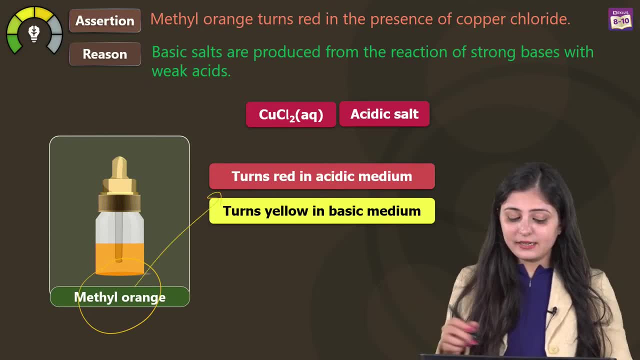 And this methyl orange. It turns red in acidic medium. And it turns yellow in basic medium. Go back to the statement given in assertion. They are saying methyl orange. Turns red in the presence of copper chloride. Very good. Absolutely correct. 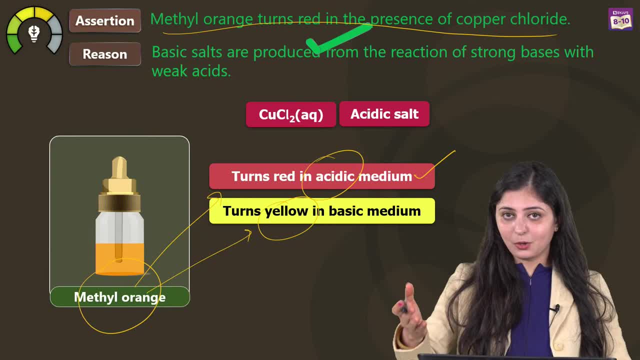 It turns red in acidic medium. That is your copper chloride. 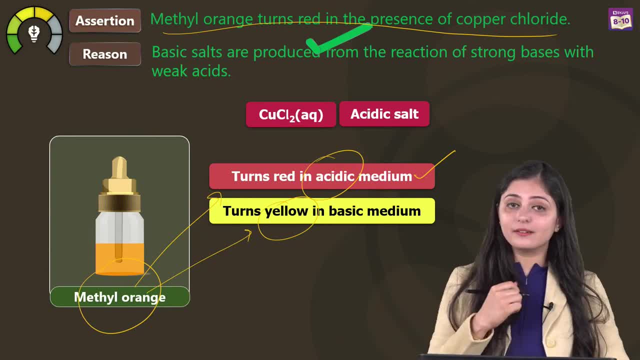 Copper chloride solution is very much acidic in nature. But in reason they are talking about basic salts. In assertion they are talking about acidic salt. How can that be the correct explanation. That is definitely not the correct explanation. 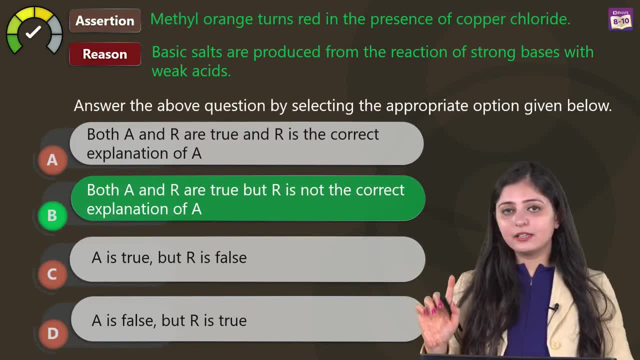 And this brings us to the answer. That both A and R are true. 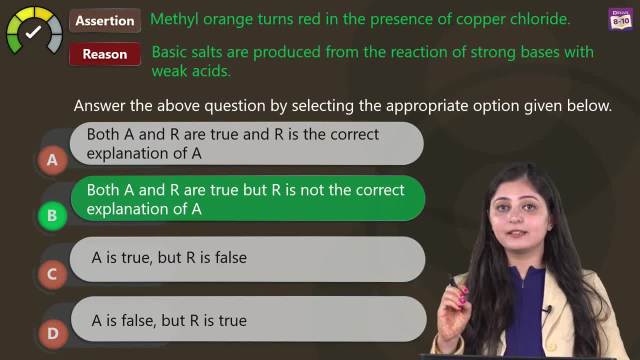 The statement given in assertion. The statement given in reason. 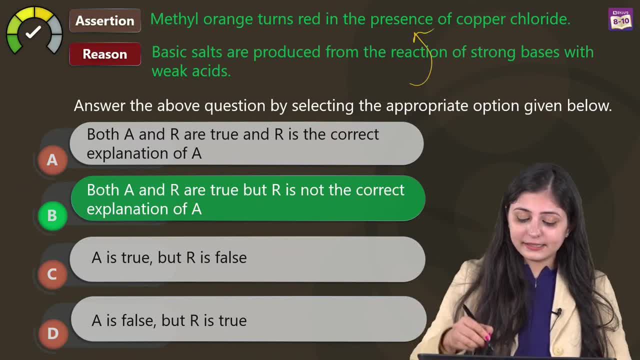 That is very much true. But it is not the correct explanation. 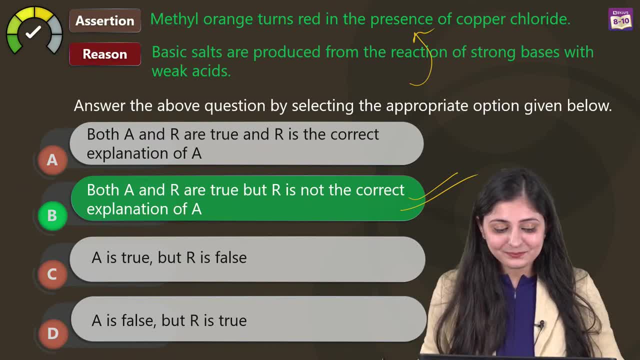 So this brings us to the answer B. Haripriya said B. Great. Shatakshi said B. Because R is not the correct explanation. Very good Shatakshi. Sainatha said B. Nikesh said B. All right. Yaseem said B. Abhilashini said B. Swathi said B. Rashid said B. Ashmita said B. Yes Nisha you are absolutely right. Nisha is saying they are not connected. Definitely not the correct explanation. 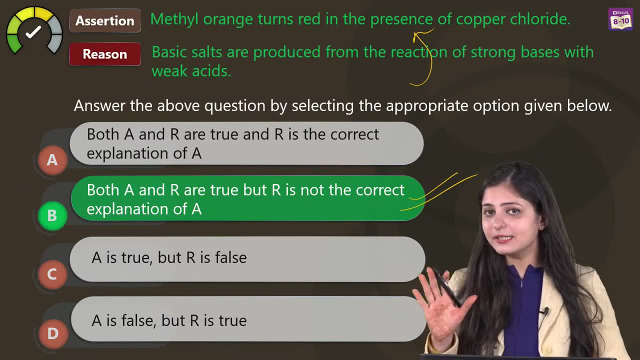 Now we have discussed assertion reason kind of questions. Wherein option A was also correct in any question. Option B. Option C. Option D. 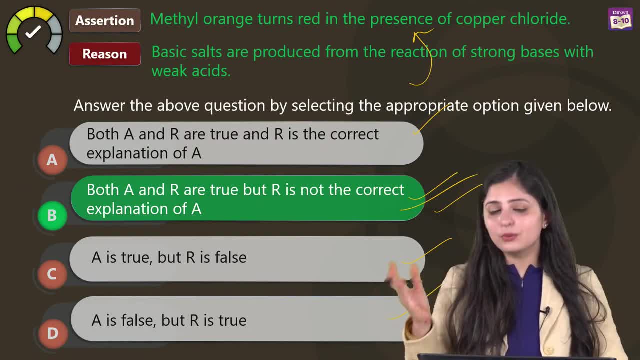 So you have got an idea that how all the options can be correct. What are the conditions. What are the situations. Now if any question comes in the exam. Any question of assertion reason. You should definitely attempt it and attempt it correctly. Can I expect that from you people. 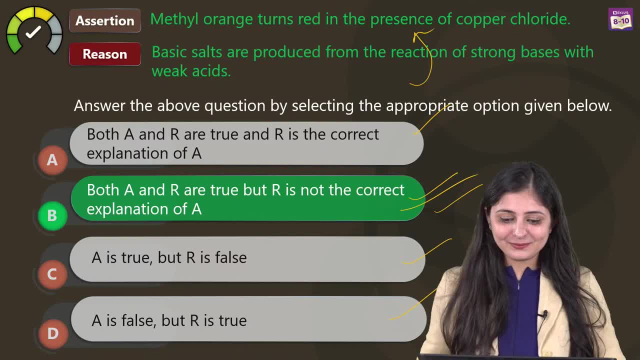 We have discussed all kinds of questions with you now. 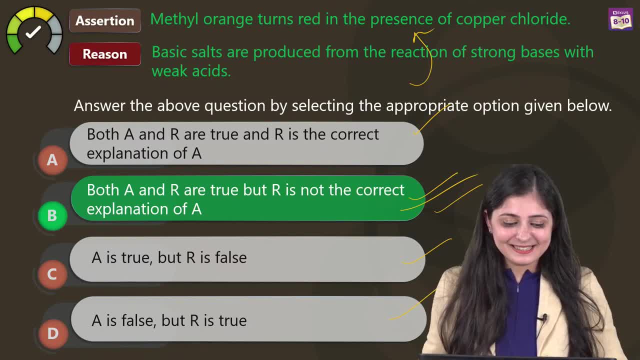 Yes. Pushpa says yes. Great. Great. Great. All right. 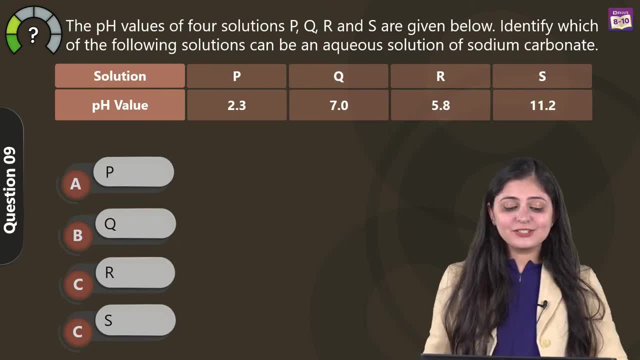 Moving on to question number 9. The pH values of 4 solutions P, Q, R and S are given below. 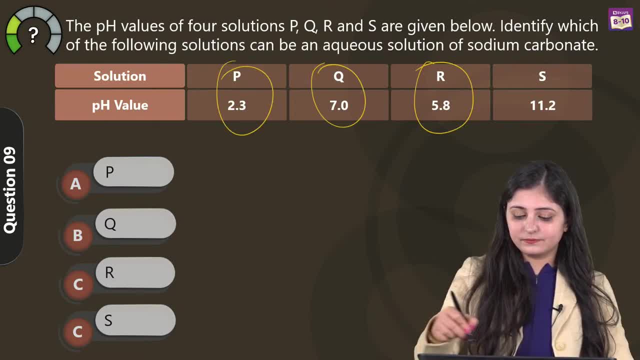 So they have given you these values. Identify which of the following solutions can be an aqueous solution of sodium carbonate. 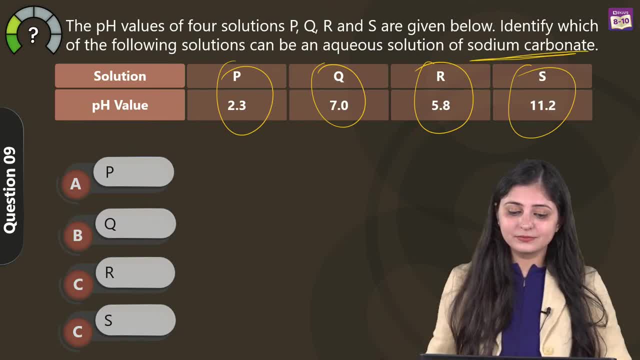 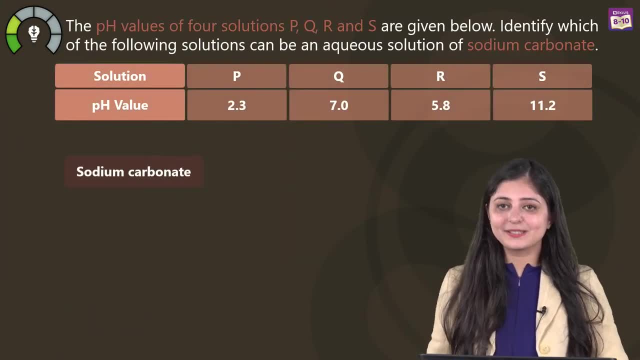 Sodium carbonate. That is your key word over here. That means you need to know about sodium carbonate. Isn't it? Now what exactly is sodium carbonate? It is Na2CO3. Sodium carbonate is being formed by sodium hydroxide base. 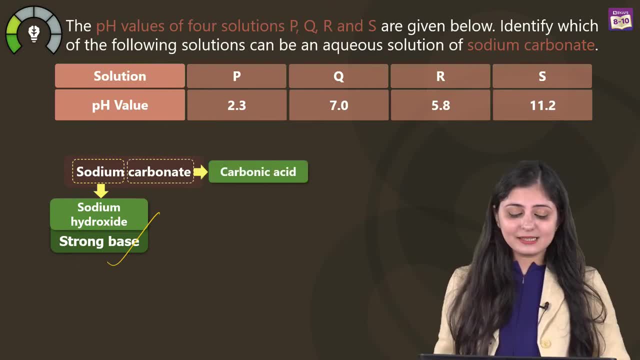 Which is a very strong base. And carbonates are called as acid. You are getting carbonic acid. Which is a weak acid. 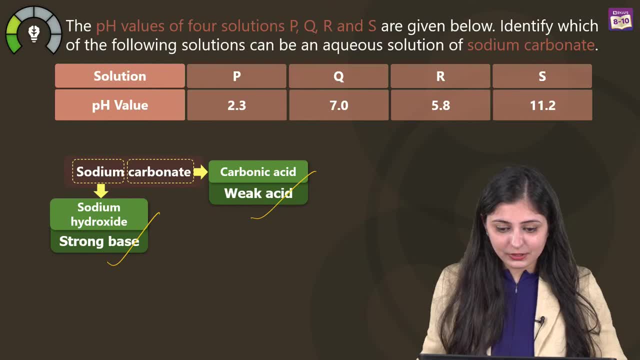 Shantha says 9th answer is D. Okay. Ananya said D. Praveet Techno Gaming says D. All right. Penel said D. Shetakshi said 11.2. Okay. 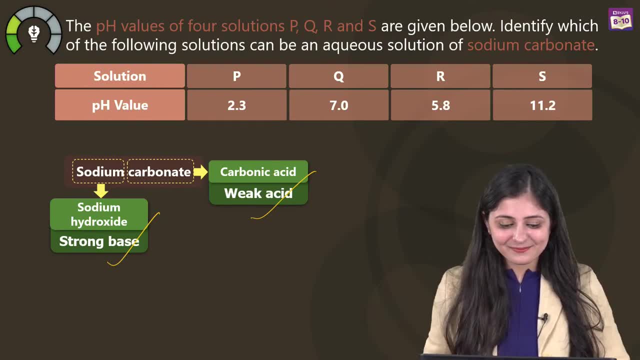 Let's see. Let's see what the right answer is. 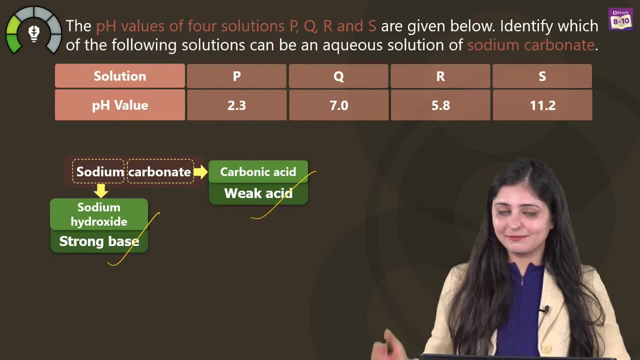 Nisha said the correct answer is S. Which means D option. All right. 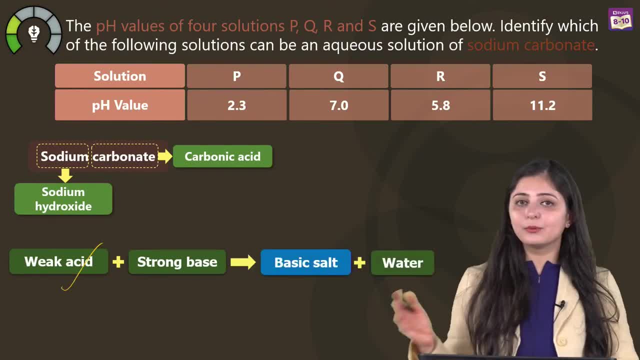 Now we have got a weak acid with us. That is your carbonic acid. 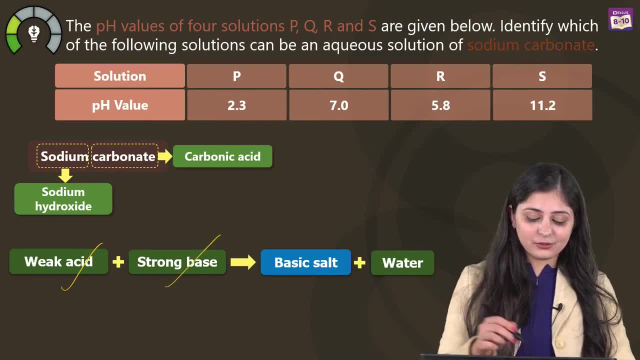 And we have got a very strong base. That is your sodium hydroxide. 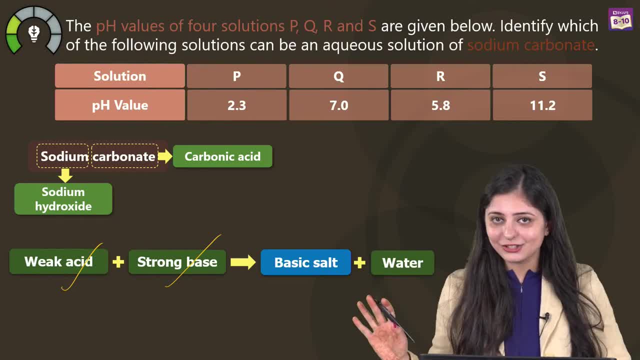 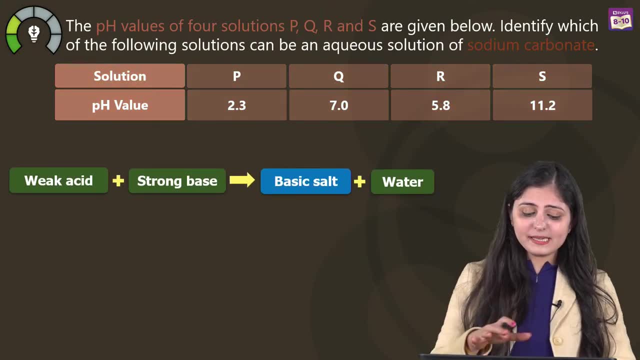 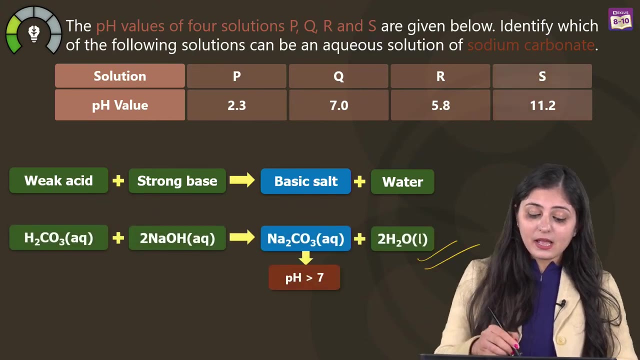 I told you jo bhi strong hoga salt ultimately usi nature ka banega. So it is going to be a basic salt that is being formed plus water. Now based on this can we judge the pH now? We can definitely judge the pH based on this equation. If it is a basic salt pH is going to be more than 7. 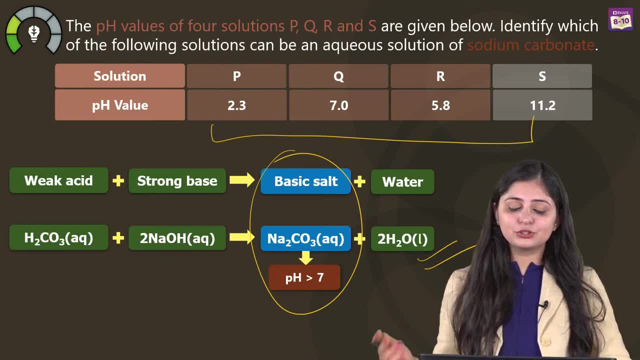 Out of these options. Ab to yeh bacho wala question ho gaya. 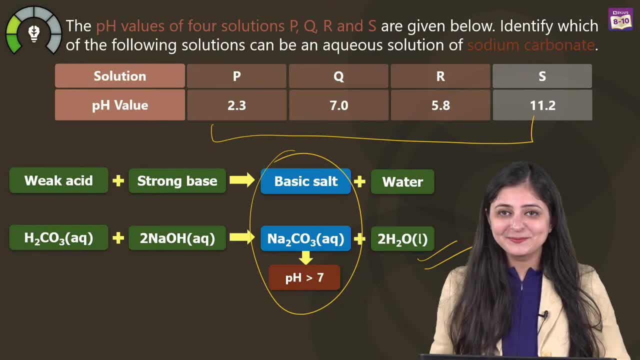 Ki 7 se upar wala number identify karke bata do. It is going to be option D. 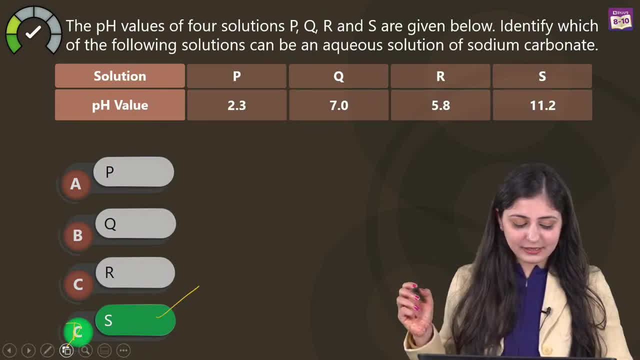 So option D is the correct option. Where in solution S that is having pH 11.2. 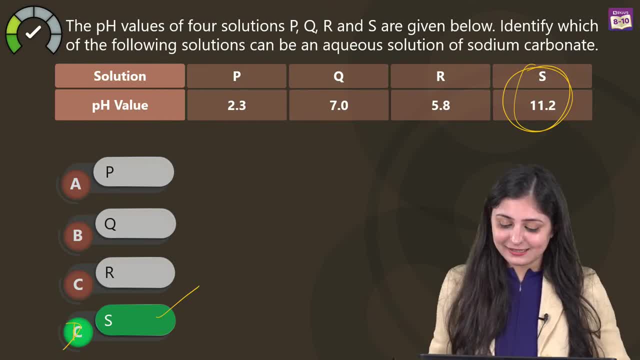 You people are absolutely right. Solution S is the correct answer. 11.2. Great. All of you got it right. 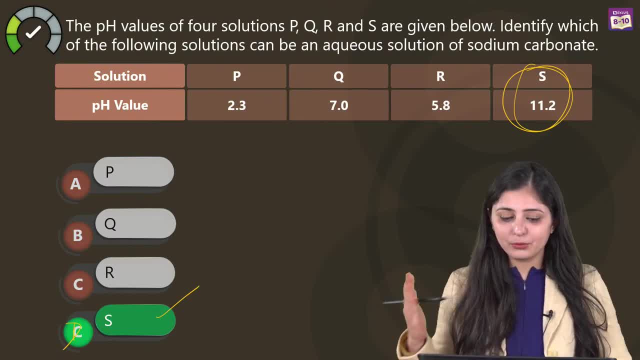 That means ab tumhe question kaise karna hai? Kya approach hai? Bohot acche se samajh a chuka hai. 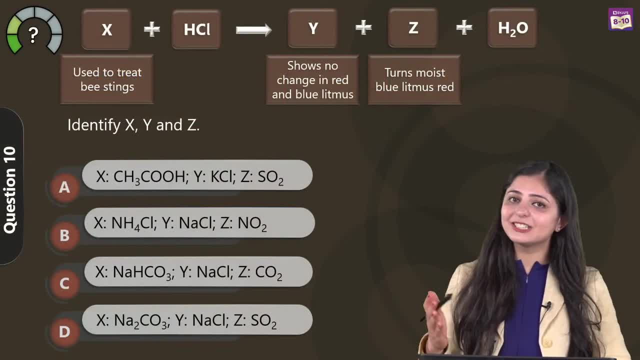 And pH based questions are very very easy ya. Bohot acche interesting questions hai yeh saare. All right. Moving on to question number 10. 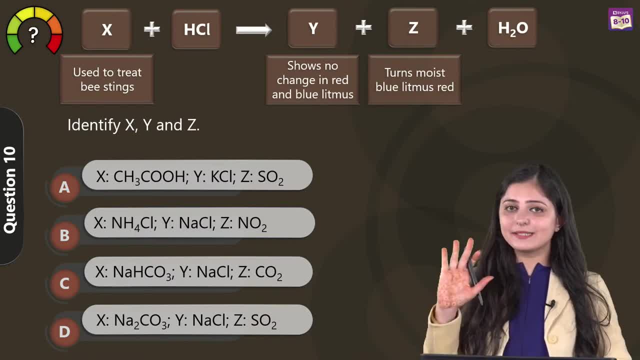 Let us get started now. There is some substance X that is being used to treat bee stings. Okay. 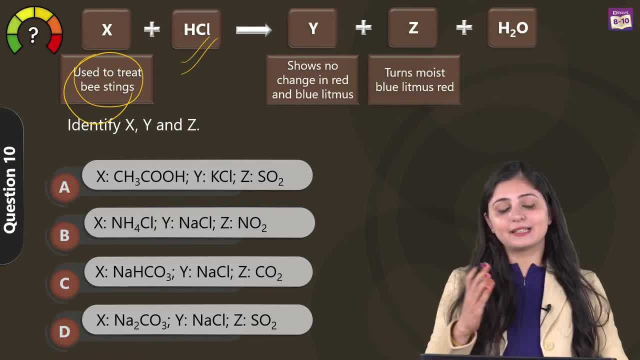 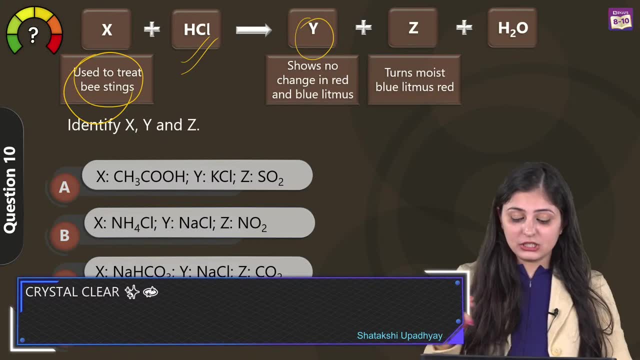 Then we have got HCL. So X is reacting with hydrochloric acid. It is giving you three products. Y which is not showing any change with red or blue litmus paper. 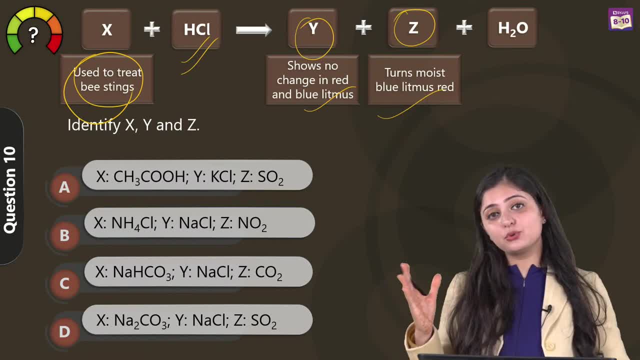 Z which is turning moist blue litmus into red. And water toh mostly har jaga aai jaata hai. 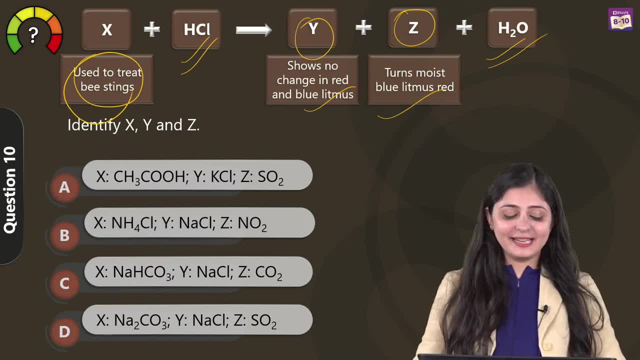 Come on tell me the answer. You have to identify X, Y and Z. 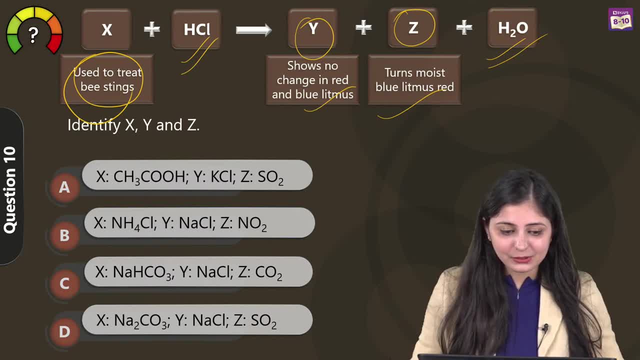 Palak says ma'am it is easy to solve with you. So do not miss any session palak. 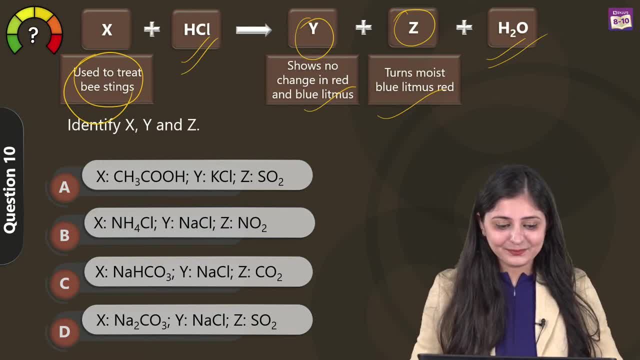 We will practice a lot. We will practice good questions here. All right. Question number 10. Put a dash. 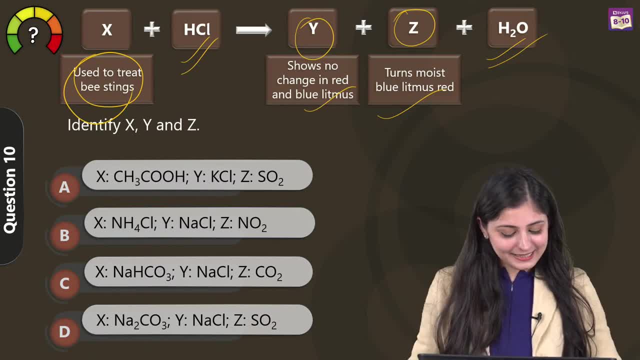 Give me the answers. Savarish says C is the correct answer. 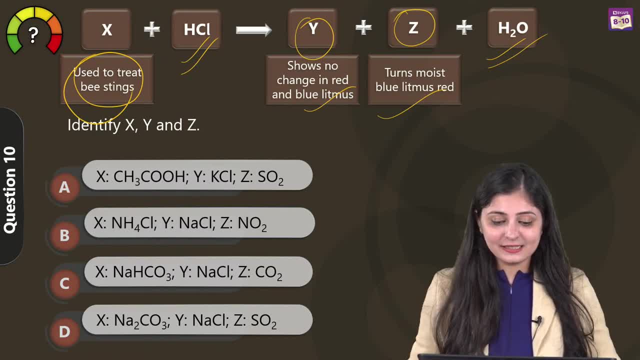 Okay. Anjana says C. Kashi says C. Ganpati says V. Ganpati, A, B, C, D me se bata do. Nikesh says C. Rishta says C. 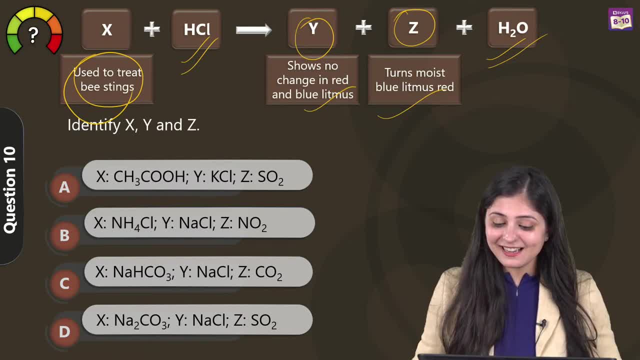 Yuvraj says C. Akriti says C. Sabina says C. Amisha says C. Great yaar. 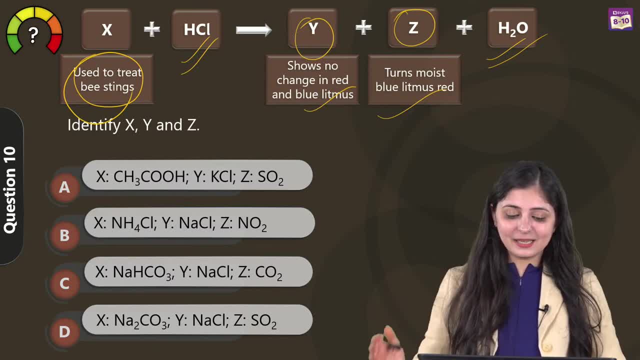 I think this topic is something that you people are very very confident about. Music full on has given explanation that D is the right answer. Okay. Music full on. See C and D again carefully. Om says C. Yasim says D. Okay. 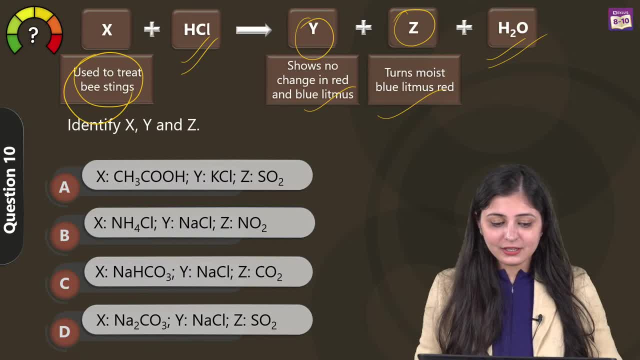 Prince says can you take lessons of light reflection. Physics sessions are already going on. Please watch those sessions every Tuesday. Yes. Great. 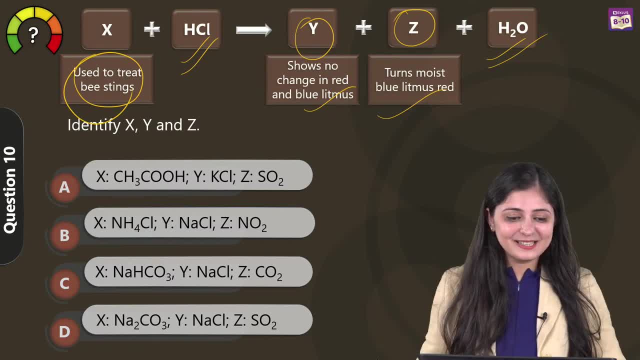 C, C, C. Varun says C. Rameez says C. Afifa says C. Priyanshi says C. Great yaar. 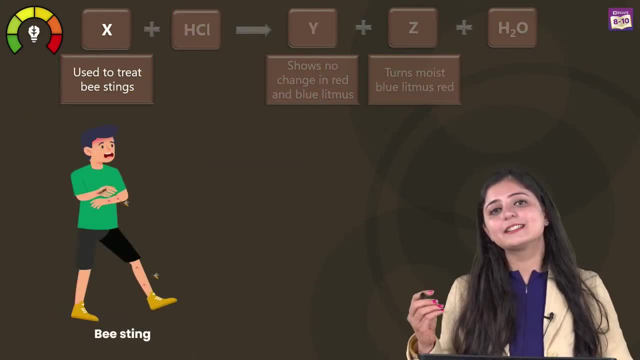 Now what is happening? Let us see this time. Unfortunately phir se B sting ho gaya. And ek jaga nahin. 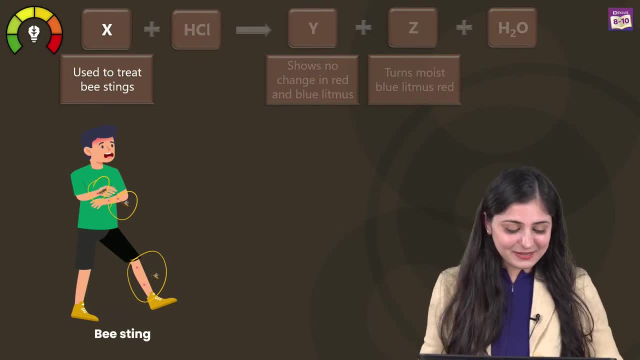 I think bahut zyada harmful way mein ho gaya. 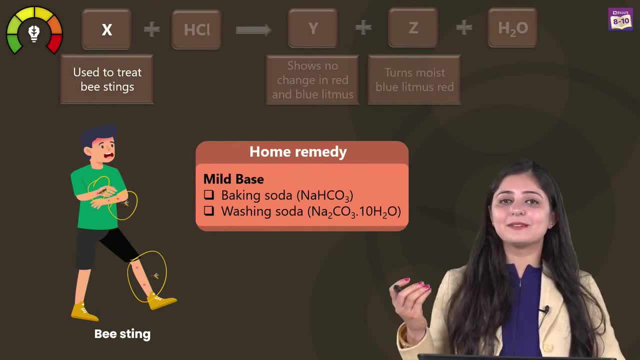 Now we just revised ki B sting mein formic acid is there. Right. 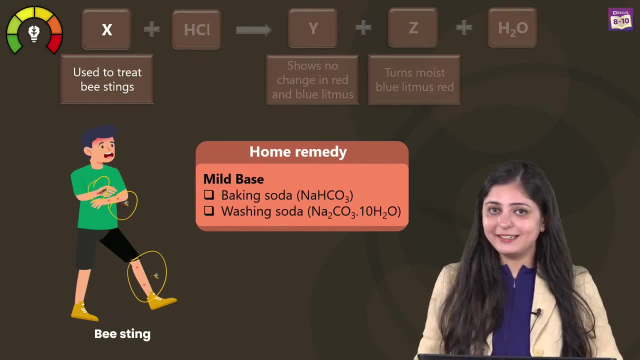 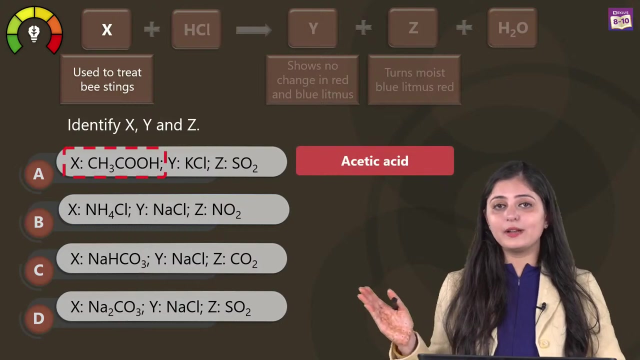 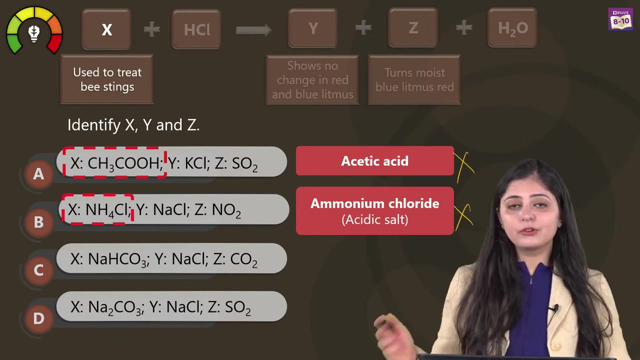 And if it is an acid to treat it to nullify its effect we need a base. We need a mild base which can be sodium hydrogen carbonate. That is your mild base that we can use as a remedy. Now in the options where they have given you acid like acetic acid in option A or some acetic salt in option B. They are going to be absolutely wrong. Yes. Shanita C is the right answer. 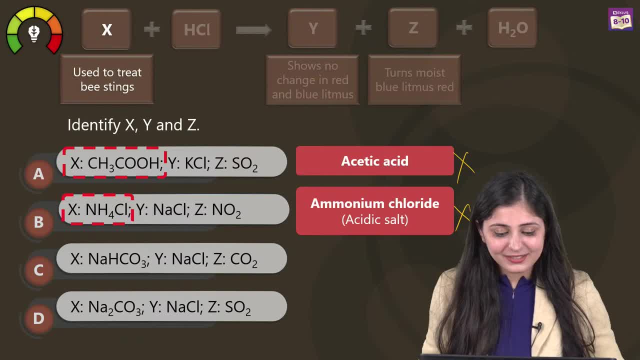 So Chitra says I love chemistry. Even I love chemistry. Hari Priya says C. Alright. 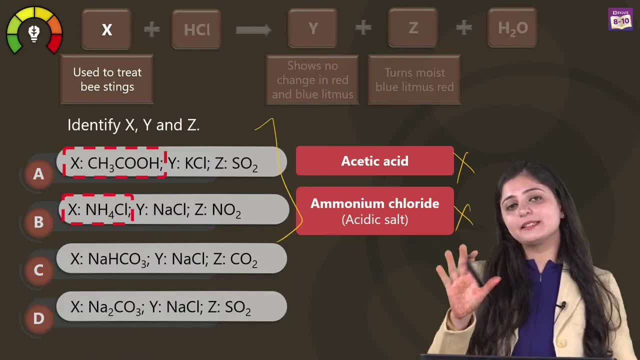 So the options wherein you see some acetic substance or the acid itself. Cross kar do. Wo toh bilkul answer sahi nahi hai. 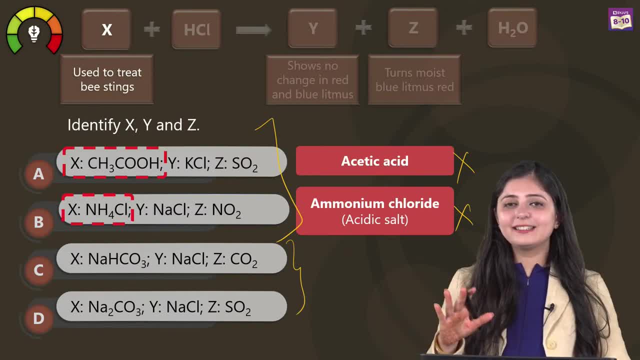 Ab in dono options ko dekho. And chemistry ko side rakho common sense se hi answer kar do. 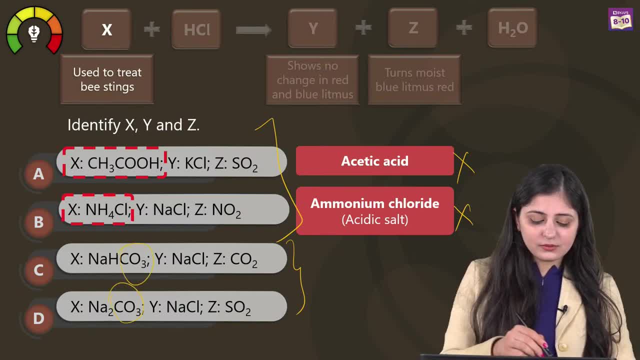 If you have a carbonate over you. Usse kaunsi gas niklegi yaar? Which gas do you think will be released? 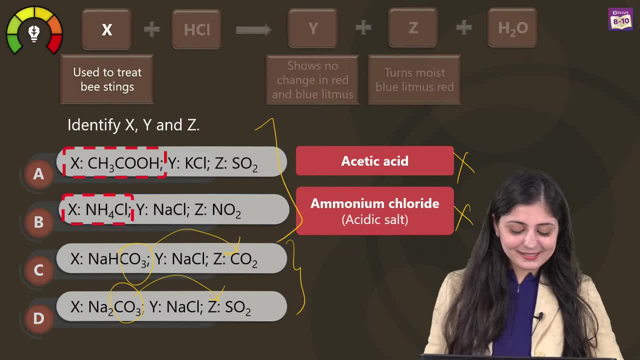 It is going to be carbon dioxide. Sulphur dioxide toh nahi hoga. Toh agar chemistry point of view se confused bhi hor rahe ho na. Be very attentive. Be very alert. 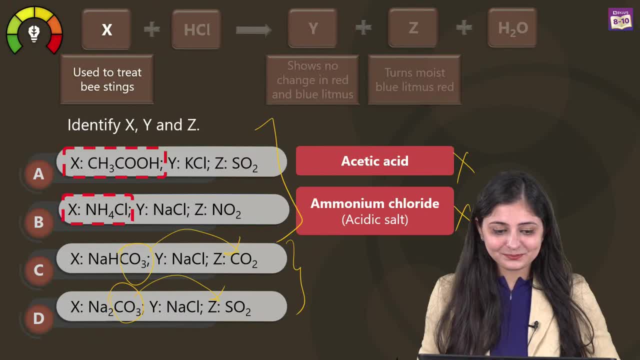 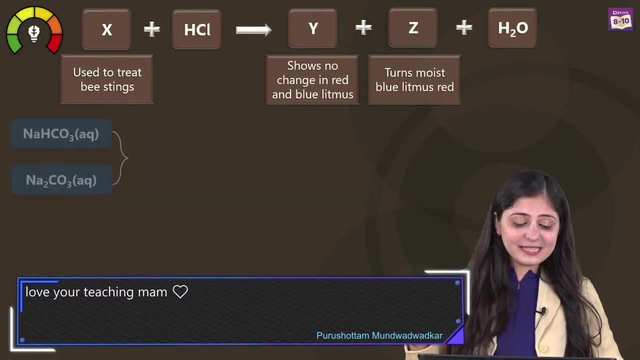 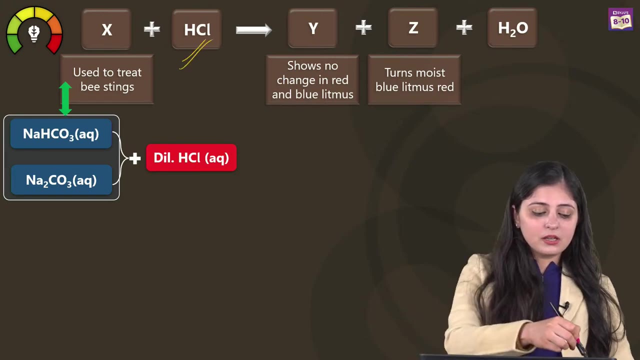 Common sense lagao you will reach at the correct answer. Alright. Now. A and B humne eliminate kar diya. Ab C or D ki jab hum baat karte hai. Dono ko jab hum HCL se treat kar aenge. Because they are saying HCL se treat kar aao. Only metal we have is sodium over here. Isn't it? 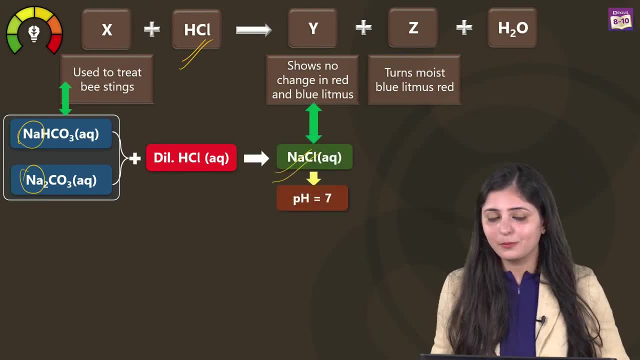 Sodium chloride will be the salt that is going to form. And we all know that. It's a neutral salt. So pH is going to be 7. And that's the reason it's not showing any change. With the red or blue litmus paper. Carbonate hai aapke paas. So carbon dioxide gas is being released. 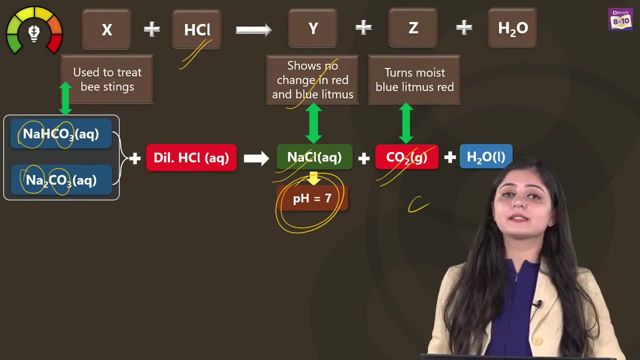 Now we know that carbon is a non-metal. And non-metallic oxides are acidic in nature. 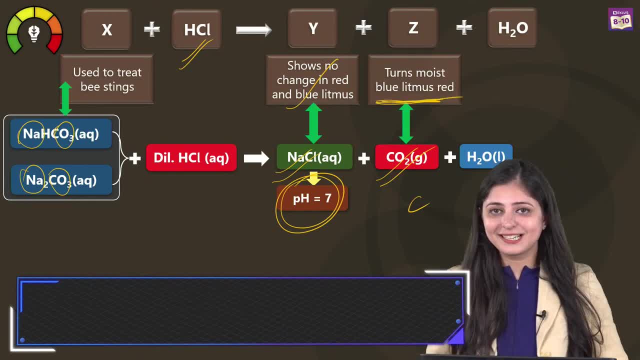 Agar wo acidic hai. Toh wo blue litmus ko kya karenge? It will turn it to red colour. 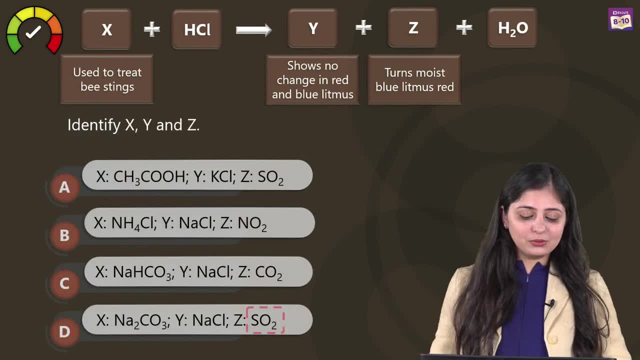 Plus water. So there you go. 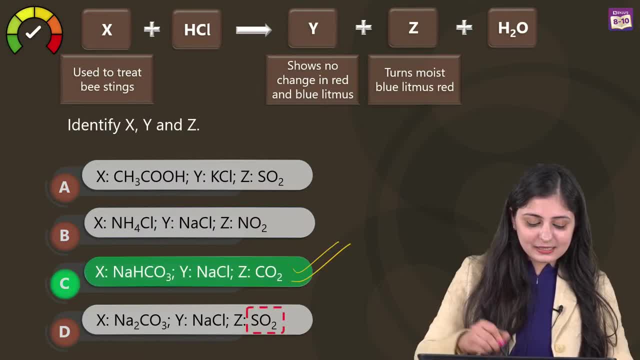 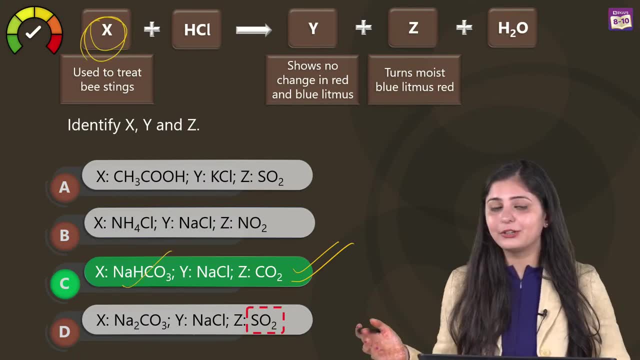 Your correct answer is option C. Your X that is being used to treat bee sting is sodium hydrogen carbonate or sodium bicarbonate or baking soda. 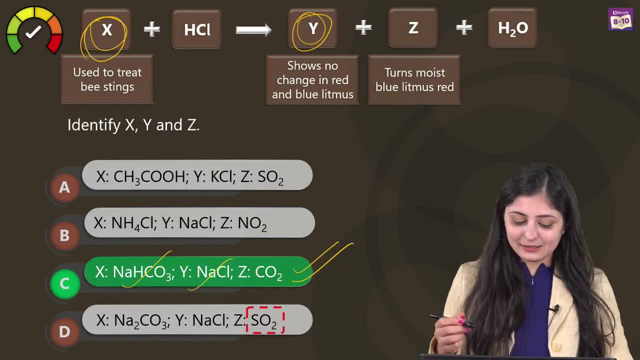 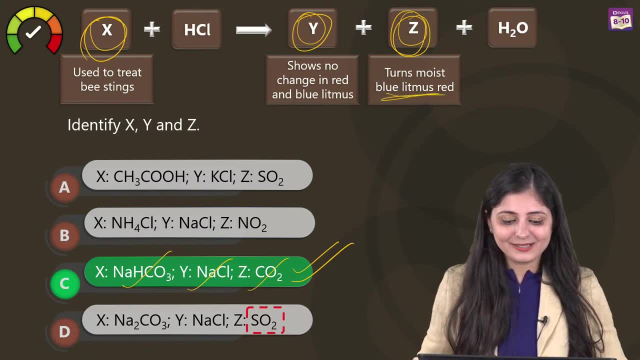 Y which is neutral is your NaCl. And Z which is turning blue litmus to red is your carbon dioxide. Shailja says interesting. 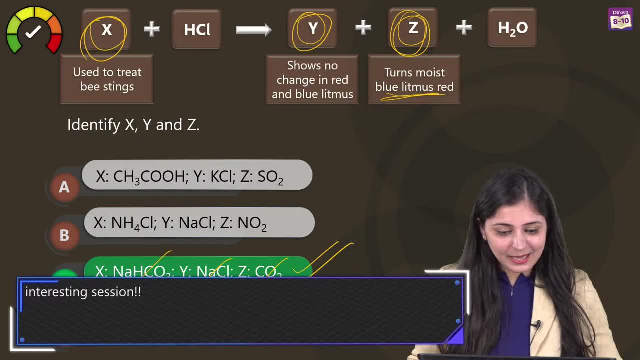 Paas said C. Samvir said C. Shubham said C. 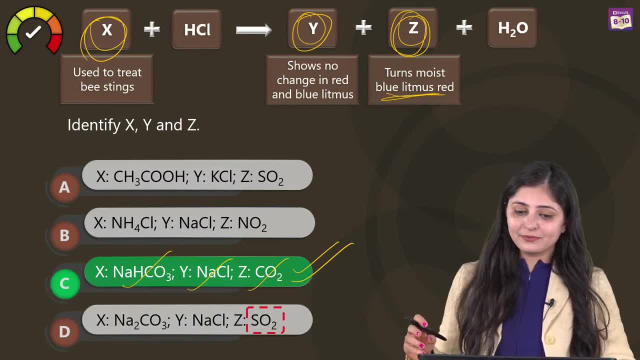 It's great that for this particular question. 95% of you were on the same page. And you had the right answer as C. 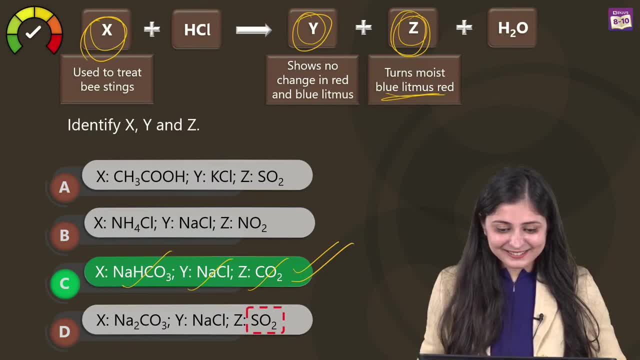 Great. Alright with this we've come to the end of today's live session. On pH and its importance in daily life. I hope this session was useful. 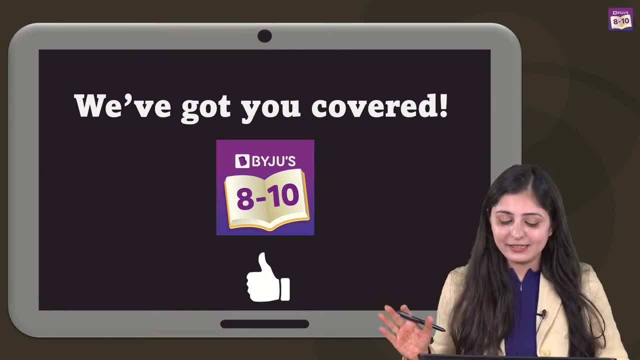 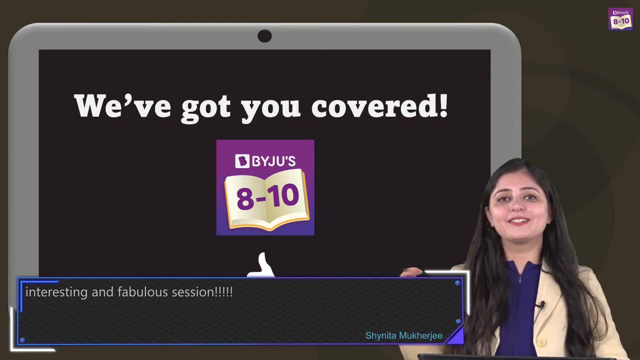 It was interesting. And it was easy. Because personally I feel ye jo topic hai na ye bohot hi zyada scoring topic hai. Isko bohot achche se karke jao. Ye questions will definitely take your percentage up. 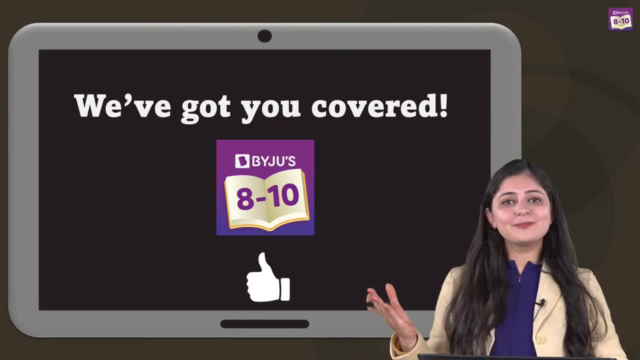 Now ye session toh khatam ho gaya. But we've got so many sessions for you people lined up. From every Monday to Friday. And these sessions are going to make you exam ready. They'll help you to ace the examination. So do not miss any session. You have to attend all of them. 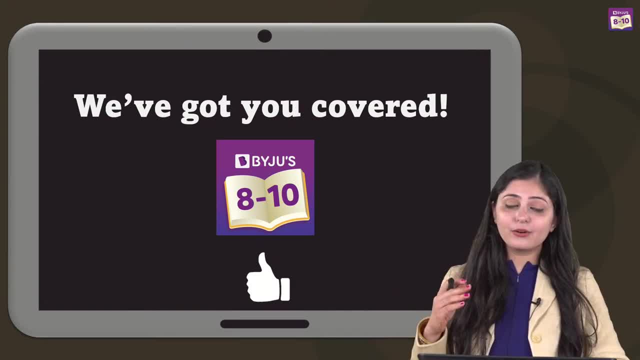 Bohot achche practice questions hai un mein. Aapka confidence us particular topic pe us particular subject me definitely increase karega. So we've got you covered guys. 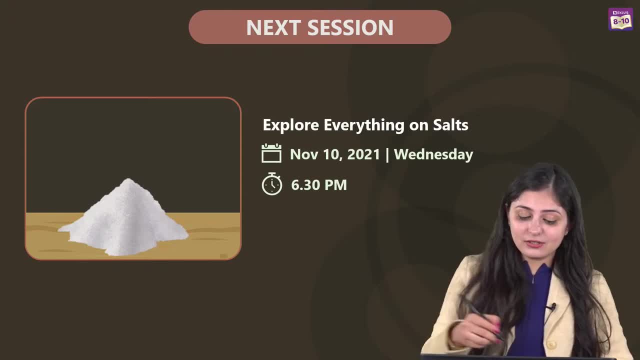 Now coming to chemistry. We've got the next session. That is on November 10. It's a Wednesday. One week from now. But guys look at the time. It's going to be at 6.30 pm. The next time. That's why subscribe to the channel. Hit the bell icon.